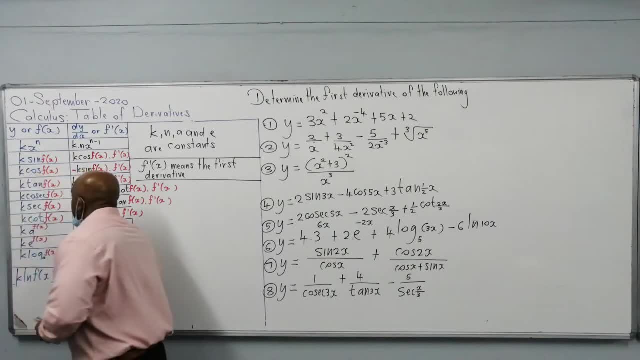 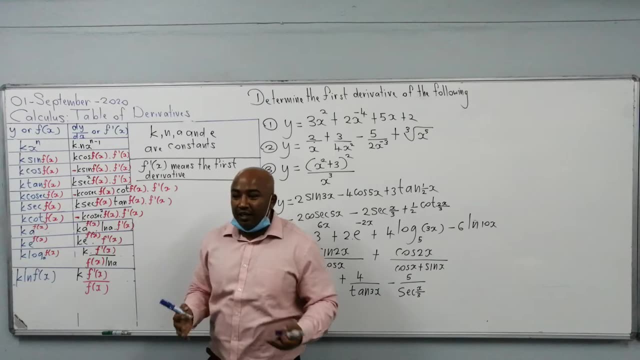 However, now you see the table of derivatives. There's not only kx to the power m. You must be able to differentiate anything here, Any graph here that you are able to sketch. you must be able to find the first derivative of: Okay, So here you can see, I've got one. 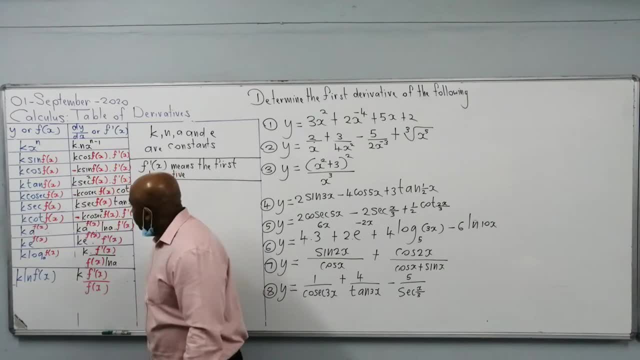 two, three. there's quite a few here. So now this is your table of derivatives. In the first column. here I have all the original functions. This is basically the questions And next to it is the answer, Basically the solution on how to differentiate it Right? so if we go to 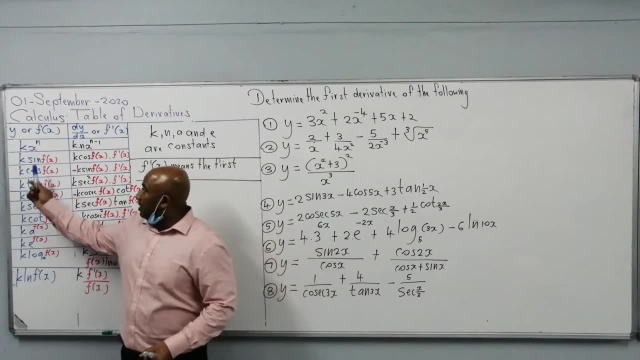 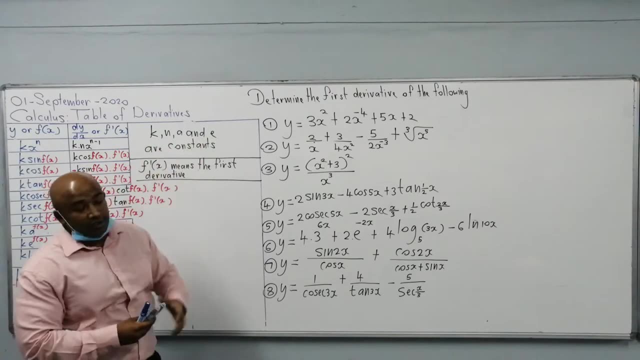 number 1, which we have been doing previously. this is a number like 2x squared, So k and m. So I wrote down here all k, m, a and e, Whenever you see that in the table of derivatives. 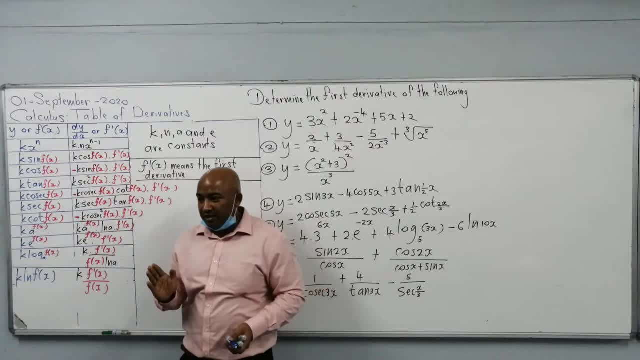 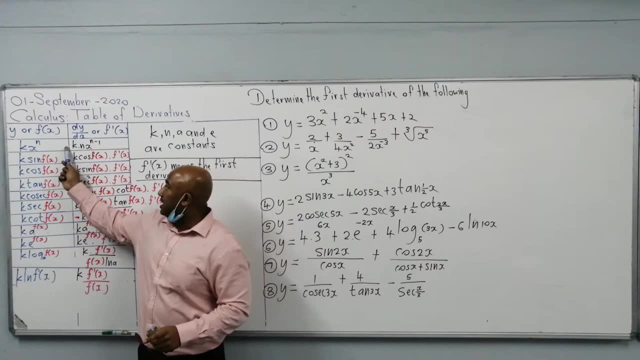 they represent constants, They don't need to be multiplied. So you can see that the numbers don't change. They are just a number. So here, remember, when you differentiate kx to the power m, then the first derivative is k multiplied by nx to the power n minus. 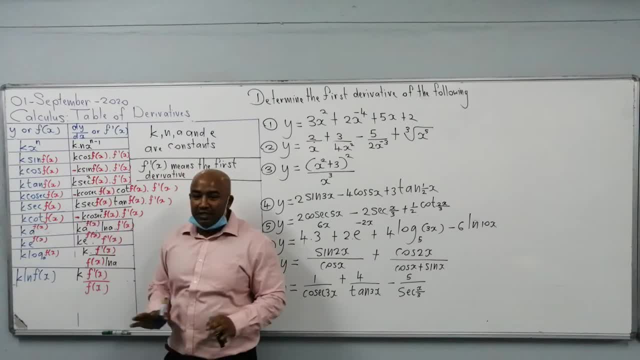 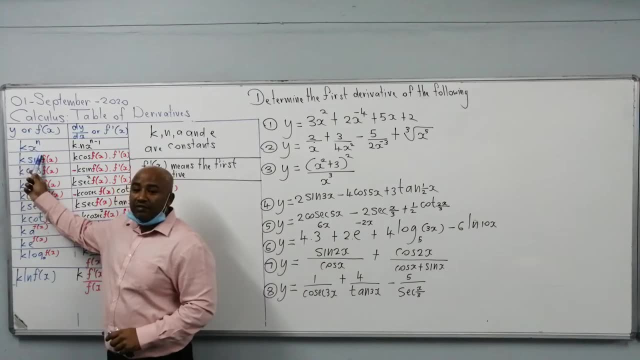 1. Right, so this is applying the rules straight from your table. This is not first principles, Right? so now you come across new things like the derivative of sine cos, tan, cosec, sec, cos. Then you've got your two exponential graphs here. 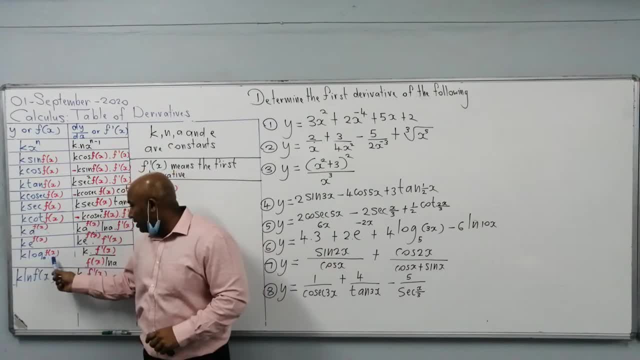 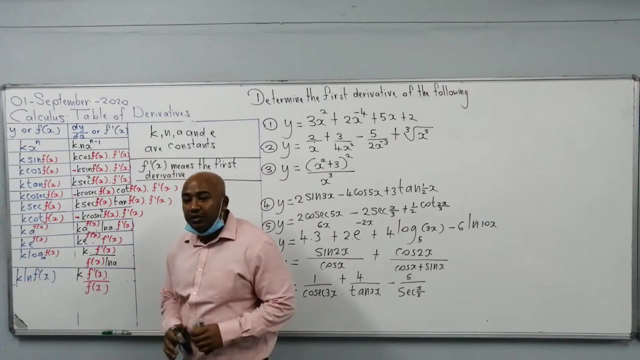 Then you have your two log graphs. This is k log f of x to the base a, and this is k l n, that's lin or natural log F of x. your base is not shown. I'm going to explain that to you in a few minutes. So now what you need to do is the best thing if you're moving. 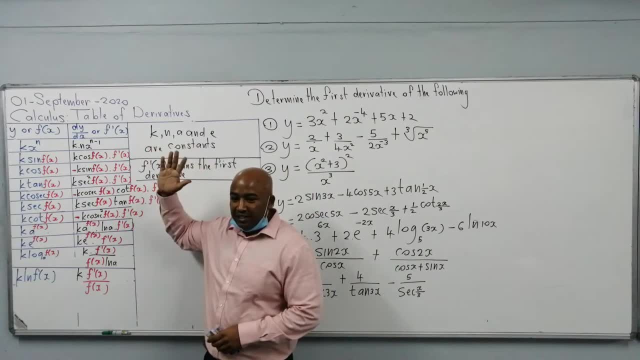 up in engineering, you're getting on to n5 and n6, you will be dealing with this. Basically, it will be the whole syllabus, So it's best to memorize this table here. Okay, because there's much more. there's many. 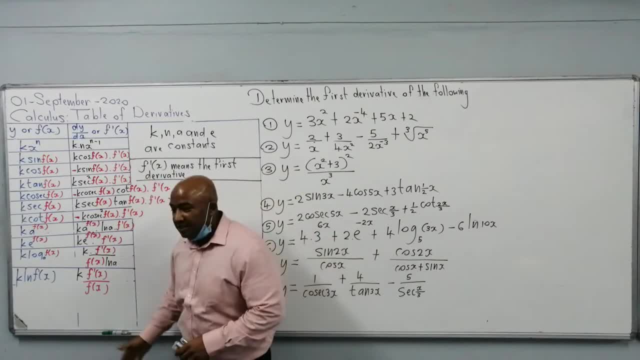 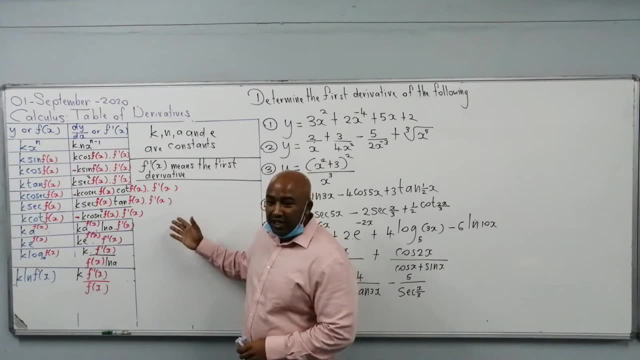 more rules that you're going to learn, but you will always be using this table of derivatives And if you have it in your head then it will be easier. Remember: differentiation is 20% and integration is another 20%, So that's calculus is 40% in your exam. So to make sure, 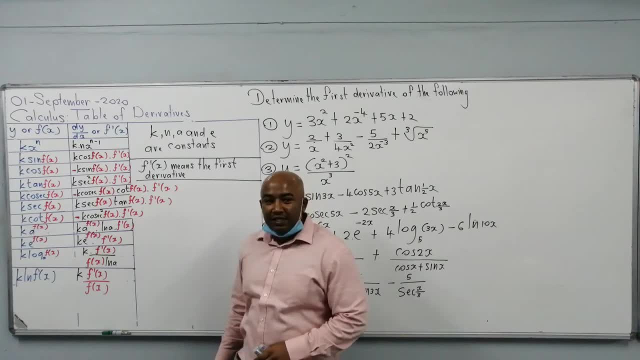 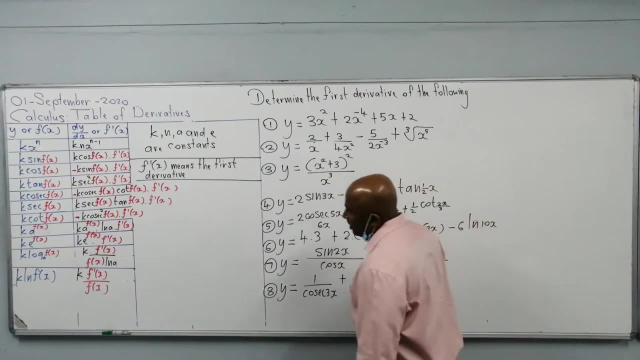 it's 40%. at least memorize this table. You write it down over and over again until you know it. So we're not going to get into first principles, We're going straight to the table. You have been dealing with first principles in grade 12 and n3.. So let's recap, Let's do a few. 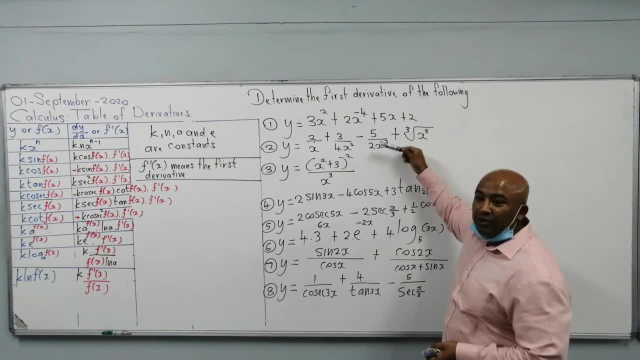 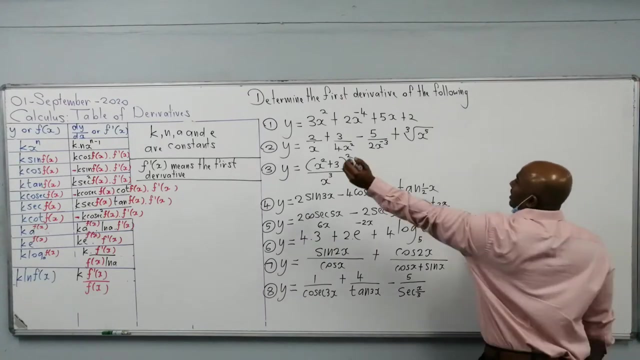 examples. This is revision of n3 work or grade 12.. All right, so the question is: determine the first principle, The first derivative? So here I'm giving you everything. This is an equation of y in terms of x. So let's deal with number one. So here for number one. first of all, if you want, 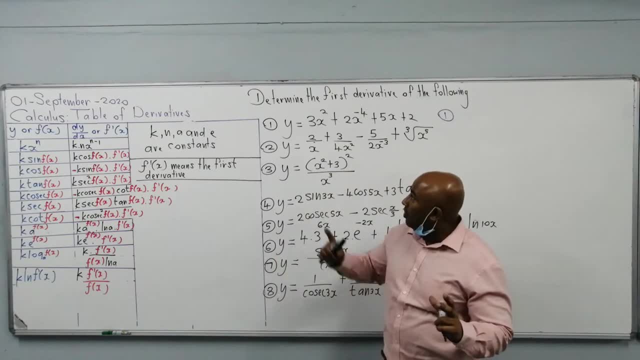 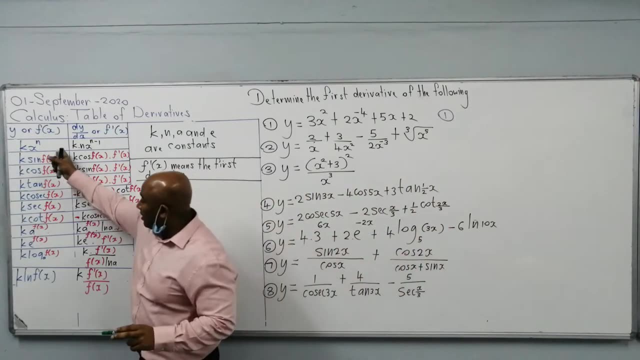 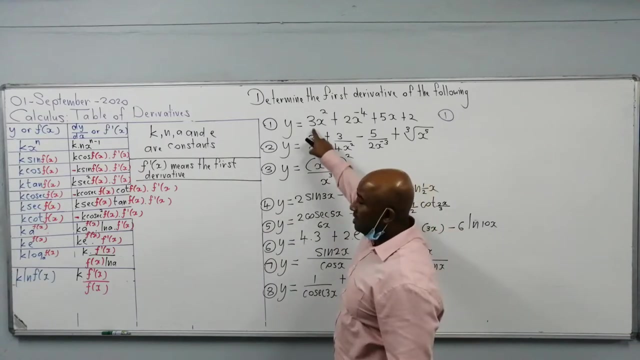 to differentiate, make sure that all terms are in standard form. Standard form means it must look like something on the left-hand side of this. So let's look at term one. Term one is in standard form. Here's your kx to the power. 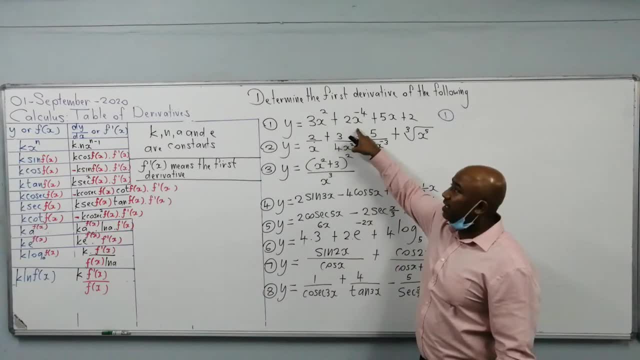 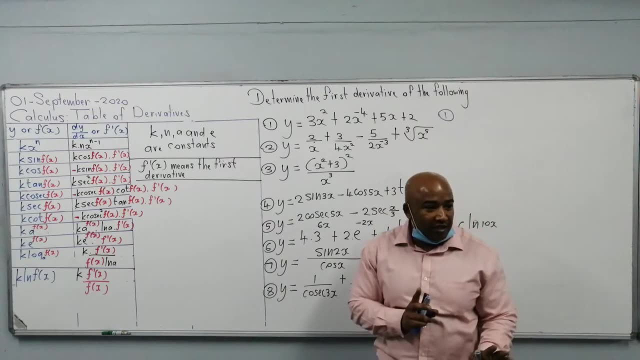 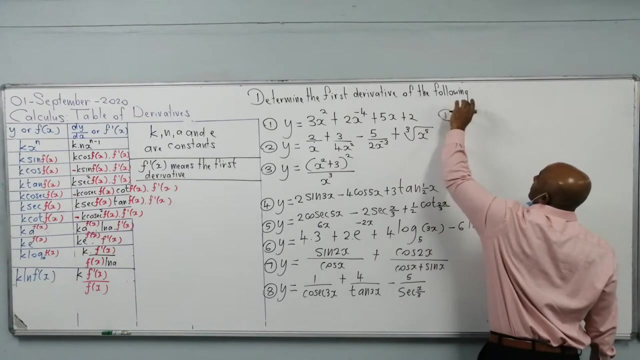 n, Term two, also in standard form, kx to the power n. Term three, term four. So they're all in standard form. I do not need to manipulate anything there. I can differentiate it straight away. So when I differentiate I'm going dy. 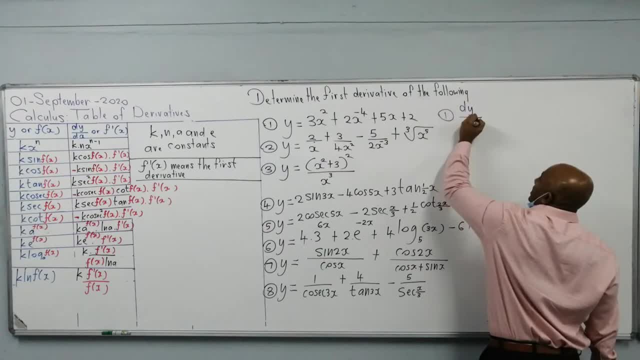 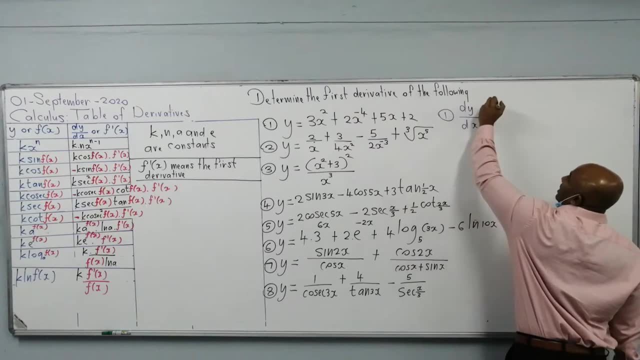 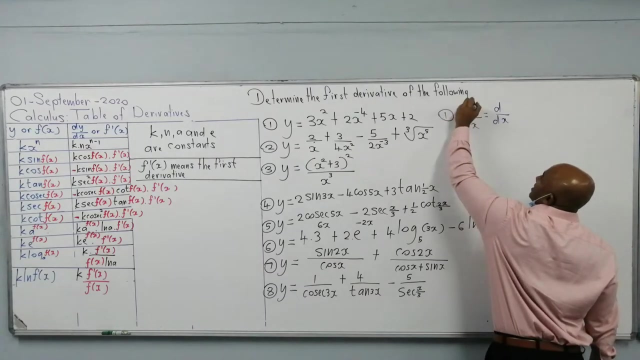 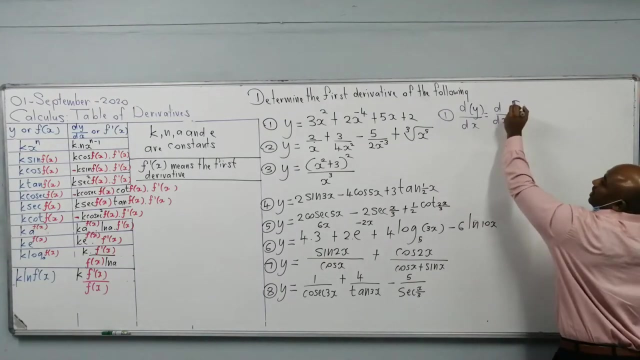 So basically, what's happening here is you are finding d over dx of both sides. Let me just rewrite this: So that's d over dx of y, So that's the left-hand side. Whatever you do on the left-hand side, you do on the right-hand side d over dx of 3x squared plus. 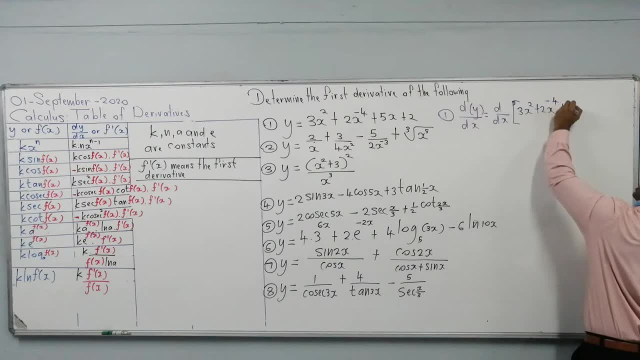 2x to the power minus 3x. So that's the left-hand side. So that's the right-hand side. That's 4 plus 5x plus 2.. So what does this mean? d over dx. I'm differentiating y with respect. 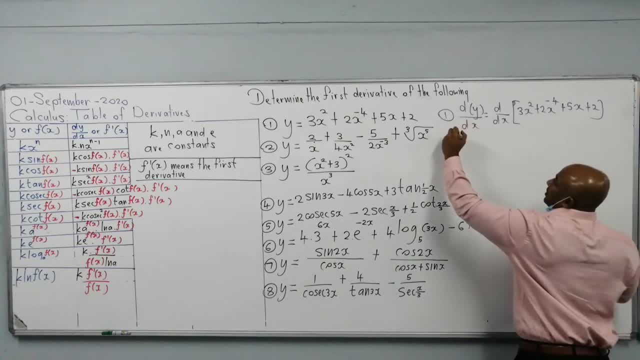 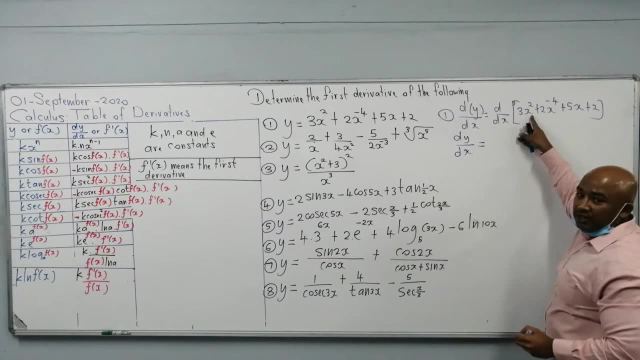 to x. So now I have dy over dx. So now d over dx of 3x squared, The derivative of 3x squared. So what do we do here? Here's: we multiply the coefficient by the exponent, So that's going to be 3 times 2.. Write down your base, which is x, and take your exponent. 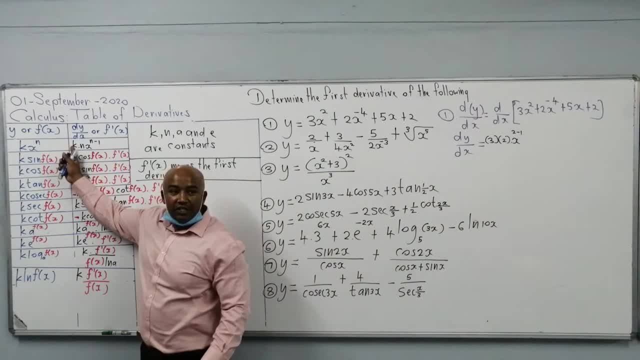 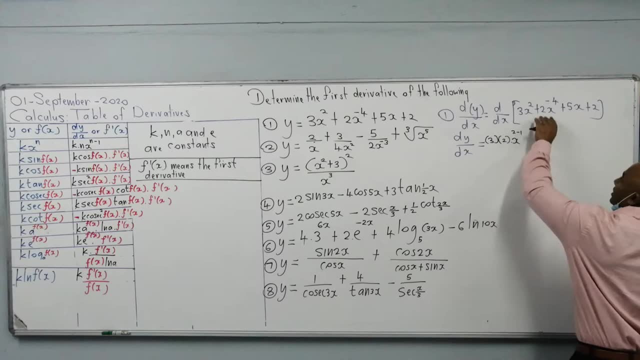 and subtract 1.. So there is the rule here: Multiply the coefficient by the power, Take the same power, Subtract 1.. You know you've been dealing with this from grade 2 up, So here this is going to be a plus 2 times minus 4.. And then you write down the base which: 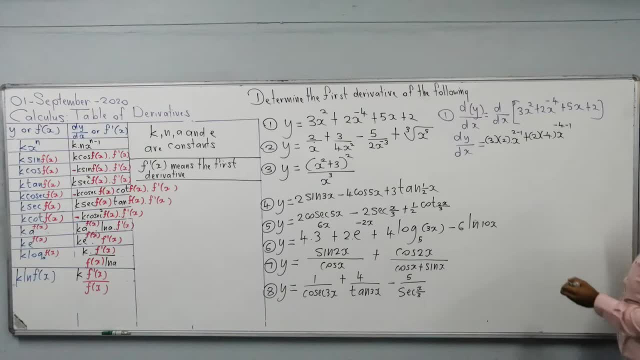 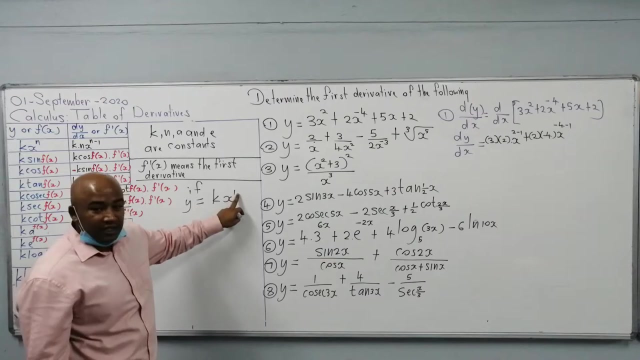 is x, And then minus 4, minus 1.. Yeah, The derivative of 5x. So there is a shortcut that you can use here. So basically, if y is equal to kx to the power 1,, if y is equal to kx to the power 1, so here, clearly, my exponent. 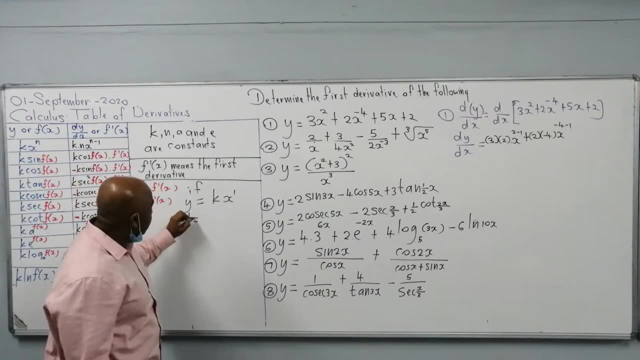 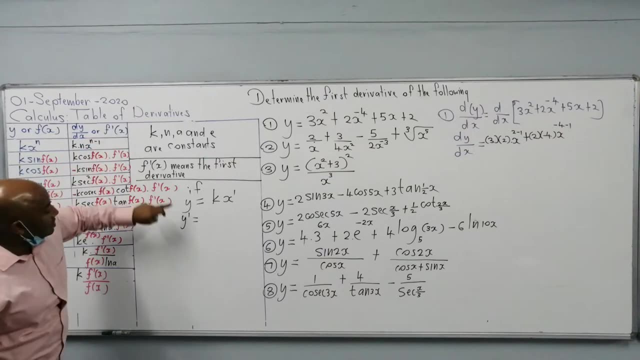 is a positive 1, then the derivative here. so I can write it as y prime. It means the same thing. So I can write it as dy over dx, F prime x. Oh, I can write it as y prime. It means they all mean the same thing. So 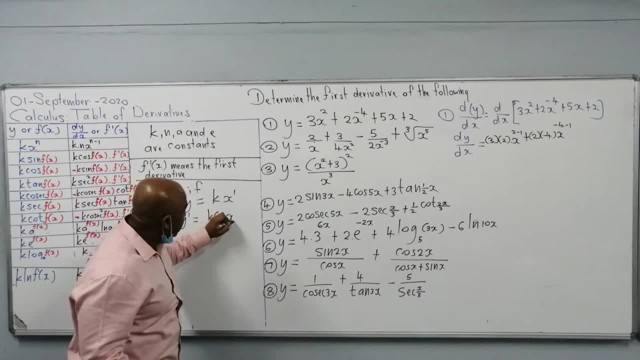 I will multiply. This will be k times 1, x to the power, 1 minus 1.. Can you see that? So therefore, k times 1 is k x. 1 minus 1 is 0. So I've got k times x to the power. 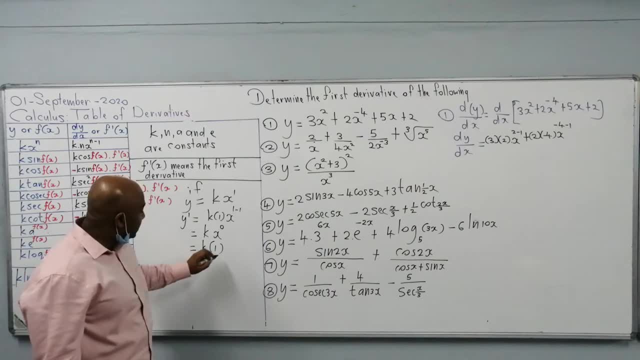 0.. What is x to the power 0?? It's 1.. So k times 1 is k. So basically the result: it will always be k if your exponent is a positive 1.. So what does that mean? It means: 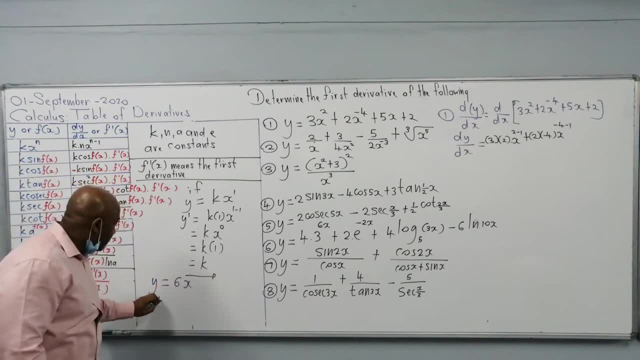 that if I've got y is equal to 6x, I do not have to go and do it the long way. I know that k is 6. here Can you see that If your exponent is a positive 1, the derivative here. 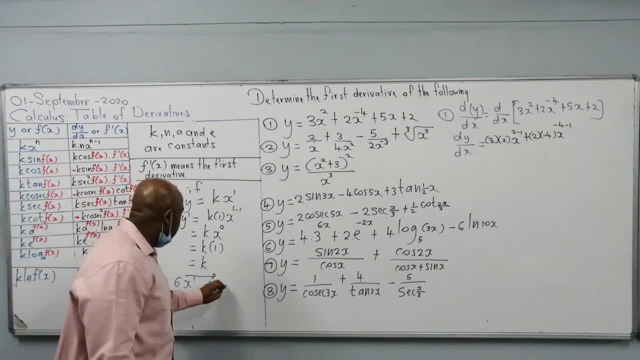 will just be 6.. So then, if I have, y is equal to minus 13x. if I want to find the first derivative, I'm going to have to do it the long way, So I'm going to have to do it. the 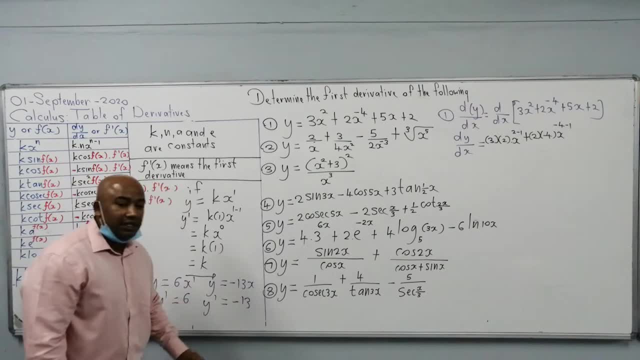 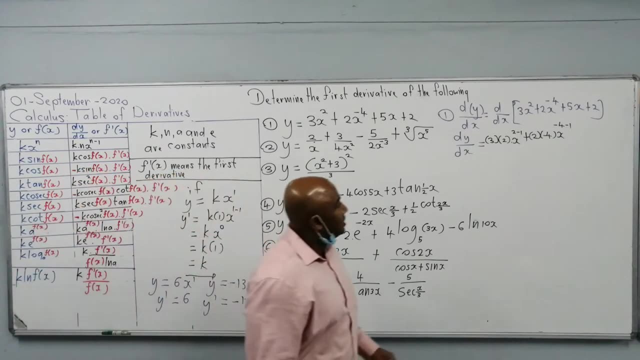 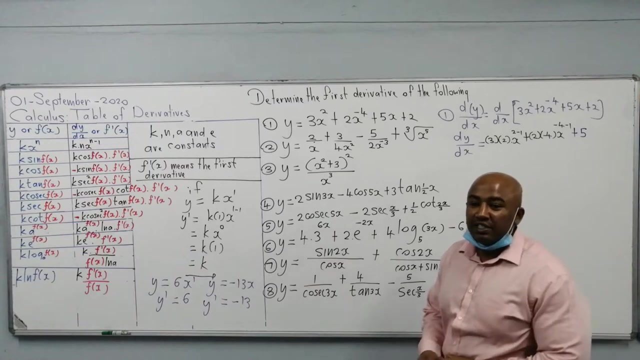 long way. So the derivative of minus 13x is going to be minus 13.. So it only works if your exponent is a positive 1. That's a shortcut. So in this case, here the derivative of 5x will be 5.. Now what about the derivative of a constant? The derivative of a constant. 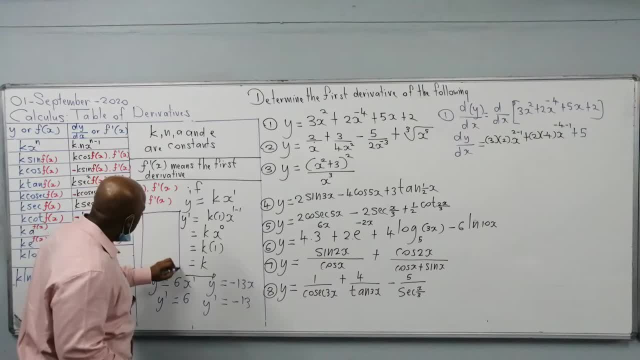 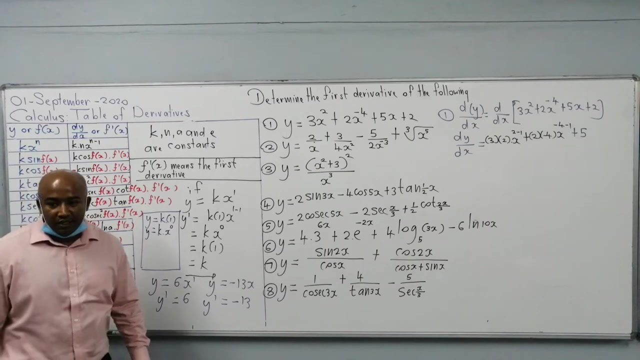 let's write it down here: y is equal to k. k is a number, a constant. So now, if I multiply it by 1, am I changing the question in any way? No one rocks. 1 is actually x to the power, 0.. x to the power. 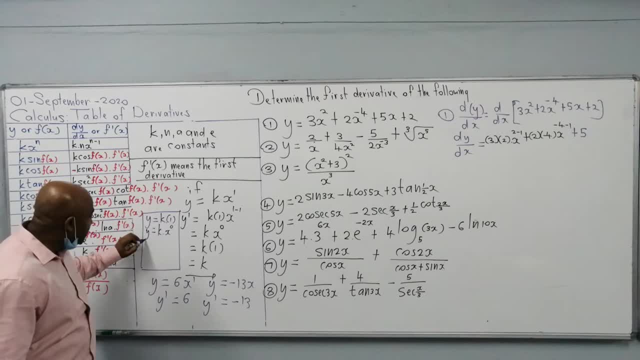 0 is 1.. So now, if I differentiate here, I'm going to go k times 0, x to the power 0. So I'm going to go k times 0 minus 1.. Can you see that? So therefore y prime is equal. 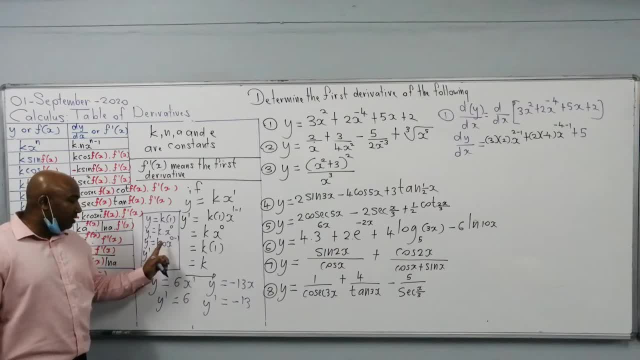 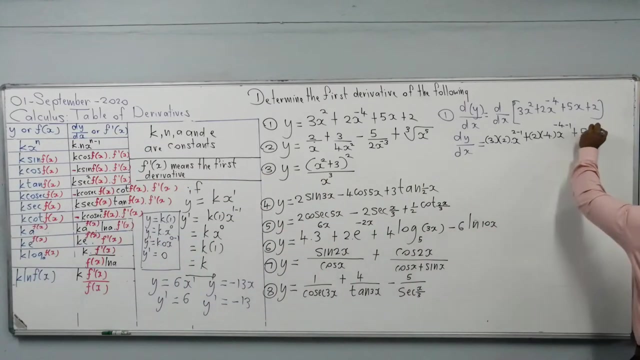 to the fact: here is 0 minus 1, is minus 1.. But this 0 is being multiplied by all the bases here, So it doesn't matter what the exponent here is: 0 times anything will be 0. So therefore, shortcuts, the derivative of a constant is 0.. Now you do not have to. 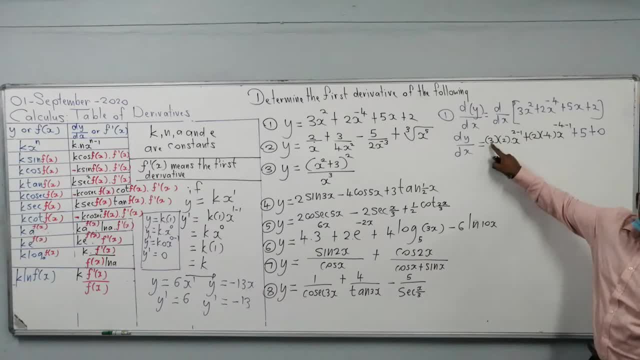 go and write down 2 minus 1. You do not have to go and write down 3 times. 2. You can go one time to the step here and write down the solution, because it's taken that you know that the rule 3 times. 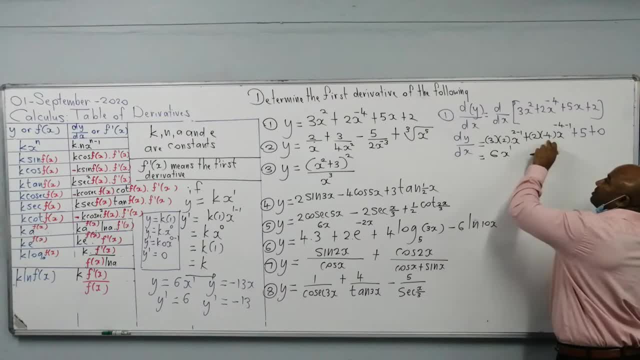 2, that will be 6x to the power 1.. 2 times minus 4 is minus 8x. Minus 4 minus 1 is minus 5.. And then we've got our plus 5 there, And I will advise you to copy down that 0 given. 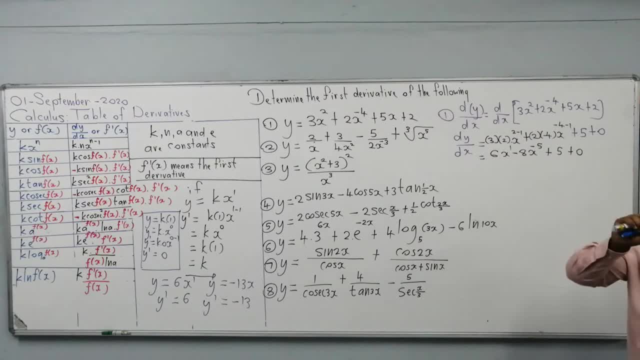 in your final answer, because whoever is marking your answer is going to be the one who is giving you the answer. So what is that 0?? That is, what is that 0?? That is the derivative of a constant. so this derivative of 1 will be equal. the same norm goes up by this here. 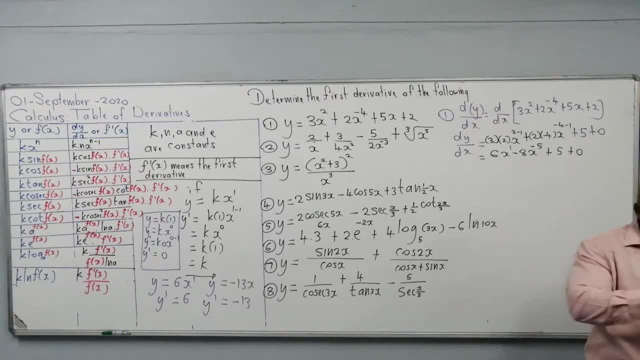 And this is going to be a diagonal here because we've sting to leave it to the where, anyhow, because we are going to מה�� Informations class. but this: A equals B, obviously. What is that? simple one That A equals Bcker, 차ız, and that might be C. So what is that? 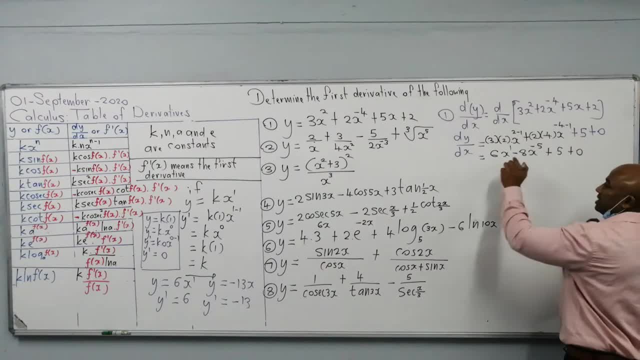 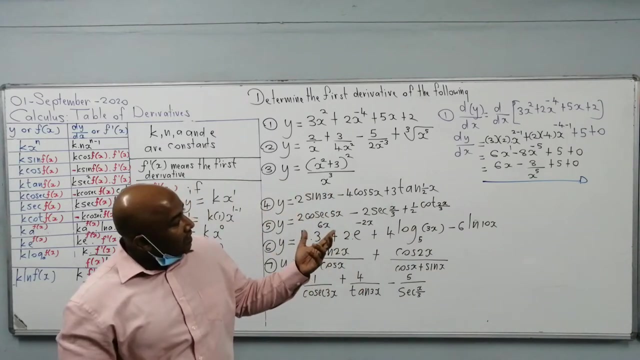 C. So that is the derivative of a constant created. See, we can just take it one more time- and that is the derivative of a constant. So when we put it together, as you can see, fortress k times 2 make that 0, that's 0 plus 1.. We can simply put two next time In this example. 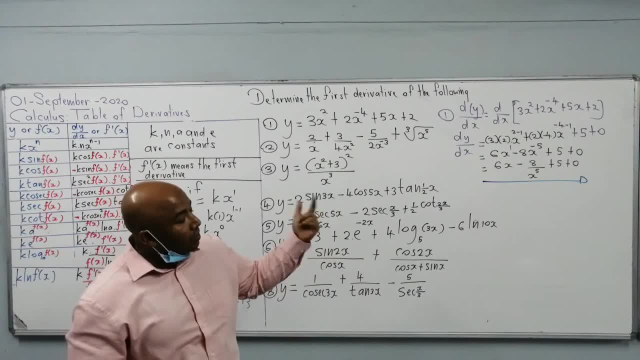 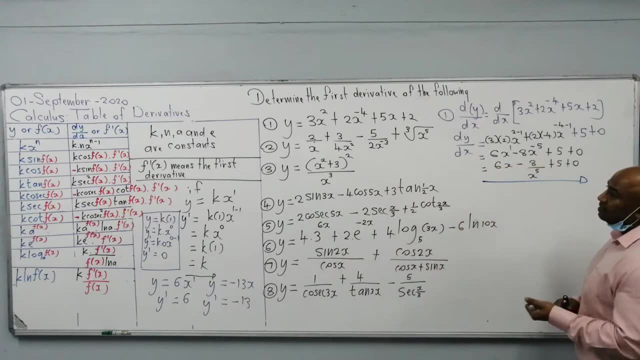 rewriting my terms of positive exponents, but you will only do that if it is required. So that is the first one. Let's deal with the second one. So I've got y is equal to 2 over x plus 3 over 4x, squared minus 5 over 2x to the power, minus 3 plus the cube root. 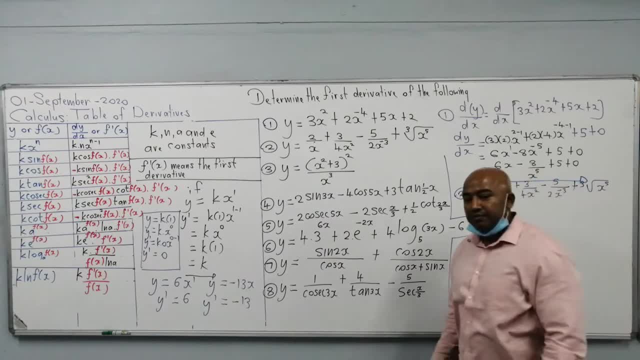 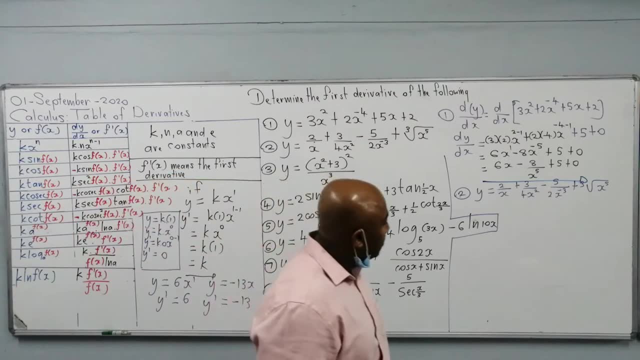 of x to the power 5.. Right, so now still dealing with some great 12 revision here, or m3 revision. we have many terms: 1,, 2,, 3,, 4 terms, So let's deal with the second one. So let's deal with the third one. So let's deal with. 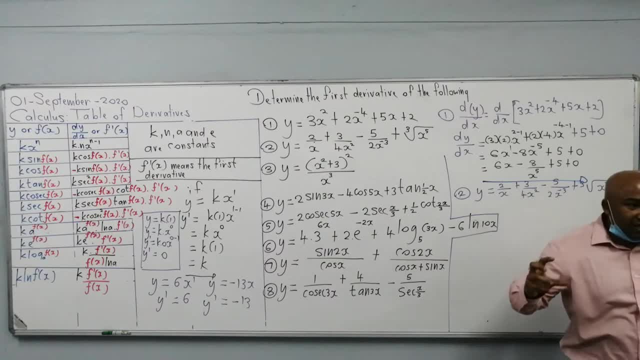 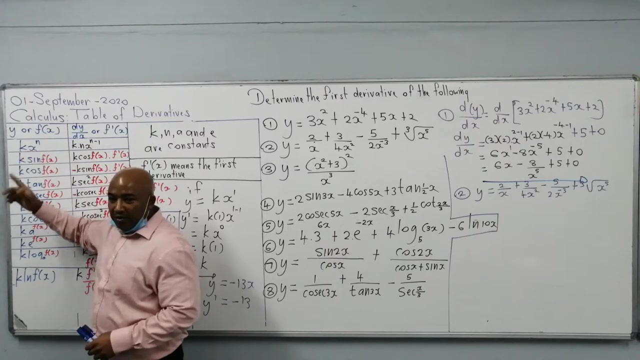 the fourth one. So let's deal with the fifth one. So let's deal with the sixth one. So now, if we need to differentiate, we need to make sure that all terms are in standard form. That means they need to be looking like number 1 here, which is kx to the power n. 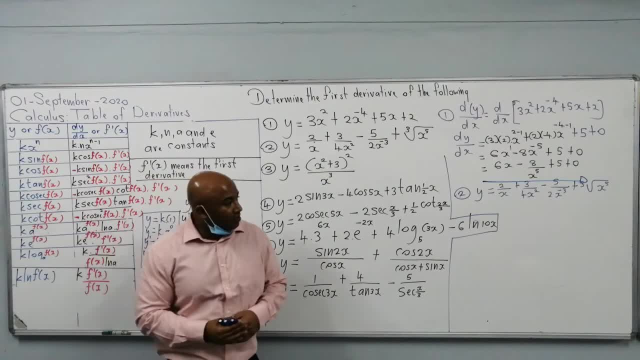 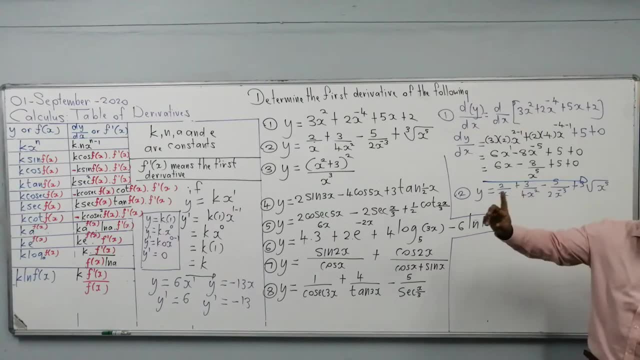 At the moment we are still dealing with only number 1 here. Right, just for to recap. So here, this is not in standard form. Your standard form is k multiple. So here this is k multiplied by x. Now you have a number divided by x. Okay, So 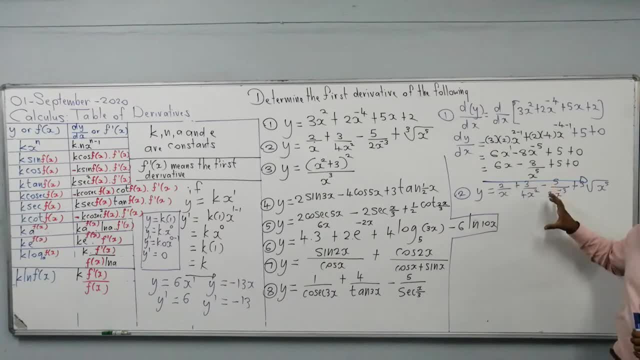 at this point, I did not show you the quotient rule, So we are not using the quotient rule yet. We are still going to learn the quotient rule in a few minutes, where you can apply a rule for differentiation regarding division and then product rule for multiplication. 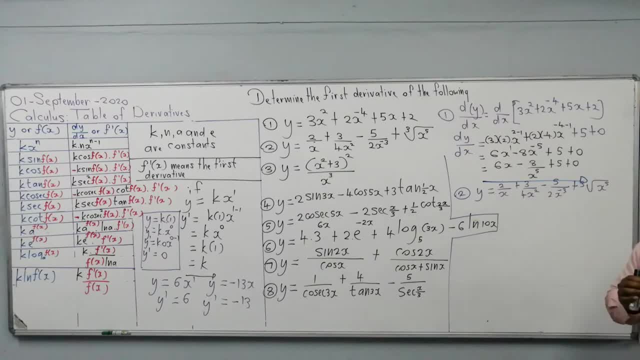 For now we have to rearrange using our exponents. So y is equal to: I got 2 over x. So remember what's the power here. If it's not shown, it's a positive one. So if I take x to the top, if I take x to the top, the sign of the exponent will: 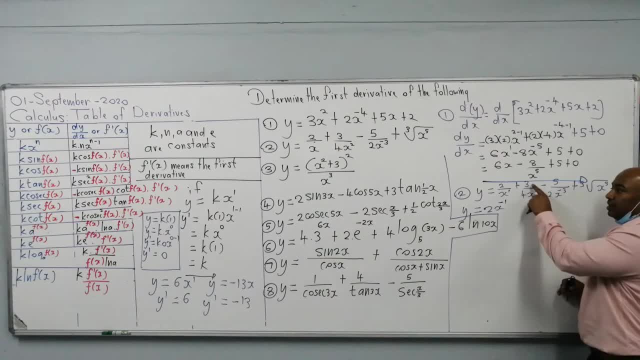 change That will become a negative. Right Here I got 3 over 4x squared, So be careful- This is a common mistake that students make. You do not take 4 to the top, because 4 is multiplied by x squared, So 3 over 4x squared. what does it mean? 3 over 4x squared? let 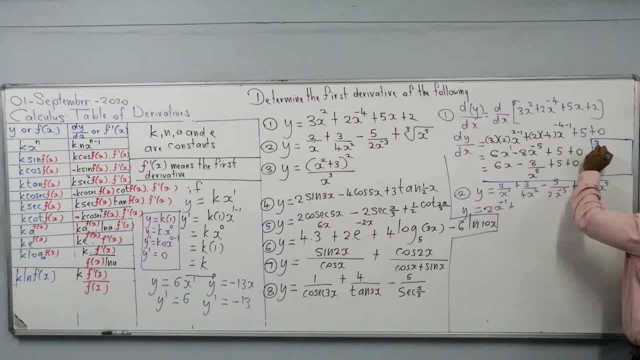 me just write it down here. So if I've got 3 over 4x squared, this means it's 3 over 4.. Sorry, And it's 3 over 4 in the bottom x squared, this means it's 3 over 4 multiplied. 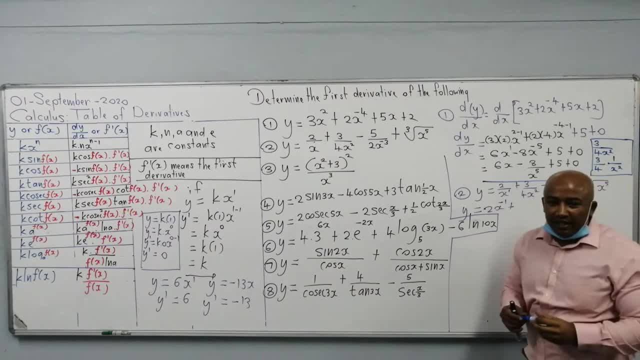 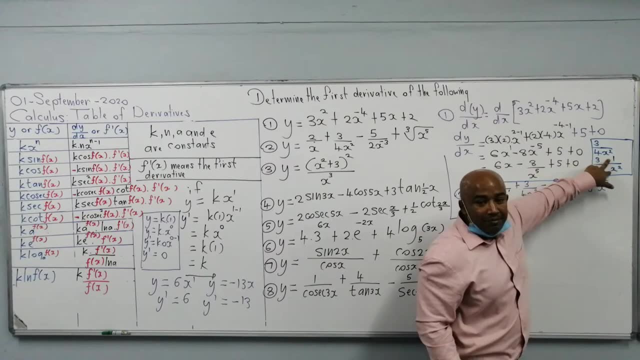 by 1 over x squared. You need to understand how to rewrite a fraction. So here's a fraction, 3 over 4, multiplied by 1 over x squared, which resulted in 3 on the top, because 3 times 1 is 3, and in the denominator, 4 times x squared is 4x squared. 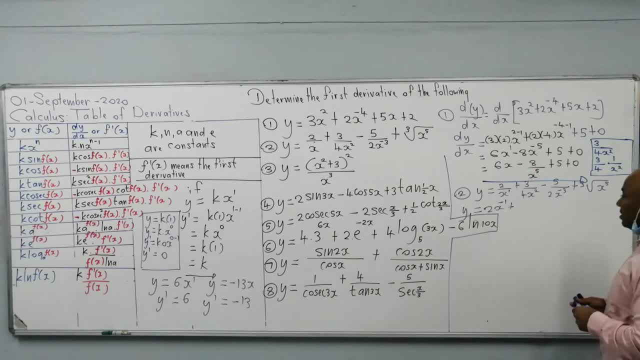 So all you're going to do is take x squared to the top. So in this situation here it's going to be 3 over 4 times x to the power negative 2.. When you take x squared to the top, the sign of the exponent will change. So if I take x squared to the top, the sign 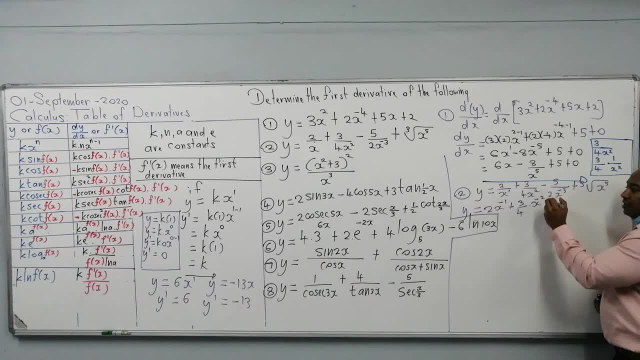 of the exponent will change. So if I take x squared to the top, the sign of the exponent changes. Here we've got minus 5 over 2.. I will take x to the power negative, 3 to the top. It will be times x to the power positive, 3.. I've got that Here. this here is the cube. 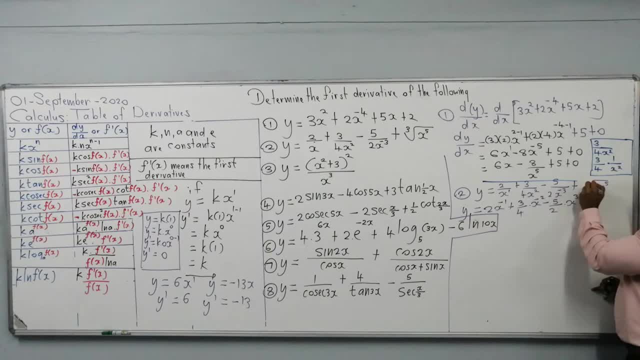 root. So here we have the cube root of x squared. So here we have the cube root of x squared. So here we have the cube root of x squared. So here we have the cube root of x to the power 5.. So I need to rewrite this in exponential form. So how do I do? 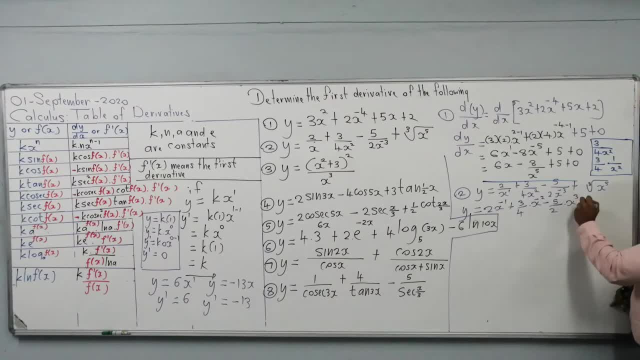 this. Remember that I will write my base, which is x, Now this 5 and 3, you will write it as an exponent, which is a fraction. What must you remember here Is that the root is outside. The root will always be outside. The root will always be outside, The root will. 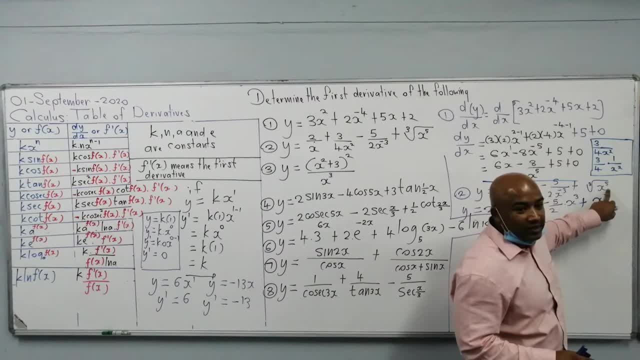 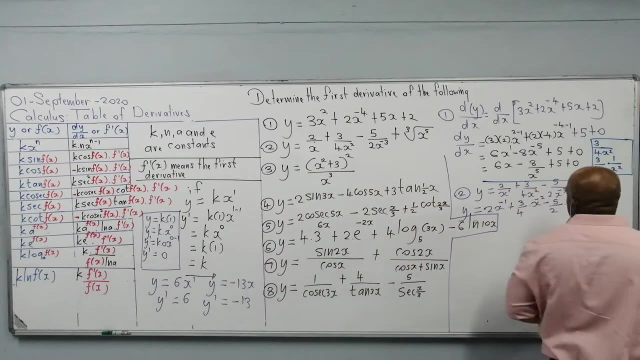 always be the denominator, So this exponent will always be the numerator when you convert it. So therefore this will be 3 in the bottom, 5 at the top, So it's x to the power, 5 over 3.. Can you see that Now all terms are in standard form, So remember standard form. 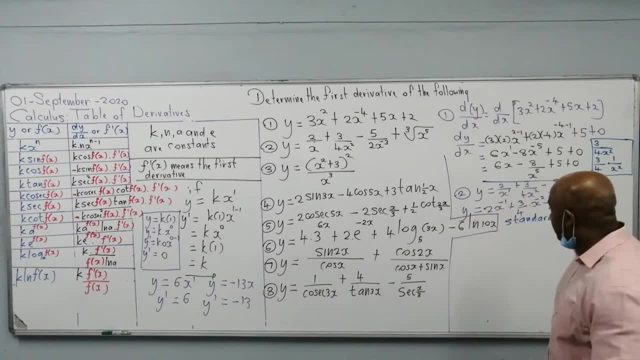 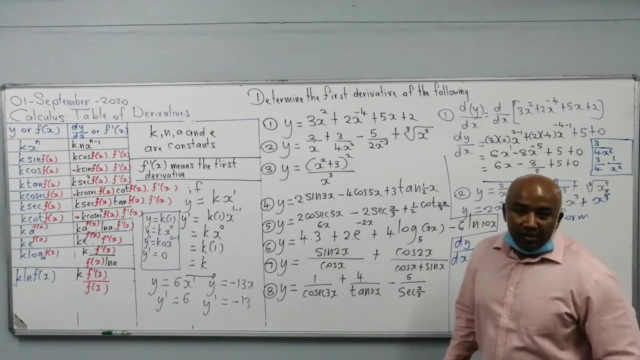 Standard form is k multiplied by x to the power n. Now I can find the first derivative there: dy over dx, So dy over dx. now This is all differentiation, straightforward. 2 times minus 1 will be minus 2x, Minus 1 minus 1. 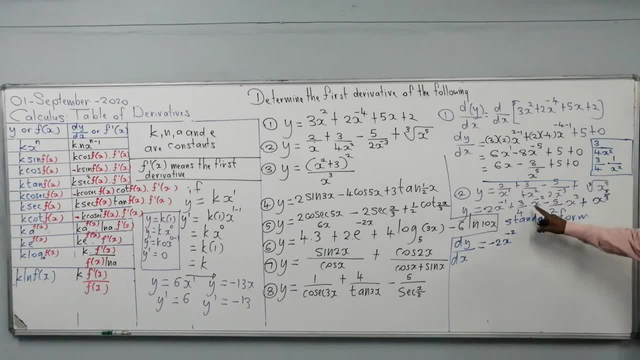 will be minus 2.. Here, 3 over 4 times minus 2 is a positive times a negative. That will be minus 6.. So 4x minus 2 minus 1 is minus 3.. Here we got a negative 5 over 2 times 3. That will. 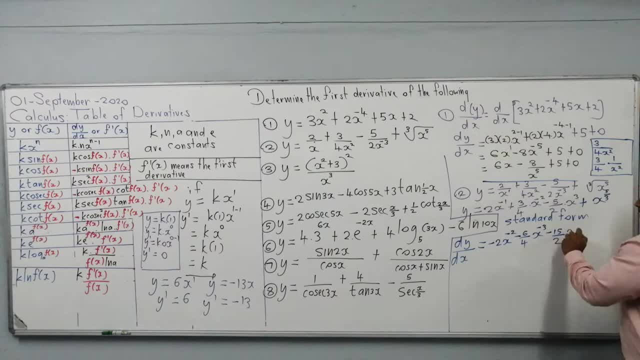 be minus 15 over 2x, and 3 minus 1 will give me 2.. Are you clear with that? Then the last one: here you got a 1 in front, So it's 1 times 5 over 3.. So 1 times 5 over 3 is minus. 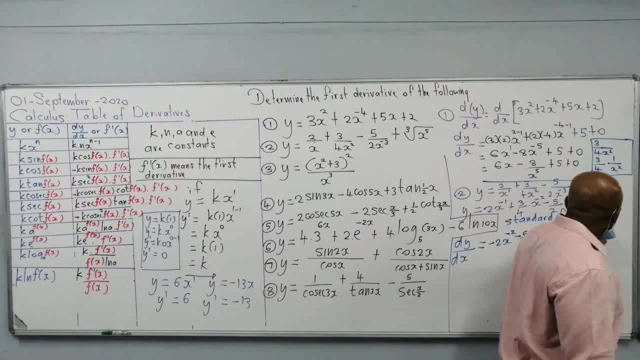 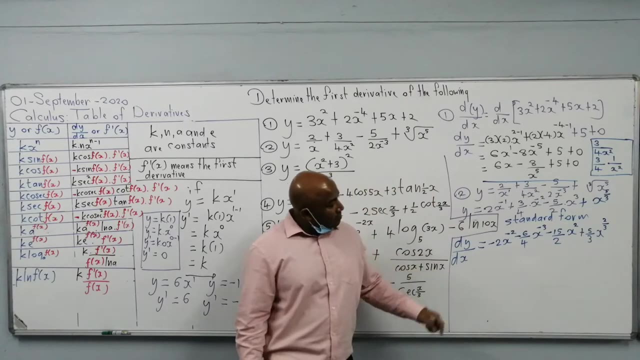 5 over 3x, Then 5 over 3 minus 1.. That means 5 over 3 minus 3 over 3, which is going to be 2 over 3.. All right, So this was, you can see, straightforward. Now I'm going to simplify my final answer. 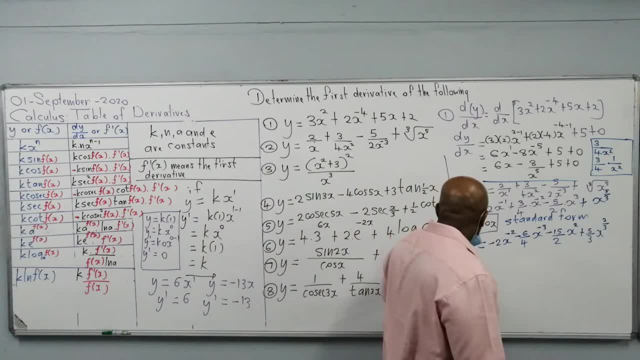 I'm going to rewrite it with a positive exponent. So my dy over dx- This is equal to that- will be minus 2 over x squared. So what did I do? I took the base to the bottom Sign of the exponent, changed And this is going to be 6 over 4.. 6 over 4. 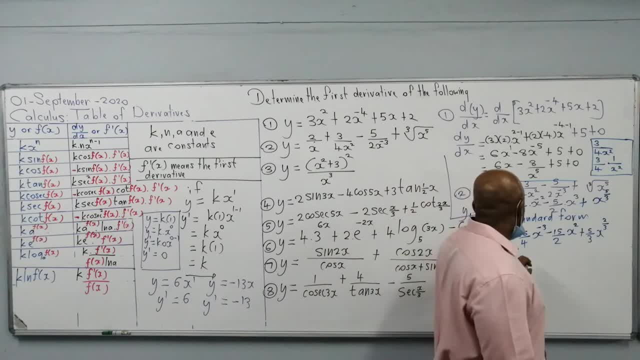 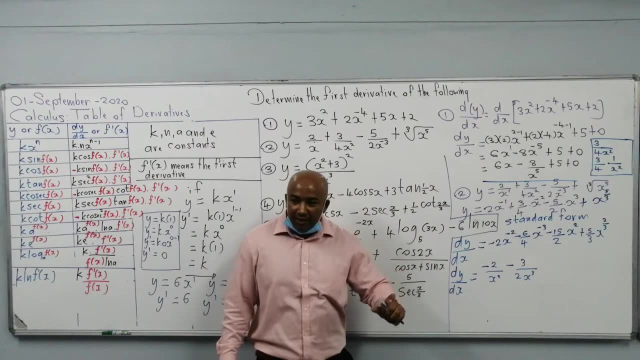 can be simplified further: 3 over 2.. So that's going to be my minus 3 over 2. x to the power 3.. Notice, I took the base x to the denominator and the sign of the exponent changed Here. 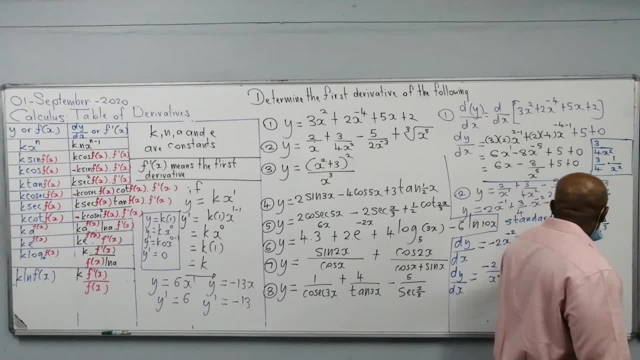 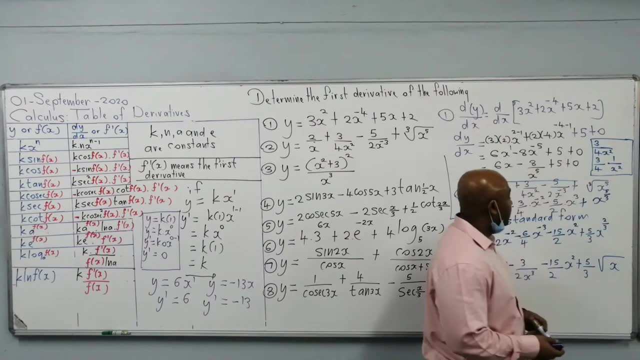 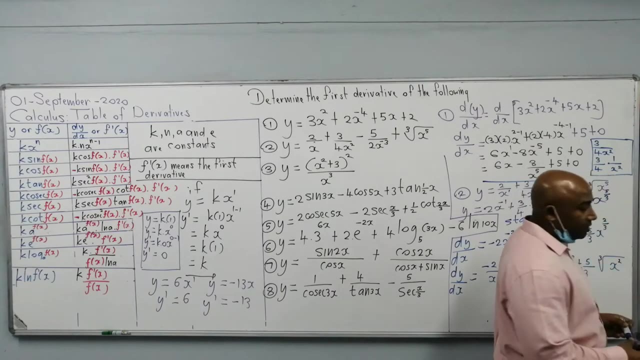 minus. there's nothing to do here. Minus 15 over 2 x squared Here. I'm going to rewrite it back in third form. I'm going to rewrite that back in third form. So this here is a 2 and this will be 3.. So that is simplifiers. All right, Have a look at that. Check the. 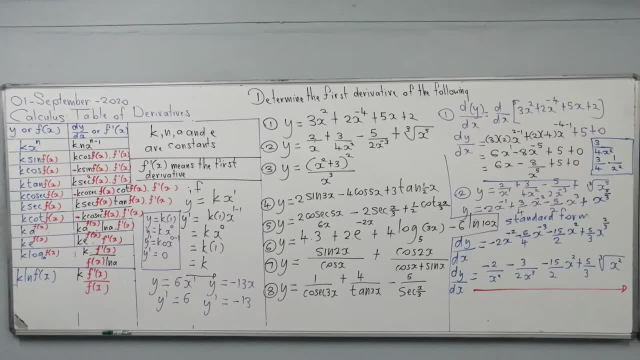 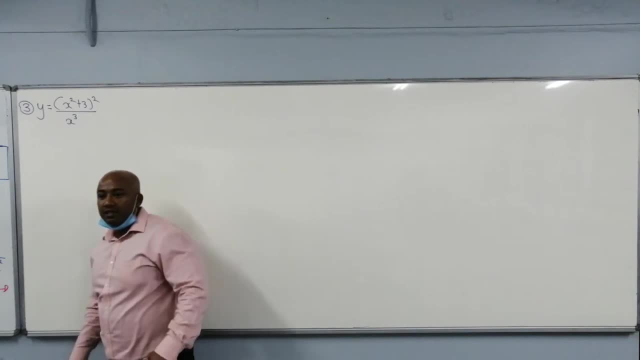 math. Any problems here? All right. So moving on to our next example, number 3.. Still dealing with last semester's work, grade 12, all and 3.. We need to simplify this here. This is not in standard form, So in order to simplify this, I need to square that. So on the top. 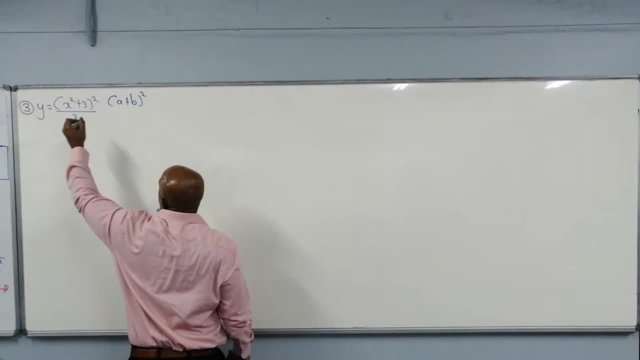 I have something in the form of a plus, So I have something in the form of a plus b squared, So which could be done in one step: a squared plus 2ab plus b squared, I can square the numerator, So y is equal. 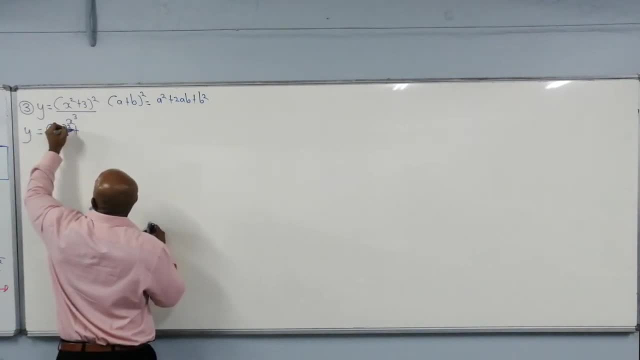 to x, squared, all squared, plus 2 times x, squared, times 3 plus 3 squared, Okay, All divided by x to the power 3.. So here I've got x squared, all squared. This can be written as: x to the power 2 times 2 is 4.. 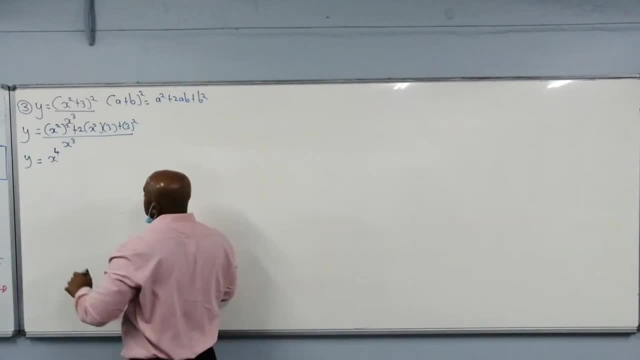 And here I've got power raised to a higher power, monthly flight to exponents. And here I've got plus 2 times 3.. That will be 6x squared and plus 3 squared, which is 9.. All divided. 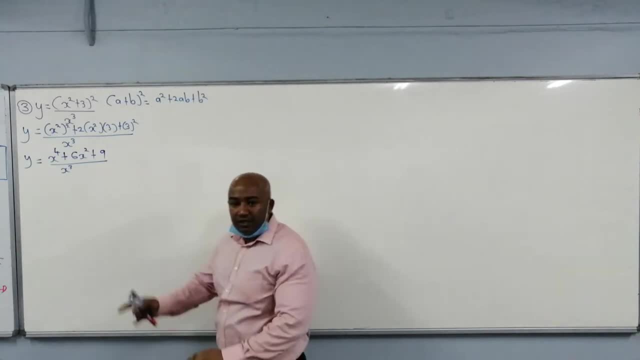 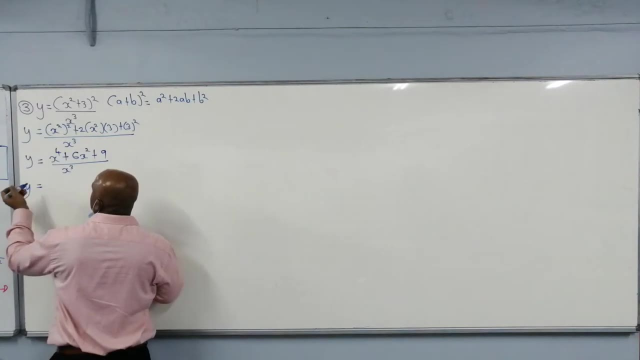 by x cubed. We still got a problem because there's division. We are dividing, So we need to separate them. We need to divide. So what I can do is I can separate this into 3 fractions because there are 3 terms in the numerator. You see that, 3 terms in the numerator. So 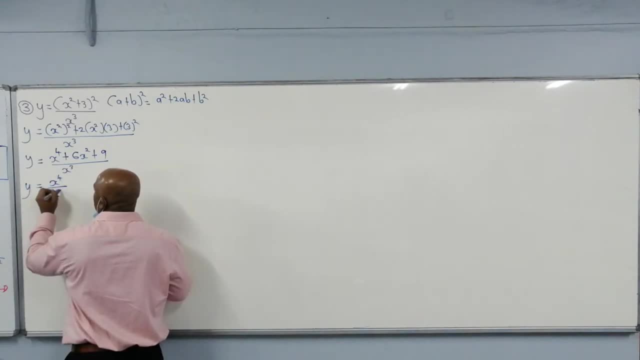 therefore, this can be written as x to the power: 4 over x cubed plus 6x squared over x cubed plus 9 over x cubed. And finally, we can simplify. So exponent laws are very important. If you do not know the exponent laws, 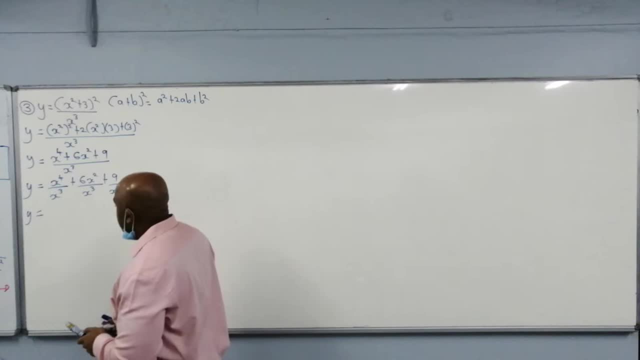 you cannot simplify what we have here, So you must be able to apply this exponent laws. So now I'm going to simplify. So what do I have now? Here I am dividing and the basis are the same. So if I have x to the power p divided by x to the power q, when I'm dividing, 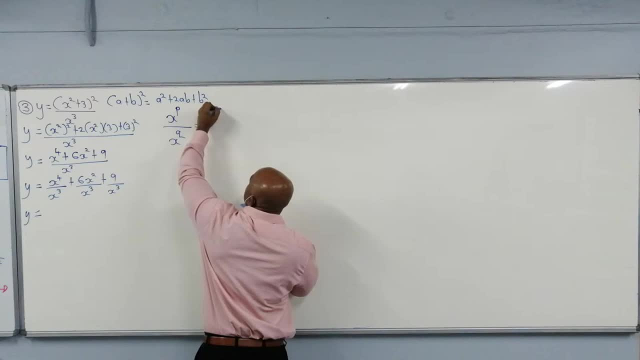 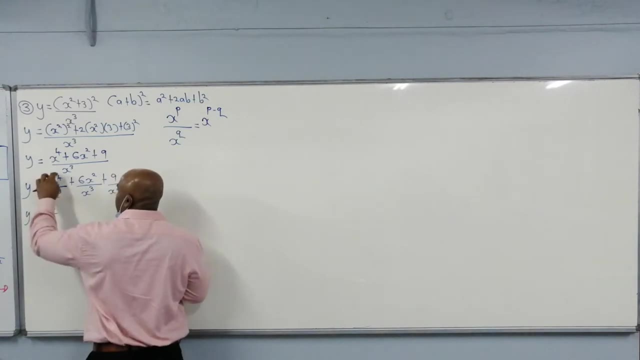 and the basis are the same. I write down the base once and subtract the exponent. That is the exponent laws. So here that's exactly what I'm going to do: x to the power, 4 minus 3,, which is 1, plus 6 divided by 1,, which is 6.. Here, 2 minus 3 is minus 1.. It's always. 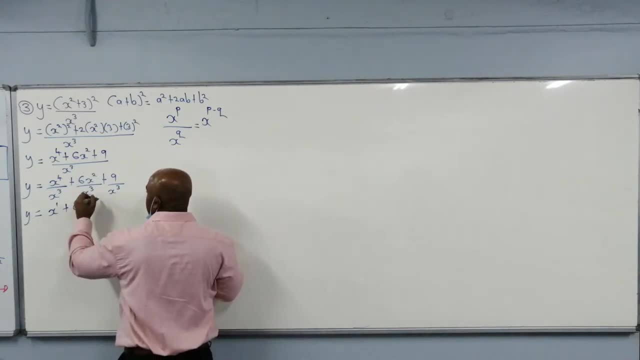 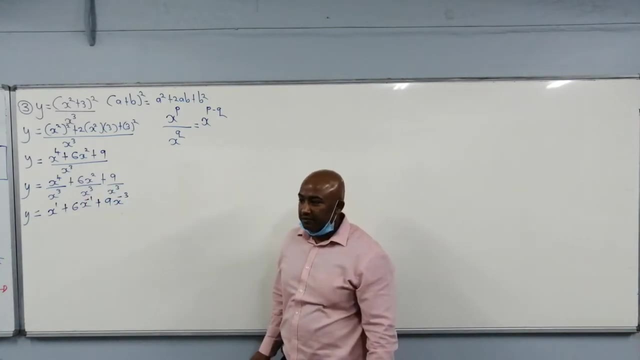 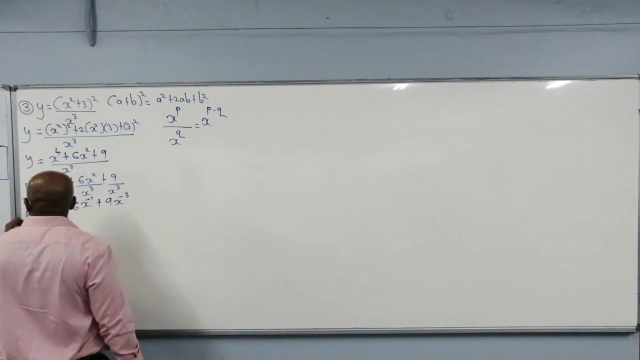 top power minus the bottom power. Here all I will do is take this to the top. It becomes 9x to the power, negative 3.. Can you all see that? Now, finally, I can differentiate. So I'm going to go dy over dx. Okay, so remember. 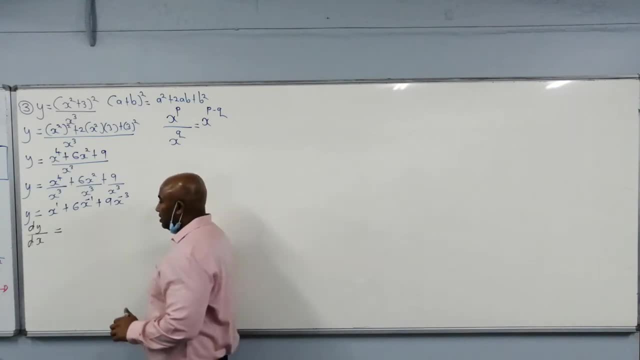 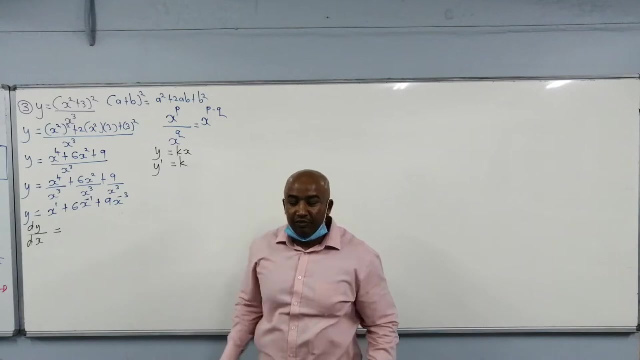 that I'm differentiating both sides with respect to x. So the derivative of x to the power 1, remember we just did that. If you have y is equal to kx, the derivative is just going to be k. The derivative of x to the power is a positive 1 only. So what's in front here is a 1.. So 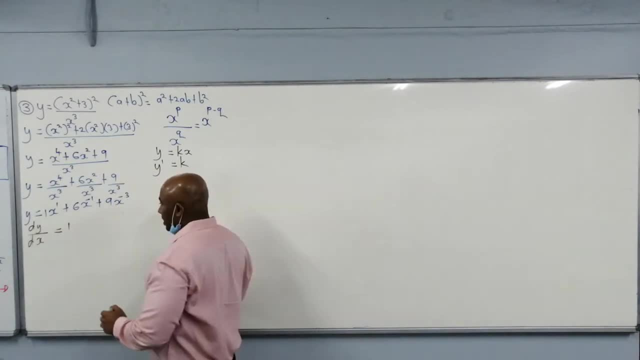 the derivative of 1x is just 1.. The derivative here 6 times minus 1 is minus 6x Minus 1 minus 1 is Minus. 2. Here 9 times negative 3 is minus 27x Minus 3 minus 1 is Minus. 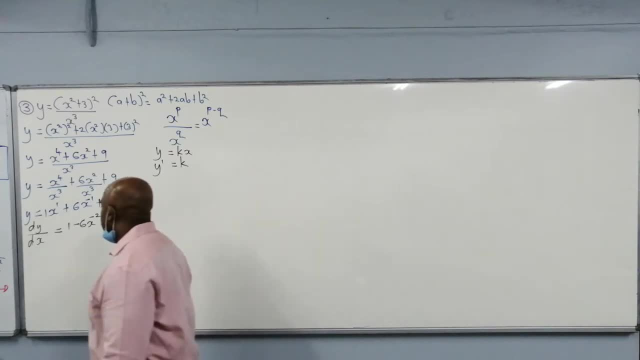 4.. Now I'm going to simplify and write the answer to positive exponents. So therefore my dy over dx is equal to 1 minus 6 over x squared minus 27,, all divided by x to the power 4.. All right, So now that was revision of. 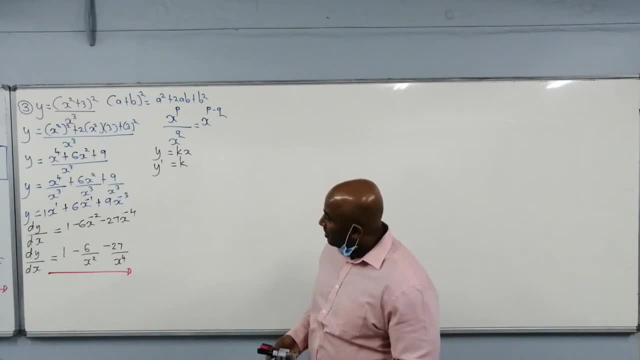 n3 work plus grade 12 stuff. Now let's deal with the next example. So what do we have now? We have 2 sine 3x, So y is equal to 2 sine 3x minus 4, cos 5x plus 3 tan 1-th x. 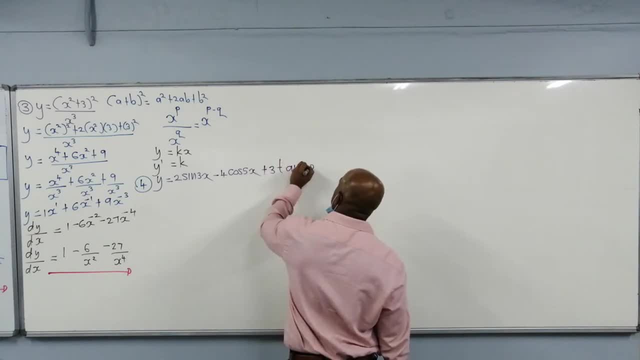 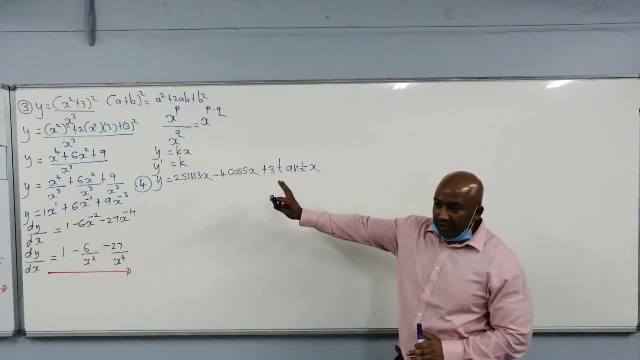 Okay, So now…. ok, Okay, So, just like with your variable x, x to the power n, it must be in standard form. The same applies for anything. So these are all standard forms. They are all in standard form. They appear on your table of derivatives. 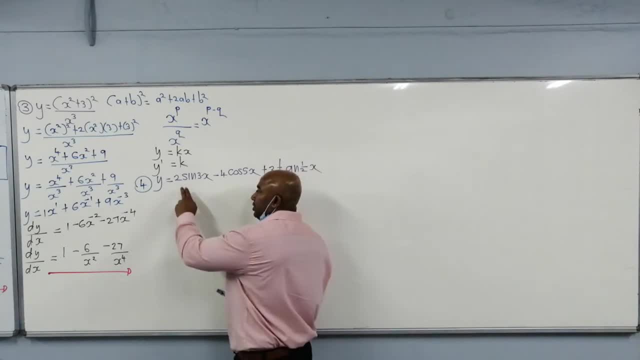 Okay, now here you read this: This is 2 sine. Now notice how do I have a person down there? You've got your y is equal to k sine and then your function of x there, So that's f of x. 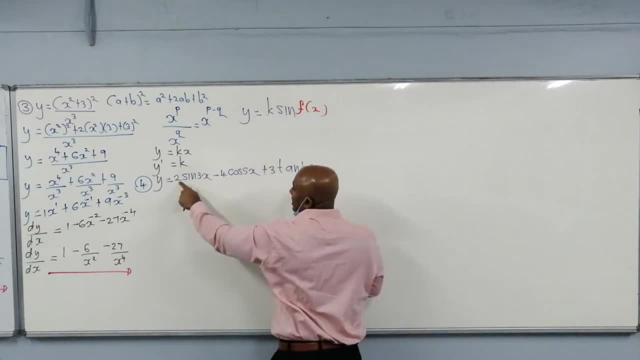 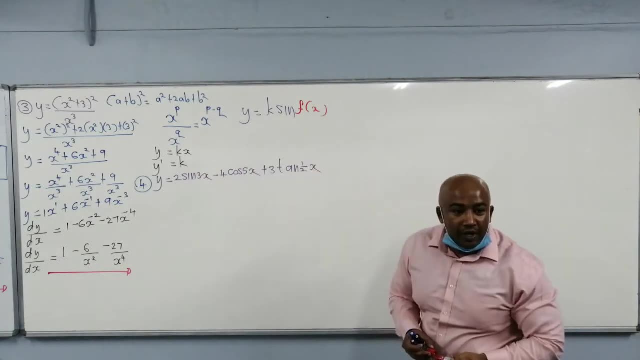 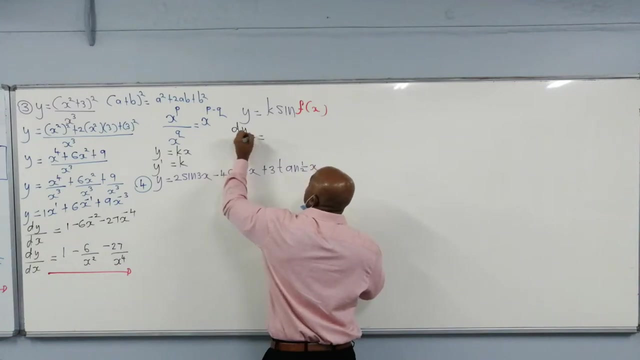 So if we compare here now the number in front, there is 2 sine of f of your function of x, here is 3x. Can you understand? Can you see that? So when we differentiate, when you differentiate, so that's going to be dy over dx, the derivative of k sine f of x is going to be k cos of the f of x. 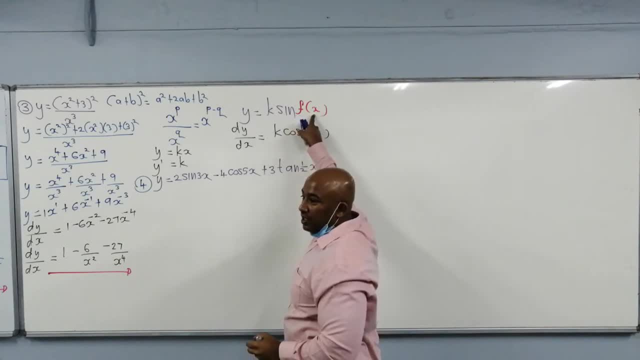 So basically you're differentiating sine of your function, which the derivative is going to be cos of that same function multiplied, okay, multiplied now by. you find the derivative here and you write down your answer here. So basically it's multiplied by the derivative of f of x. Everywhere on that table you can see, you always have f prime x. 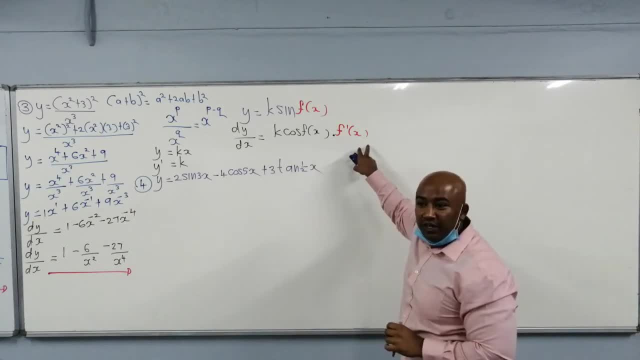 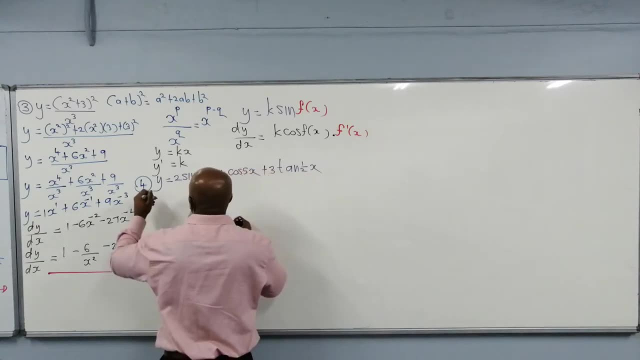 That means differentiate what you have here, write down your answer. Okay, that's how we deal with this, So let's deal with this one. So I've got dy over dx. So the derivative of 2 sine of 3x is going to be 2 cos of 3x. So basically, what's happening is you're differentiating sine, which becomes cos times. now you're differentiating 3x, The derivative of 3x is going to be 3.. That's all simple. 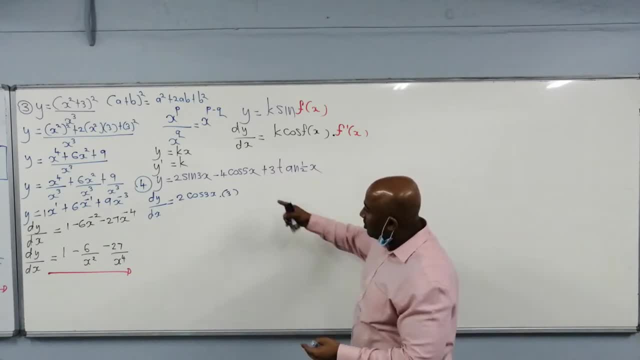 That's how you apply a formula. So the same goes for cos 10.. Look at your table of derivative then. So the derivative of cos. now I've got a minus 4 there. ok, remember, it's minus 4 times cos 5x. 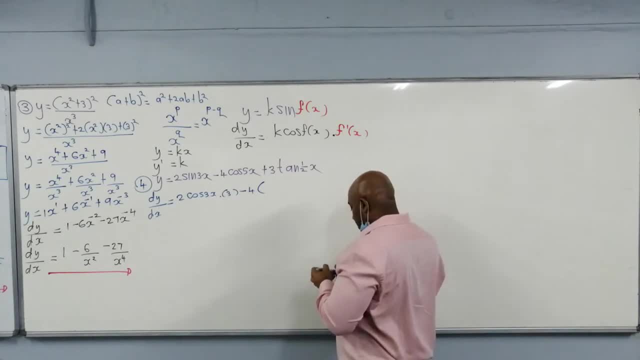 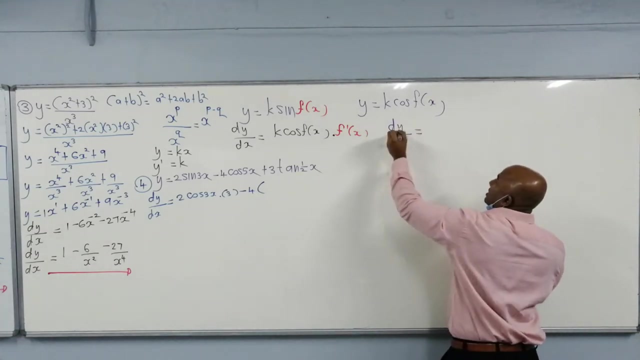 so the derivative of cos. if you look at your table, let me just write this down, ok, since the table is up in front of you. so if I've got y is equal to k cos f of x, then the derivative there dy over dx. the derivative is going to be minus. 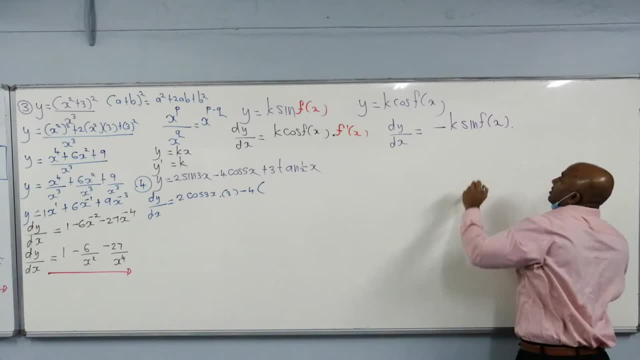 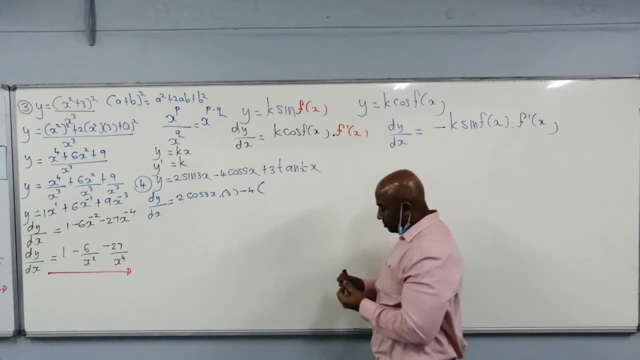 k sin f of x. so the derivative of cos is minus sin times f of x. so here the derivative of cos of 5x is going to be minus sin of 5x. or if you wanted to keep the 4, it doesn't make a difference. all multiplication. 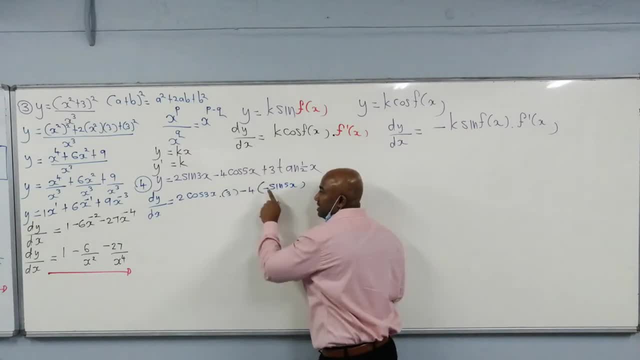 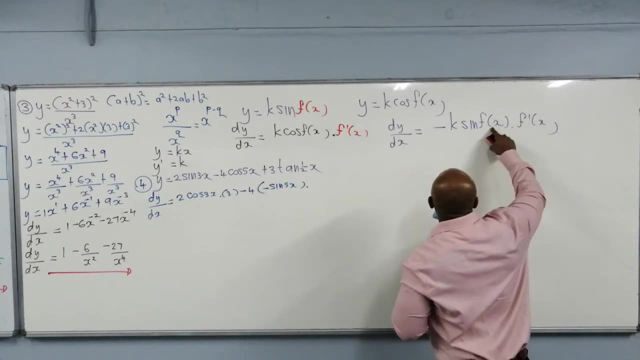 right, but the fact is the derivative of cos is a negative sin of the function of x. times now. times now. differentiate what's here and write it down here. so the derivative of 5x is 5. ok with that. now term 3 is: 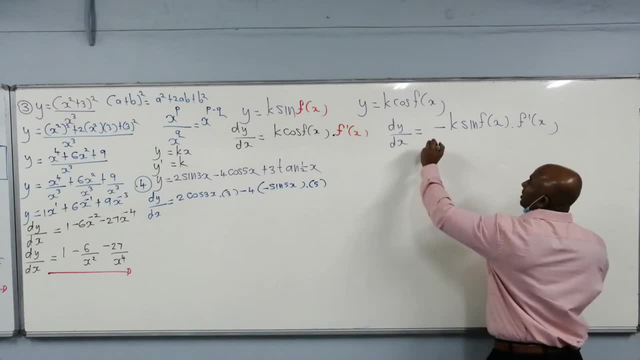 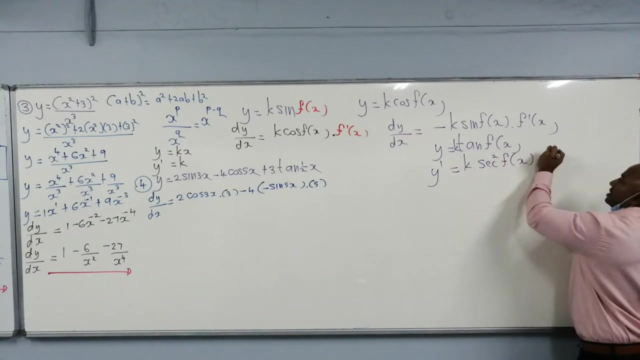 10. so let me just rewrite 10 for you there. so if I've got y is equal to 10 f of x, then the derivative of 10 is 10. f of x is going to be step squared f of x times f prime x. 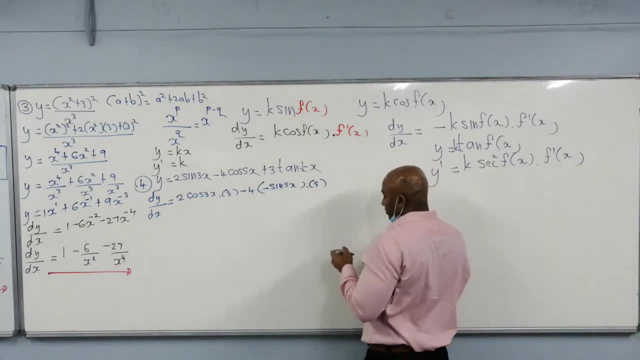 so the derivative of 10 of half 3, 10 of half x, will be 3 step squared of the function of x, which is half x. so we're at this point here. times now differentiate f of x. write down your answer here: what's the derivative of half x? 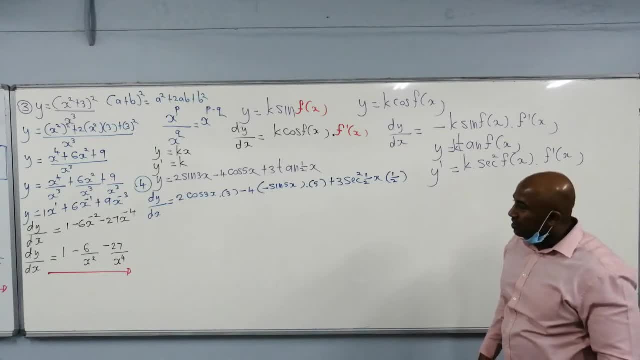 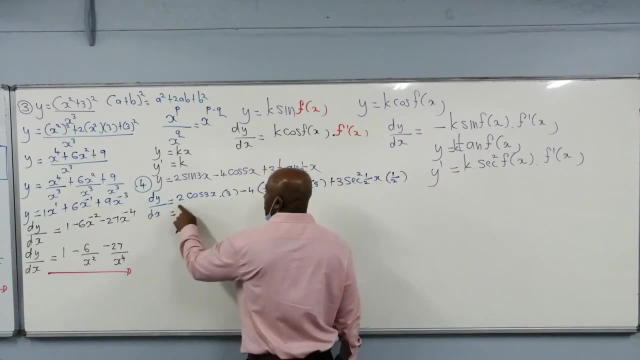 it's just half right, you're done now. that is it. it's just to simplify. multiply the constants. so 2 times 3 will be 6 cos 3x- here negative times negative is a positive. 4 times 5, here is 20 sin 5x. 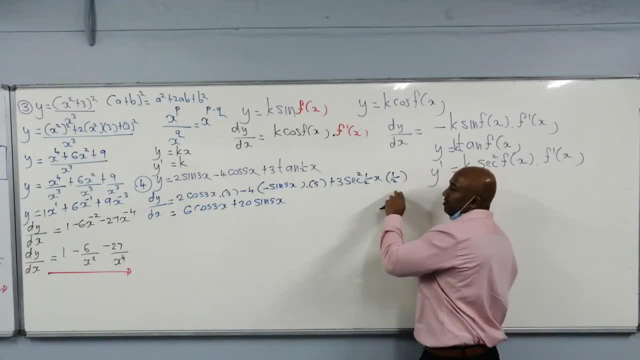 here we've got 3 times 1 divide by 2, which is the same as 3 times 1, which is the same as 3 times 1, which is the same as 3 times 1, which is the same as 3 over 2. 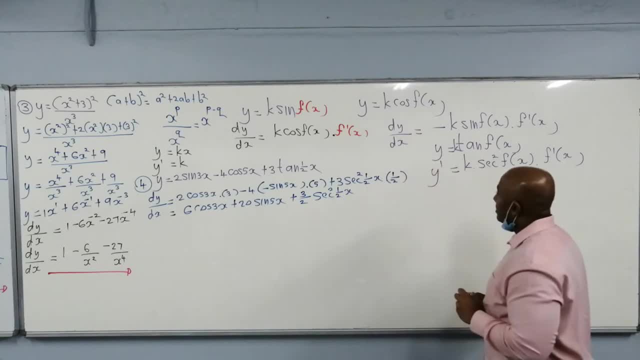 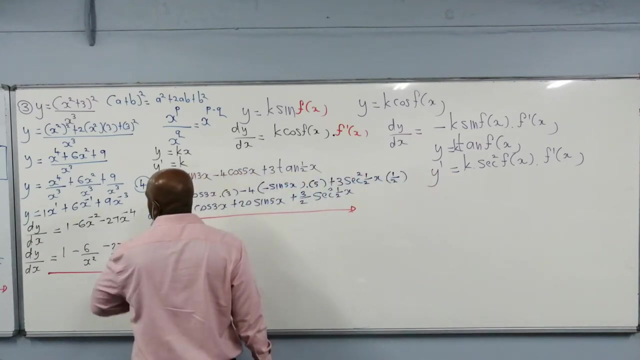 step squared f of x, and that's basically it. so differentiating using the table of derivatives very easy. ok, that is number 5. now we've got 2 cos 5x. we have 2 cos 5x minus 2 sin x over 3. 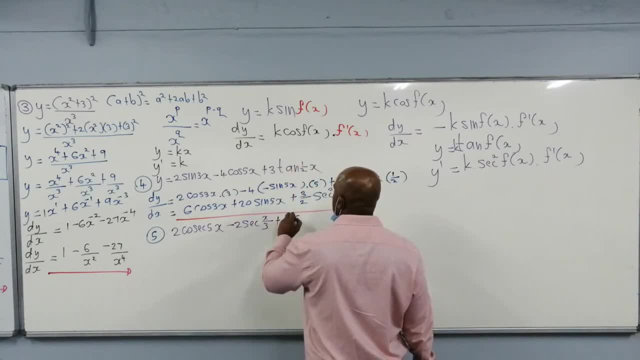 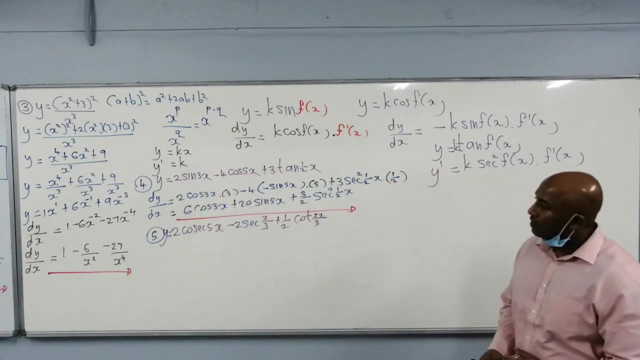 and plus half cot of 2x over 3, right? so what are we dealing with now? we are dealing with cosec. so if y is equal to k, cosec f of x from your table of derivatives, then the derivative of cosec is going to be a negative. 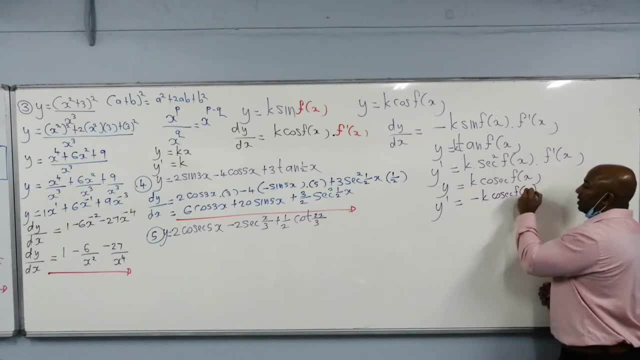 cosec f of x times cot f of x times f prime x. that is the formula to differentiate cosec. what is the next one? we have sec. if y is equal to sec f of x, then the derivative of sec is going to be sec f of x. 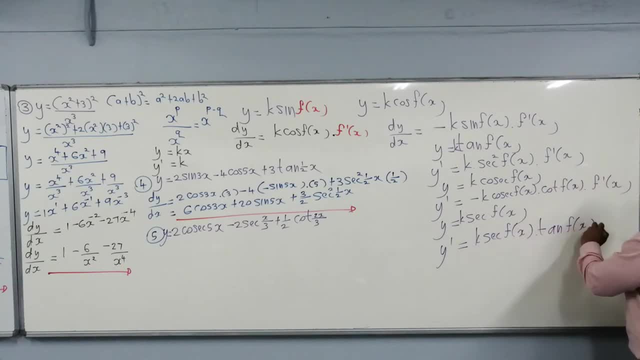 times tan f of x, and always after you differentiate your trig function, then it's the derivative of f of x as she comes: f prime x. what is the last one, cot? so if y is equal to cot f of x from your table of derivatives, then you differentiate cot. 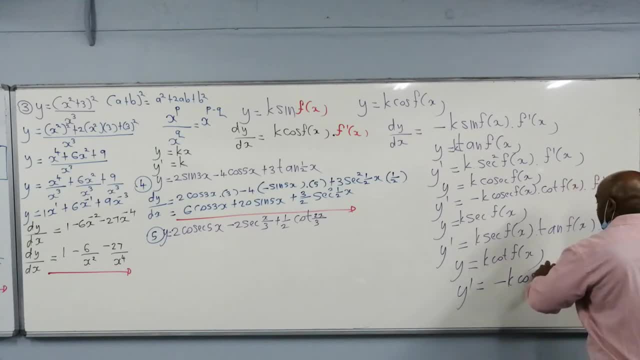 that's going to be negative. cosec: squared f of x and then times f prime x, right? you write it down a hundred times and it's in your head, right, it will help you to get full marks here. but obviously not it will help you. 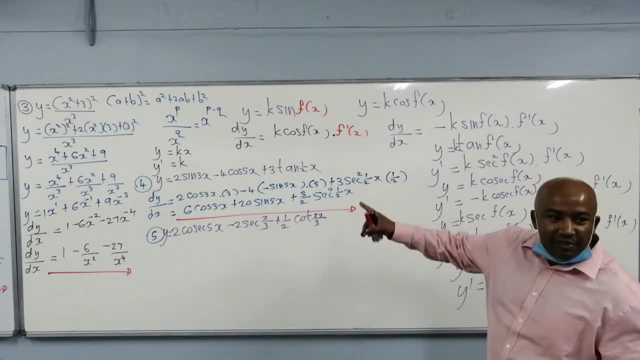 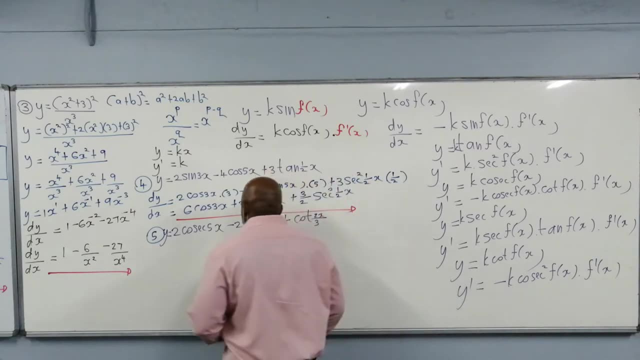 but in order to get full marks you have to know simplification- how to rearrange something- and you have to know your exponent laws. so now let's differentiate this. so I've got y is equal to 2 cosec there, so dy over dx. so here is the formula. 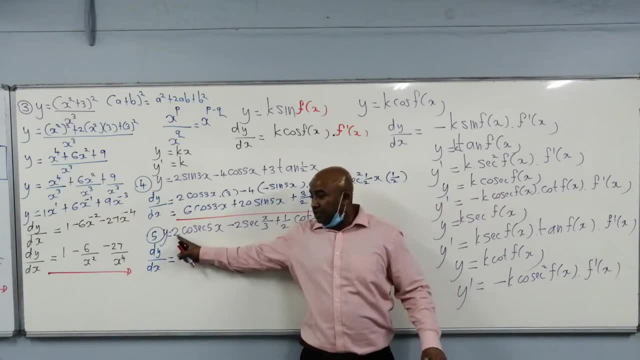 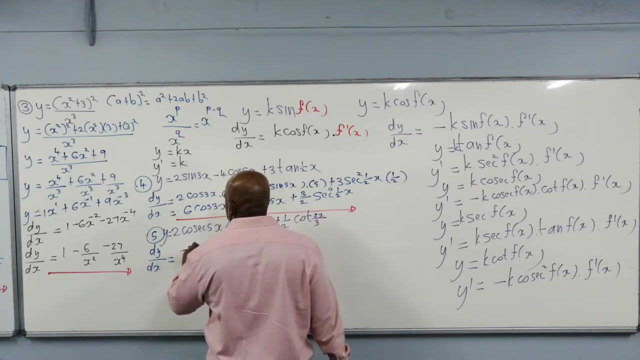 I've got 2 cosec f of x, so there's my 2 there. that's 2 cosec 5x. f of x is 5x. alright, differentiate the derivative of 2 cosec 5x will be negative: 2 cosec 5x. 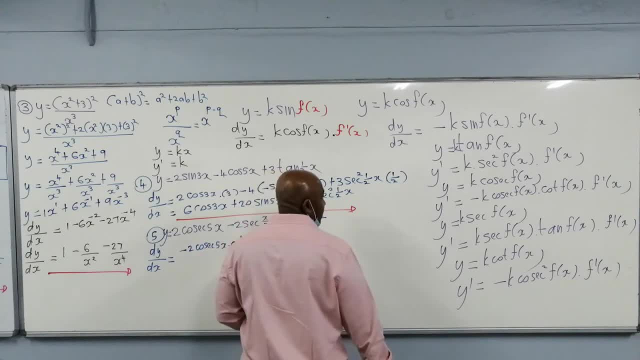 times cot, 5x. so where am I now? I'm going negative cosec times cot and then at the end always f prime x. so that's going to be times f of x is 5x. so f prime x is the derivative of 5x, which is 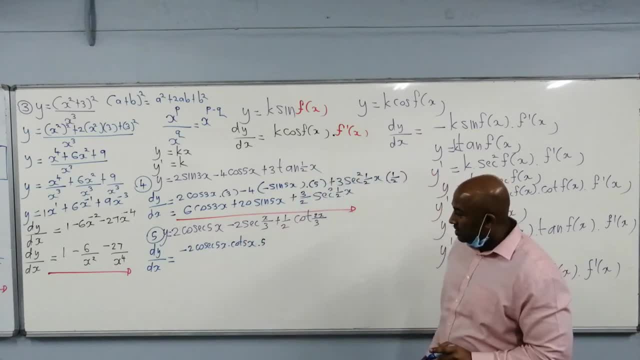 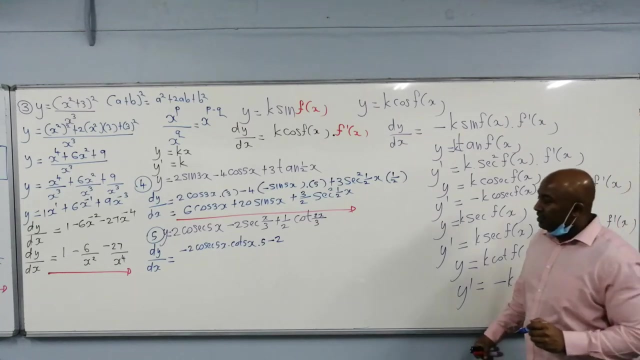 5. so that is cosec here the derivative of sec. so that's minus 2. when you have where is sec, there's sec. here the derivative of sec is sec f of x times 10. so you can see that. so the derivative of sec there is going to be. 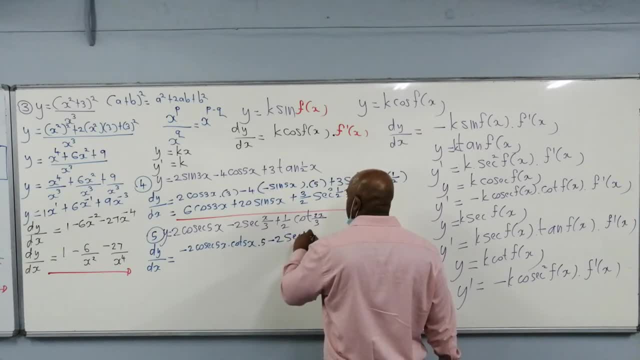 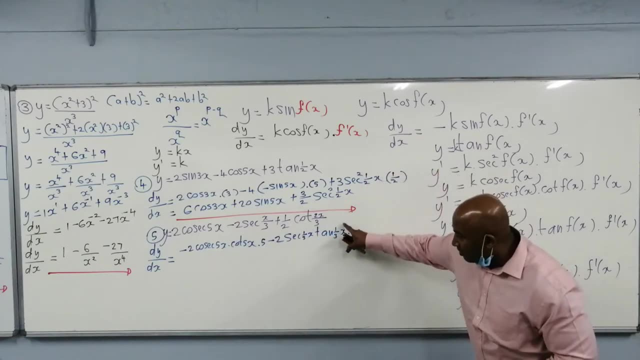 sec. 1 over 3x times 10, 1 over 3x times the derivative of 1 over 3x, which is 1 over 3, 1 over 3, cot- where is cot? there's cot here? the derivative of cot of f of x is going to be negative. 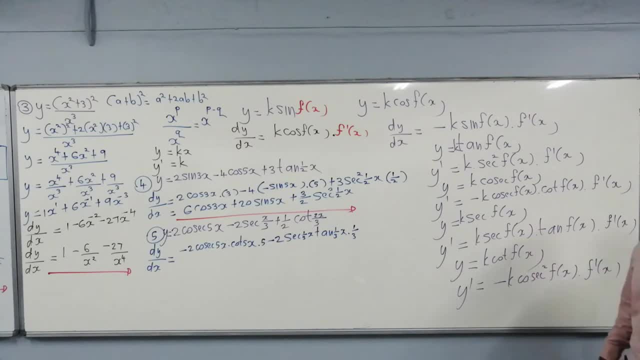 cosec squared f of x times f prime x. so the derivative of positive half will be negative, half will be negative. half cosec squared of 2 over 3x times the derivative of 2 over 3x, which is 2 over 3. 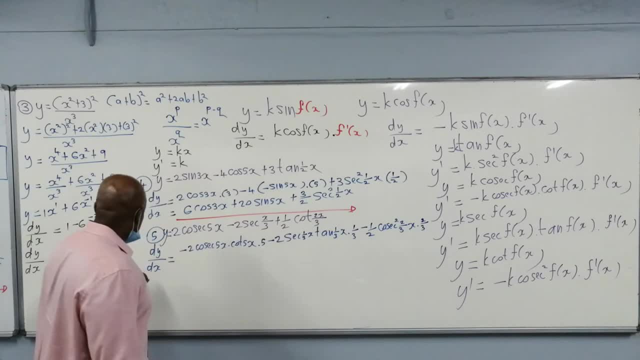 so that's basically it. let's simplify. so what do I have? I'm just going to multiply the constant, so that's going to be minus 2 times 5x, minus 10 cosec, 5x times cot, 5x, then term 2. 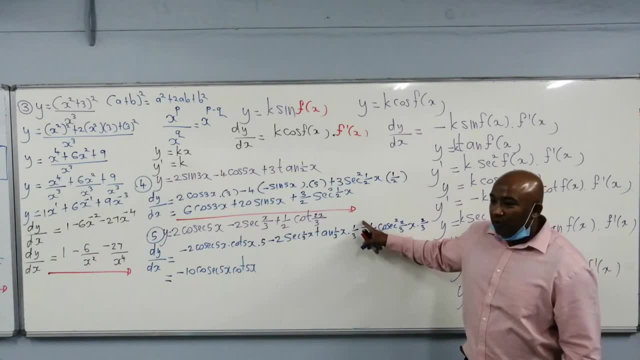 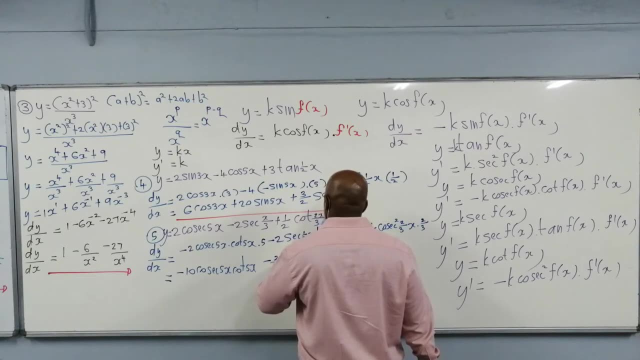 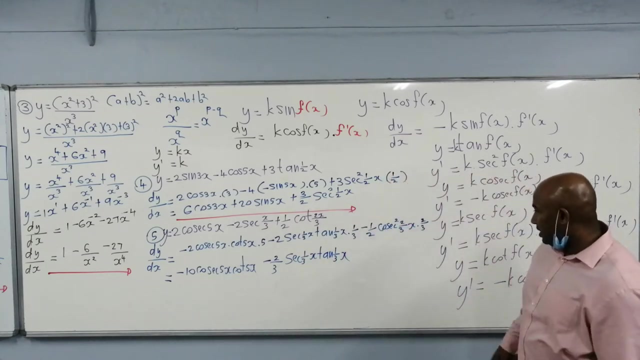 what do I have here minus 2 times 1 over 3, so that's going to be minus 2 over 3 sec. 1 over 3x times 1 over 3x here. what do I have here minus 1 over 2? 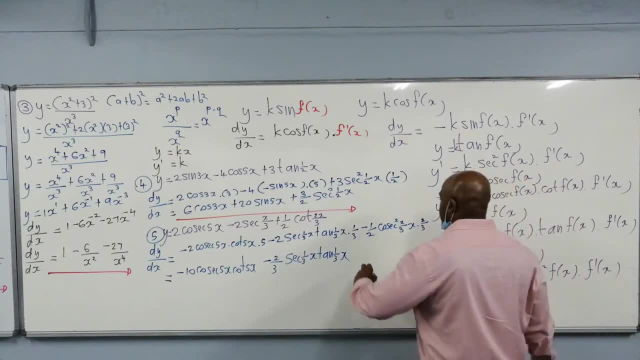 times 2 over 3. so 2 and 2 cancel. I end up with minus 1 over 3. cosec, cosec squared 2 over 3x. that is just a simplification. you make sure you know these. this must be in your head. 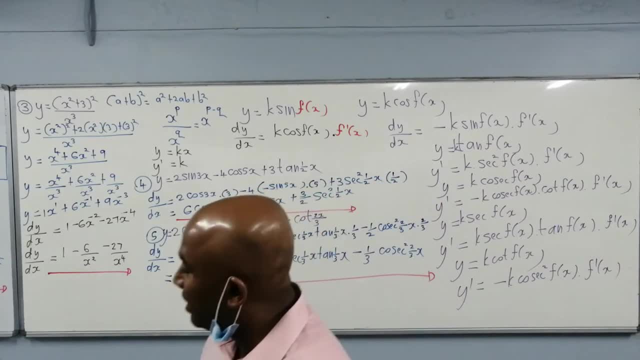 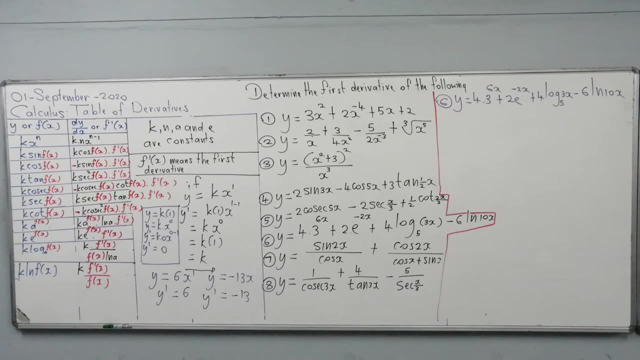 all right, so I'm going to erase the board so we can deal with the next few examples there. all right, number 6. so here we've got 4. be careful, this is not 43, it's. this is 3 to the power. 6x. 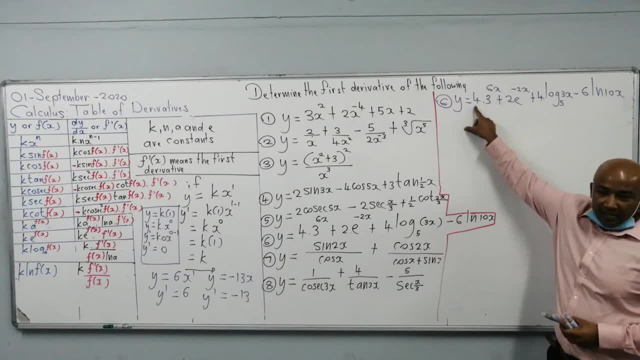 and this whole thing is multiplied by the number 4. that's how you read it. so it's 4 multiplied by 3 to the power 6x. this is 2 multiplied by e to the power minus 2x. okay, e is a constant. 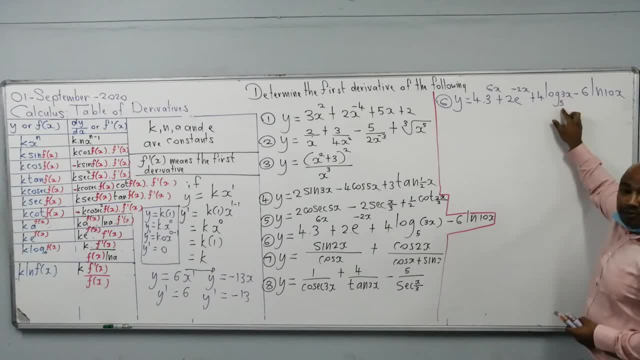 and here we've got 4 log 3x base 5 here, minus 6 linx, minus 6 желiano, minus 3liz, right, so these are normal. so these are all points equal to of x. so here we, let's give it a follow up. 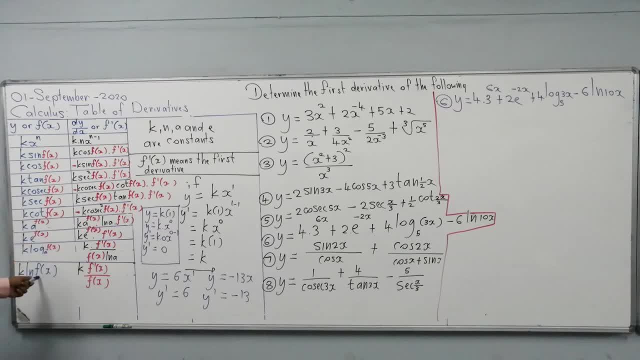 remember that infinity of x is the out of the center of this circle of over dx. So how do you differentiate? Now you look at, there's a table in front of you. When you differentiate your exponential function, step number one is to copy it down. 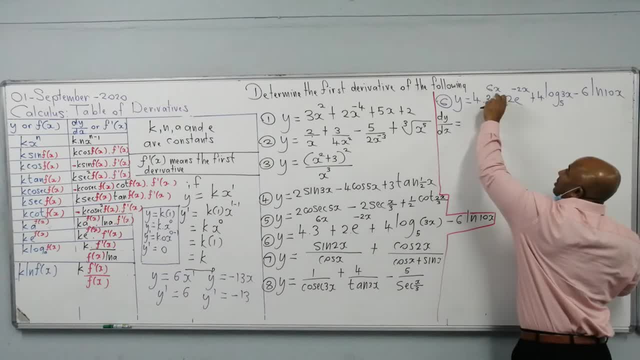 as it is. So k times a to the power f of x is k times a to the power f of x. That is step one. You can see it Times now. you put ln as natural log of the base. What is your base 3.? 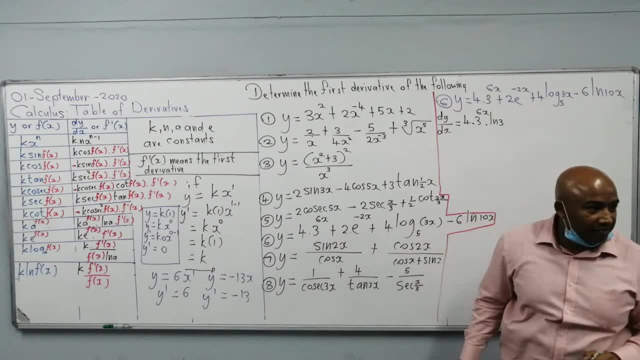 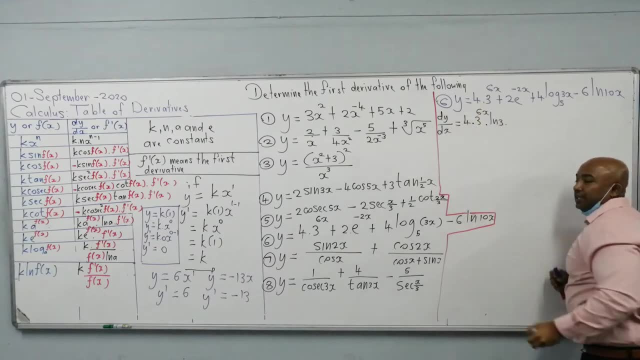 You can see ln of a. a is the base. Can you see that Times? now the last thing you're going to do is the exponent is f of x, So you differentiate the exponent and write down your answer there. 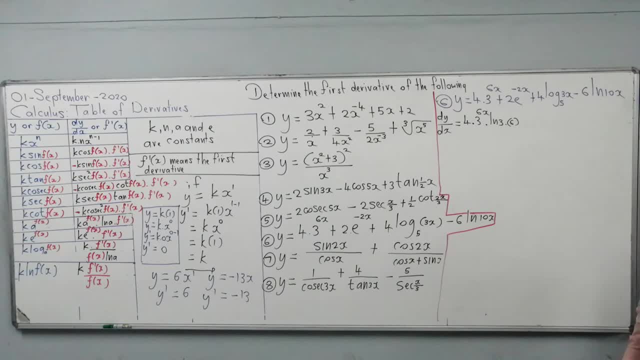 Multiply, so that's times 6.. Are you clear with that? So that's going to be k a to the power f of x times ln, a times f, prime x, This one. When you're doing this, your base is e, So basically. 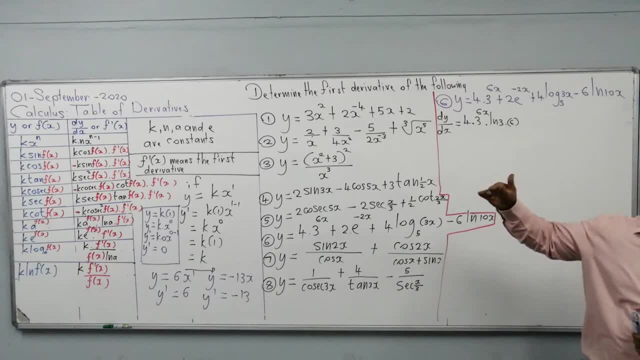 you can use the above formula k a, the one that we just used, But when it's e, there's no need to put the ln back there. So we've got plus 2 times e to the power, minus 2x, And then you don't. 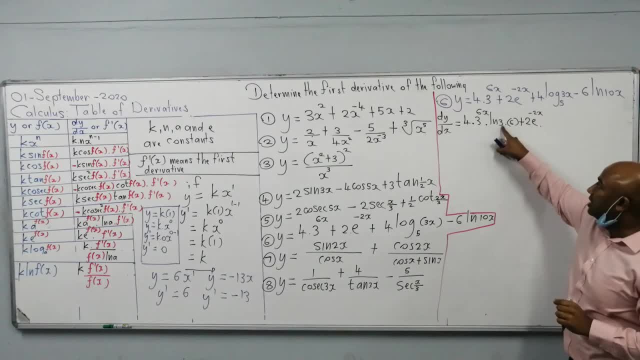 have to put down ln of e Like here. I put ln of the base. Here your base is e, because ln of e is the same as log of 10, which is 1.. So that's why it's unnecessary to put down. 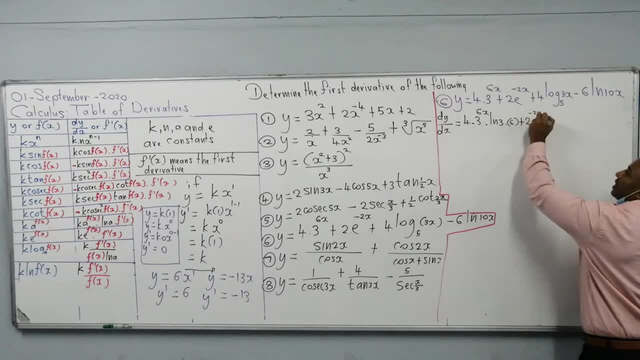 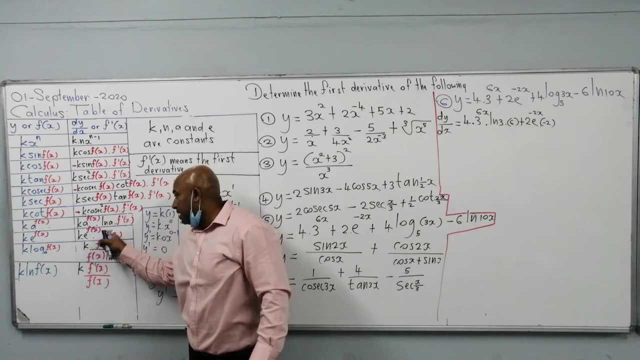 an e, You go straight for f prime x. the derivative of minus 2x is minus 2.. As you can see, there's k e to the power f of x times f prime x. Right, So here this one. 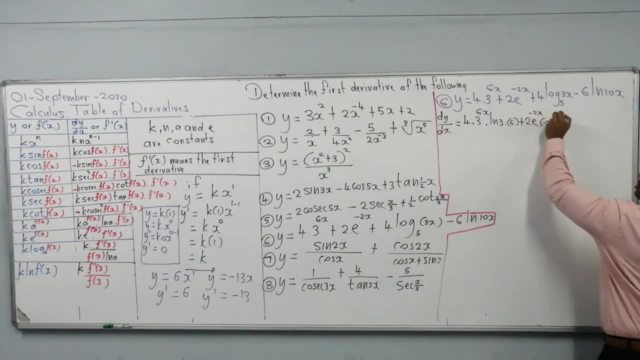 This is k. log f of x to the base a. So the rule is: you've got your 4 times. Now this is going to be a fraction, Okay, So the derivative there. this is f of x. So the derivative. 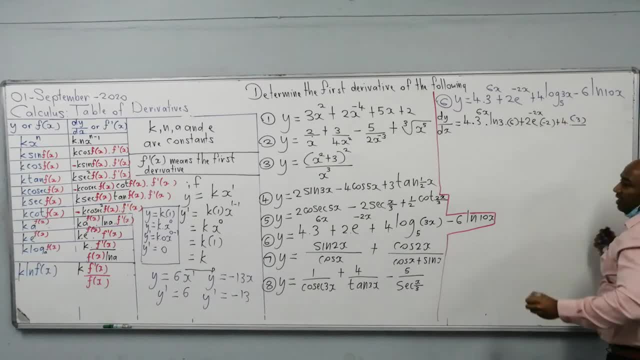 is f prime x, which is 3.. As you can see, there's a jump. Okay, f prime x, all divided by f of x. So I need to divide by the same f of x there. So that's f prime x divided by. 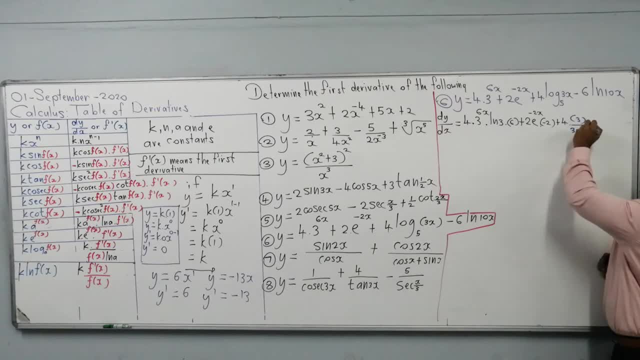 f of x. Also times natural log of the base: ln of the base. your base. there is 5.. You can see that ln of a. So there's ln a. a is the base of your log. Alright, So now. 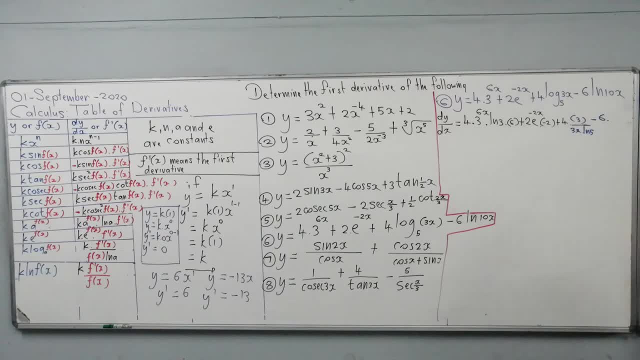 this one here minus 6 times. it's almost the same formula, Almost In fact. the base here is not shown. If your base is not shown, for natural log it is e. So the formula is f prime x divided by f of x. 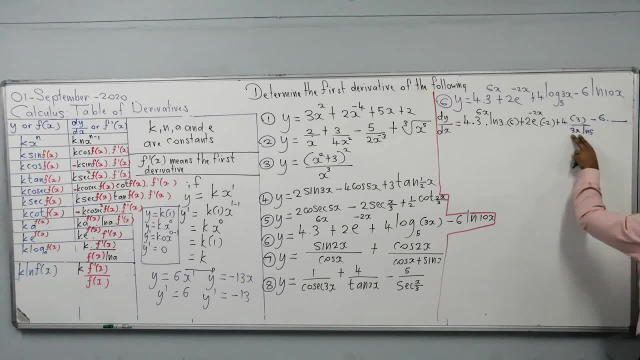 So take this f of x, just like how you took the f of x, copied it here. Take 10x, copy it in the denominator. differentiate this and write down the result: f prime x divided by f of x. And that's how we use those words. 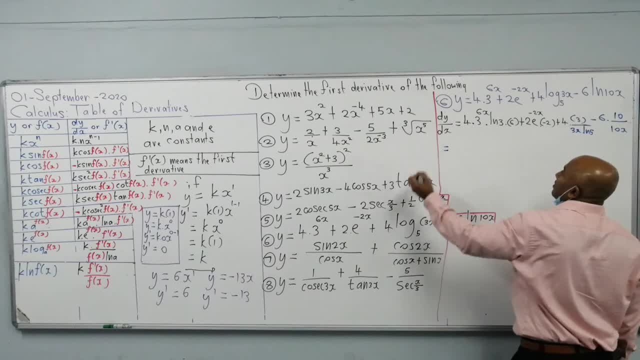 So now, what's the what's the simplifier? So here there's nothing much you can except there's a 6 there and there's a 4 there. This is not 3, this is natural log of 3.. 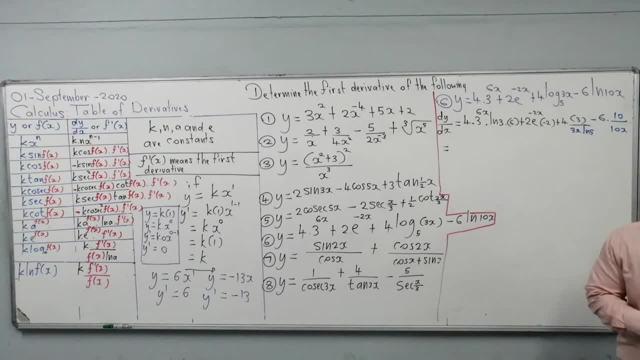 So you cannot multiply this 3 by 6 there, because it is not 3.. Right, it's natural log of 3.. But you can go 6 times 4, which is 24 times 3, to the power 6x. 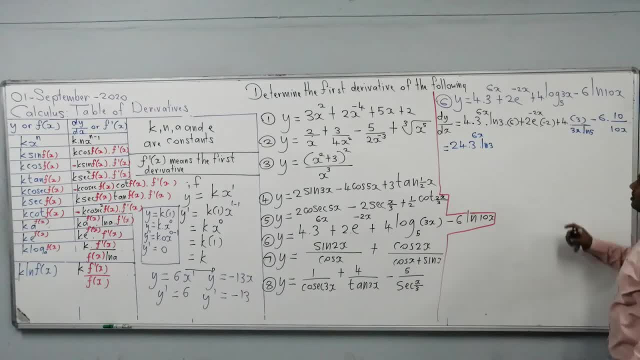 ln 3.. Here I can go positive times, negative, so that will be minus 4, e to the power minus 2x. Here 3 and 3 will cancel, So I end up with a plus 4 divided by x, natural log 5,. 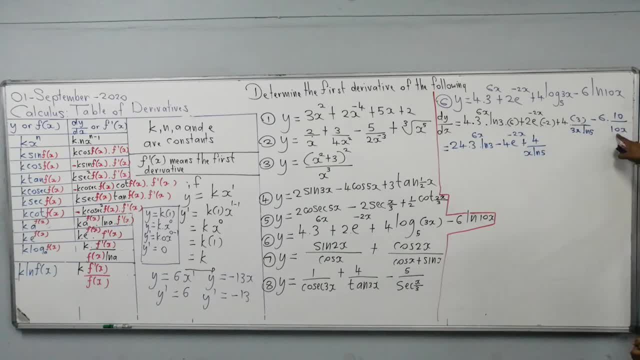 ln 5.. Here 10 and 10 will cancel. You end up with minus 6 divided by x. You do not have to make that exponent positive here, because this is the standard form for your exponent. So that was number 6.. 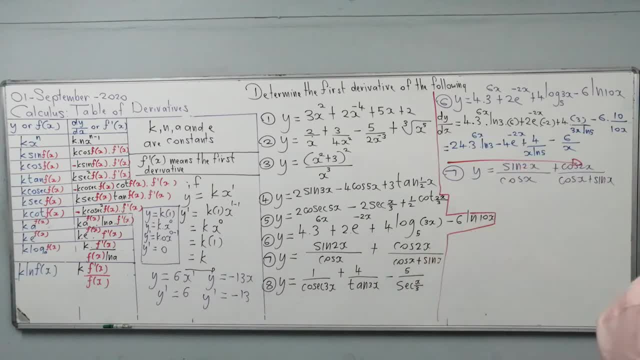 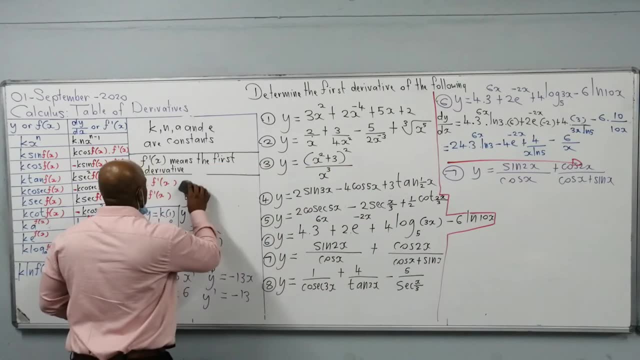 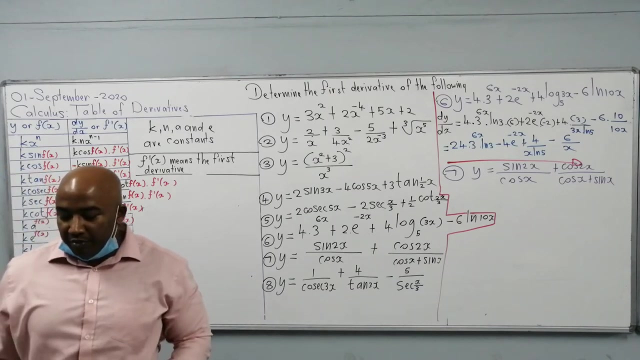 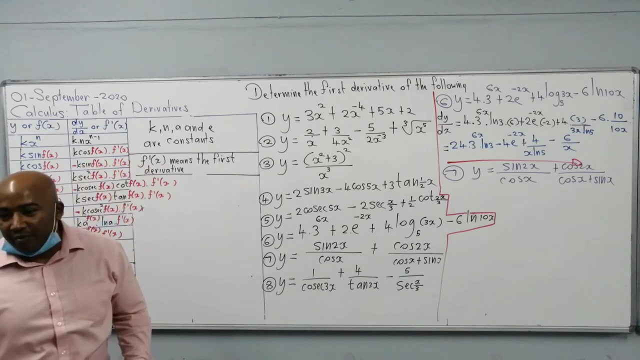 Okay, Number 6.. 7. Number 7, we need to simplify here. So the numerator is sin 2x. So in this case we need our double angle formulas from trigonometry grade 12.. So let me write it down for you. 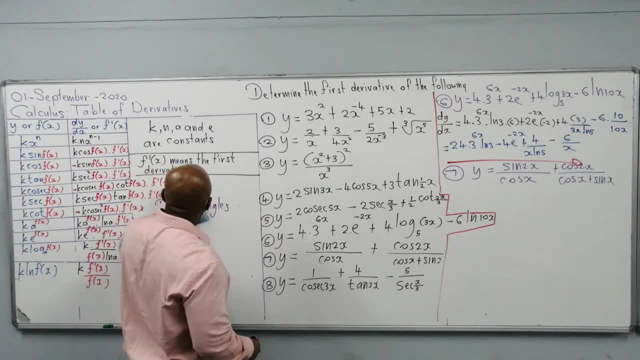 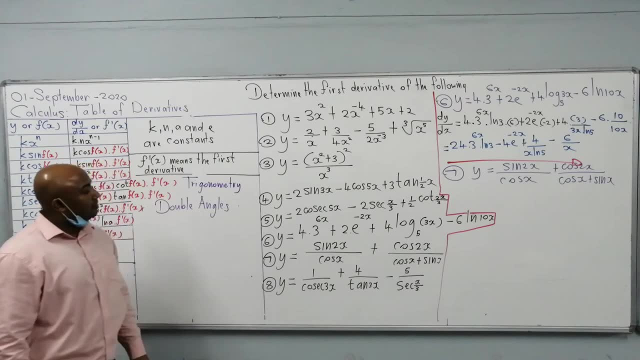 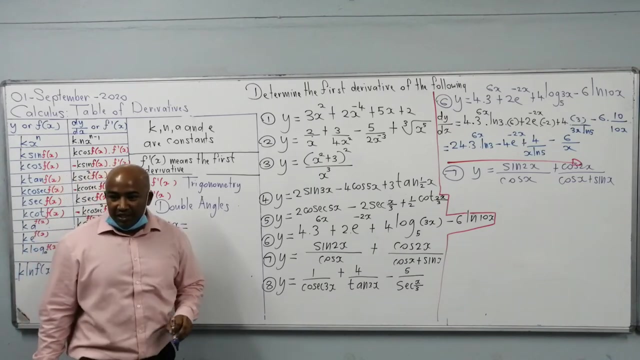 So this is trigonometry, Double angles. So we need to be able to write down the equivalent for sin 2x, So sin 2x. the double angle formula for sin 2x is going to be 2 sin 1x, cos 1.. 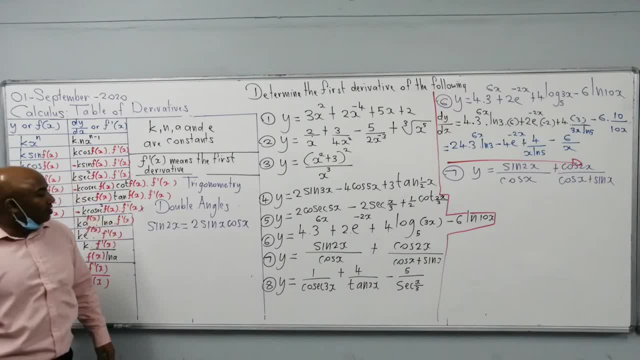 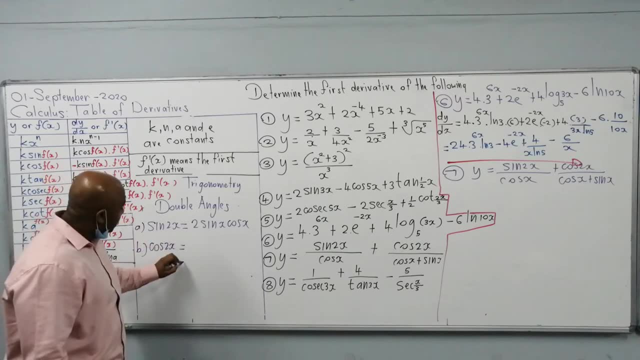 Then the double angle formula for cos 2x. There's actually 3 formulas for cos 2x. First one is cos squared minus sin squared, So remember there's a 2 there and that becomes a 1 and a 1 there. Then the second one is 1 minus sin squared, So remember there's a. 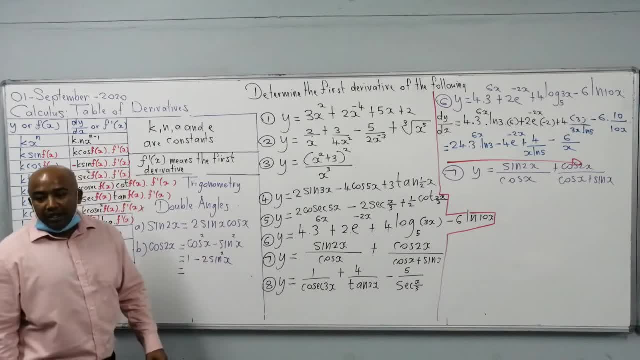 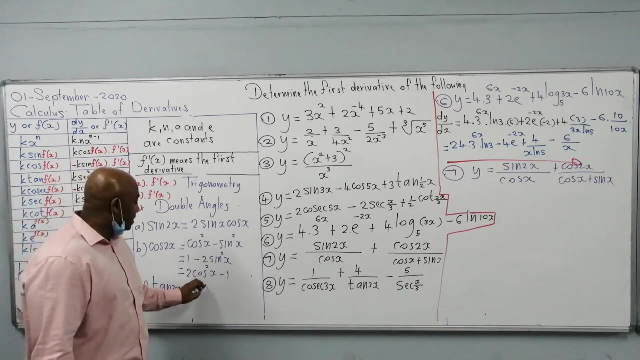 minus 2 sin squared. And then the last one, for cos 2x is 2 cos squared x minus 1.. And then we also have a formula for tan 2x, which is going to be 2 tan x all divided by 1 minus. 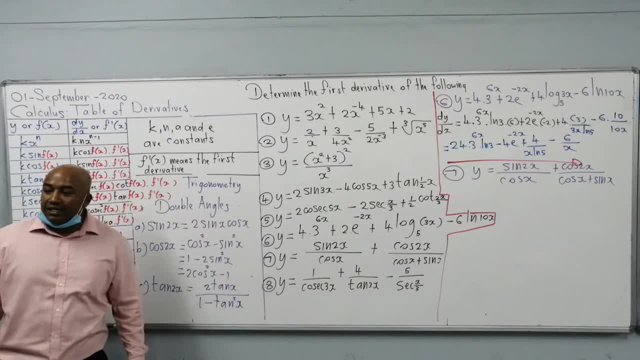 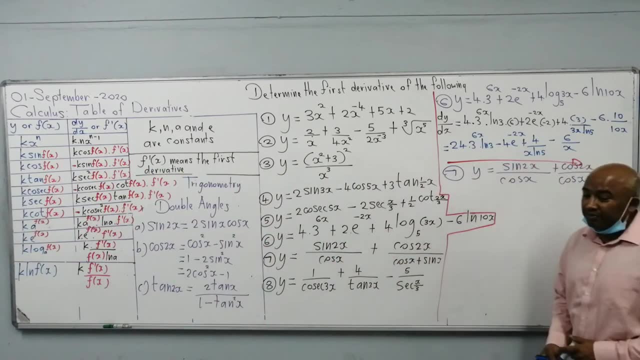 tan squared x. Right? so those are the double angle formulas from trigonometry. We might have to use it. Yeah, in fact, we are going to be using it. So the problem is that this is a double angle and this is not, it's just a single, It's just 1D. Can you see that? So we cannot go. 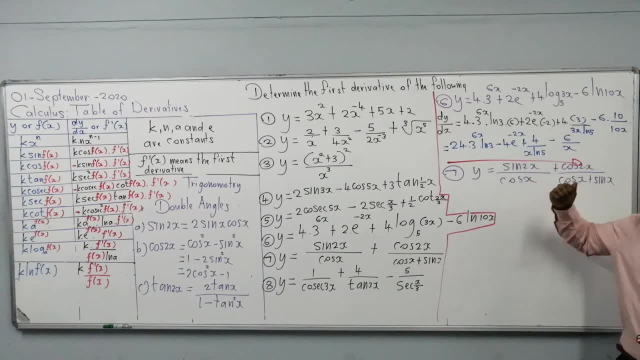 sin over cos, It's tan, Only sin over cos. If the angles are the same, then it's equal to tan. Okay, so here I will have to apply my double angle formula. So I've got: y is equal to 2.. 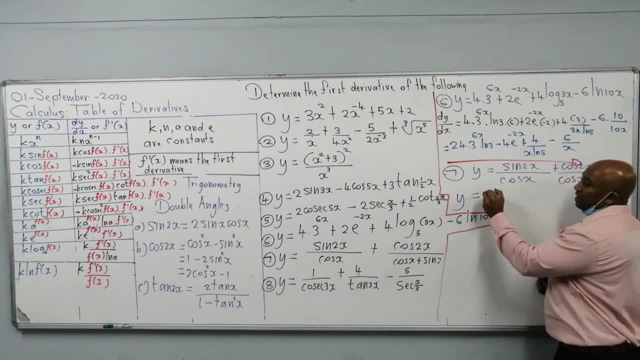 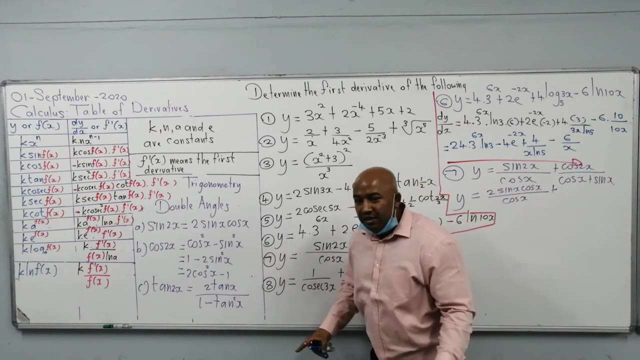 So sin 2x. there's only one formula for sin 2x, which is 2 sin x. cos x all divided by cos x. Okay, now cos 2x. there's three formulas for cos 2x. Which one is best suited for this? 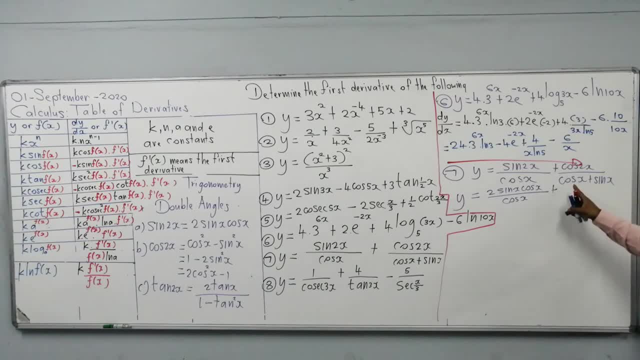 example, It's the formula that has both cos and sin in it, because look at the denominator. The denominator is the clue. The denominator has both sin and cos. So use the formula that has both sin and cos. So it's going to be cos squared minus sin squared, all divided by cos x plus sin x. Now it still. 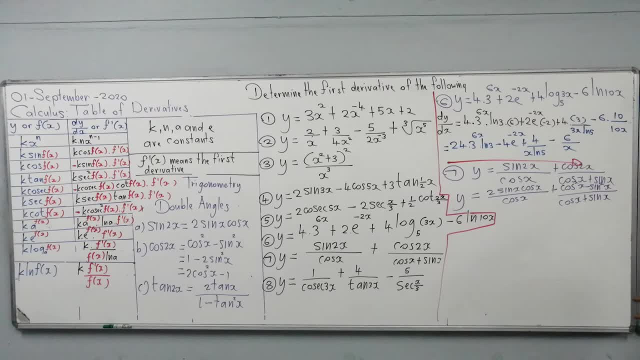 does not cancel, because you cannot cancel terms, You can only cancel factors. This one does not cancel at this stage, but clearly for this cos and cos, Can you see that? So now let's see what happens here. We've got: y is equal to 2 sin x plus. 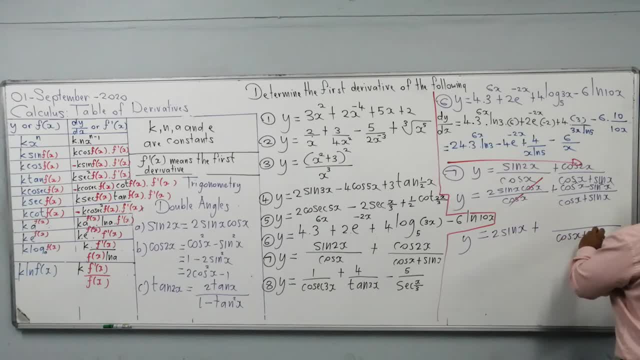 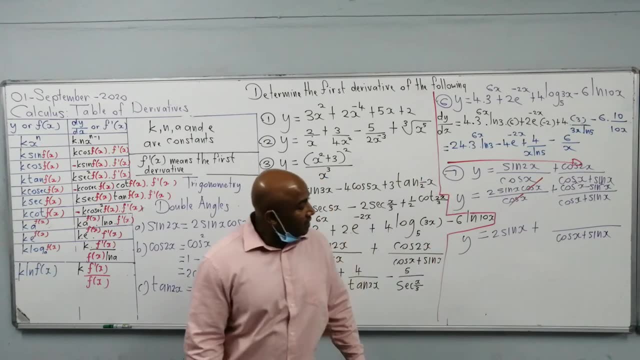 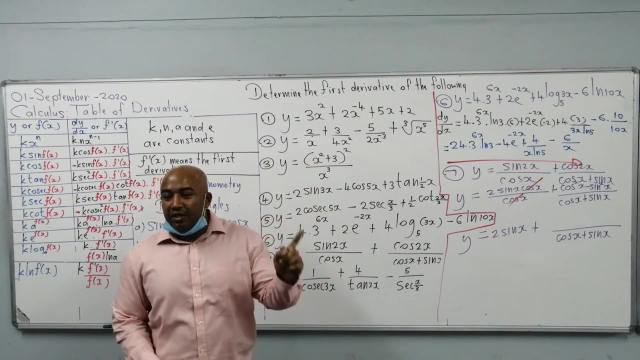 here I've got cos x plus sin x in the denominator, But what do you notice about the numerator? Cos squared minus sin squared. Notice that there's a negative sign and on the left there's something squared, on the right something squared. So this is the difference of cos. 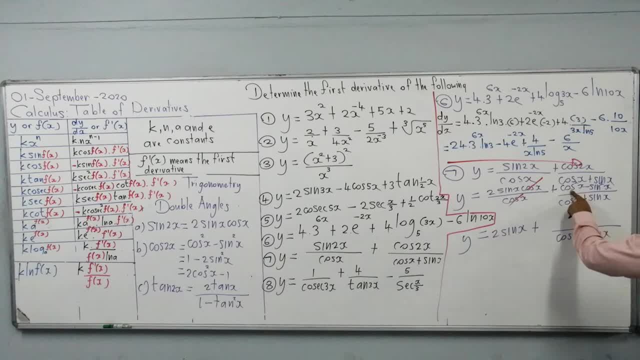 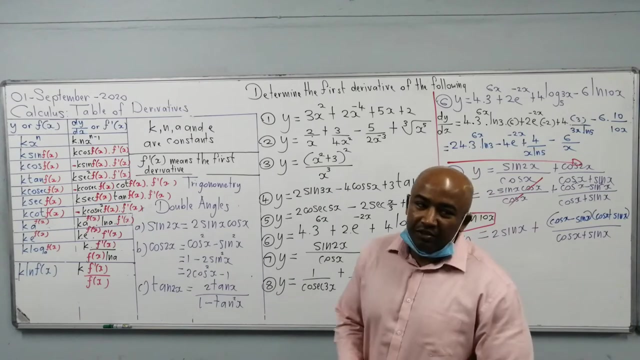 This is the difference of 2 squares. That means we can factorize. This is the difference of 2 squares. We can factorize. So it's going to be a minus b, a plus b. So we will factorize and that will be cos x minus sin x, cos x plus sin x. Can you see that? So you have. 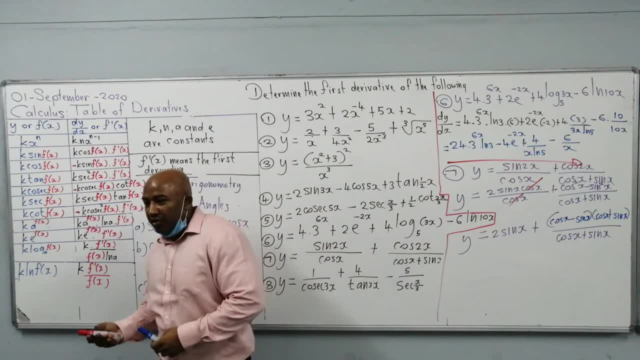 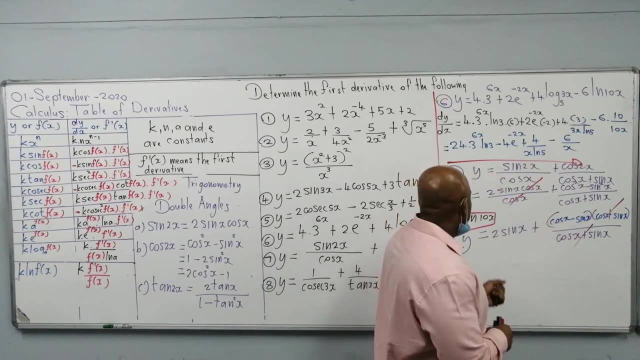 to. besides knowing the formula, you have to know how to factorize, You have to know which formula. This is another type of formula to use. So now, clearly, that and that cancel. Can you see that? So now what remains? What remains is: y is equal to 2, sin x plus, cos x minus. 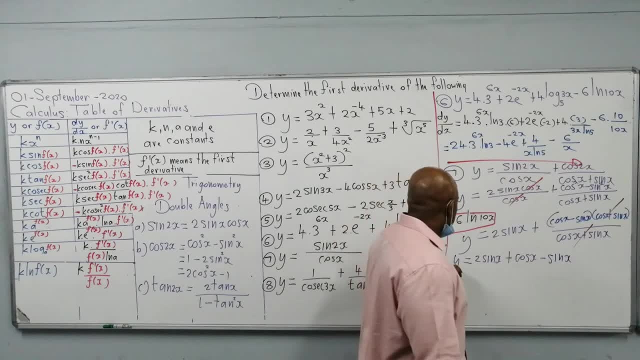 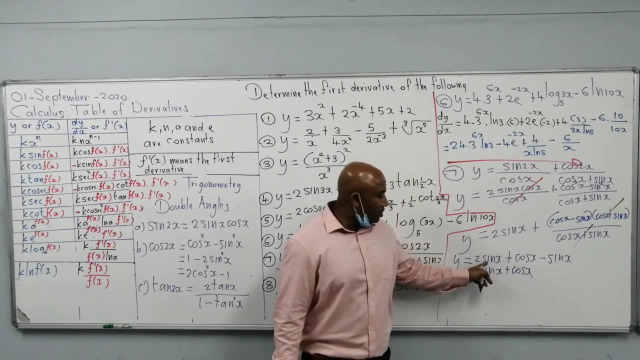 sin x, So y is just equal to sin x plus cos x, Because I've got 2 sin x plus cos x, So I've got 2 like terms. yeah, Can you see that 2 sin x minus sin x will give me just. 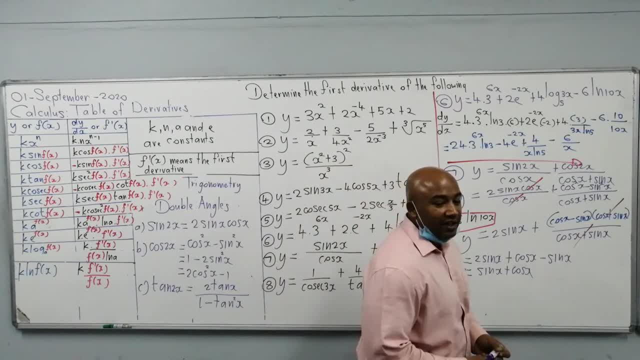 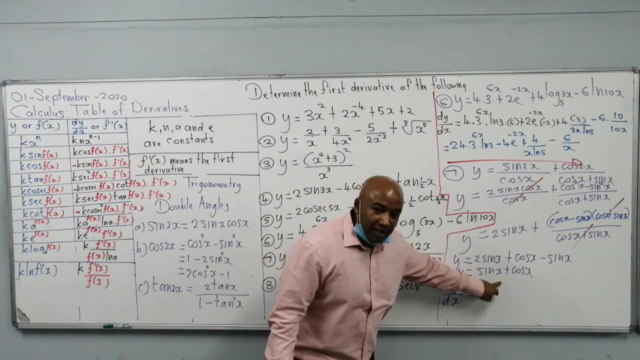 sin x. So that is all. Now I can find my first derivative here. So that's going to be dy over dx. Go to your table of derivatives. So it's k sin f of x. It is 1 sin 1x The. 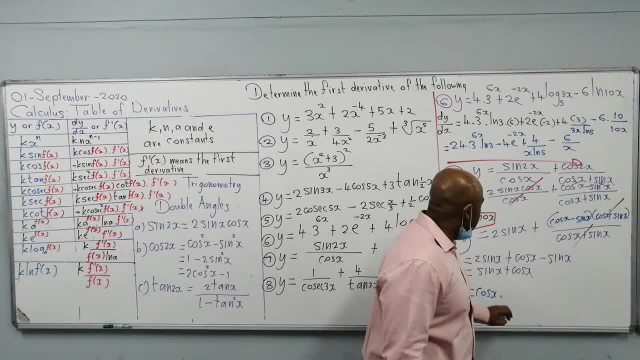 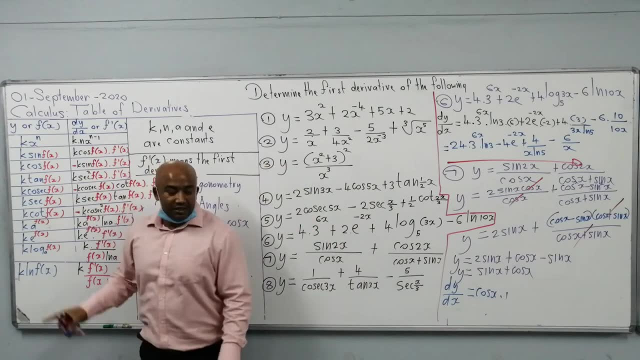 derivative of sin x is going to be cos x times the derivative of x, So that is going to be x here, which is 1.. Remember, f of x, f prime x. You don't have to write down the 1,, but the fact is you need to know that it's supposed to be a 1.. 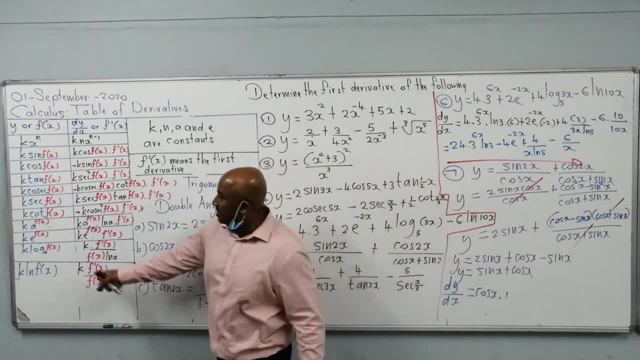 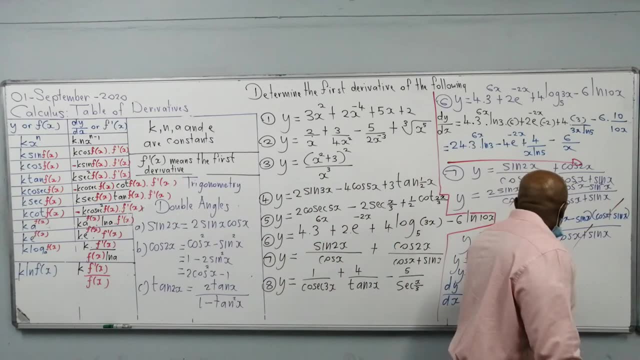 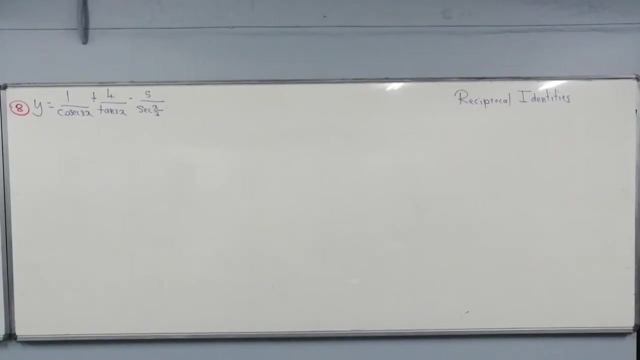 Then the derivative of cos. what is the derivative of cos? Here's your cos. It's going to be negative sin, So that's going to be minus sin x. Nothing to simplify then. So that is the solution. move on to the next one, right? our next example, here again dealing with trig functions, but 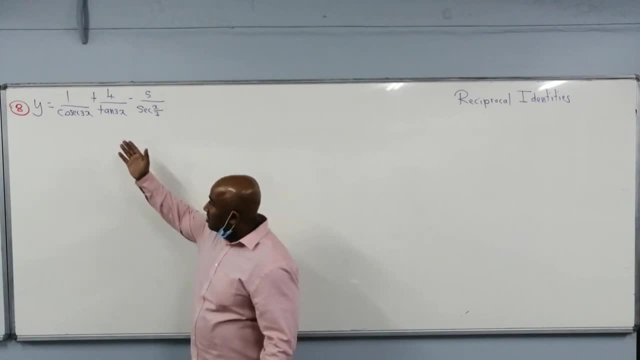 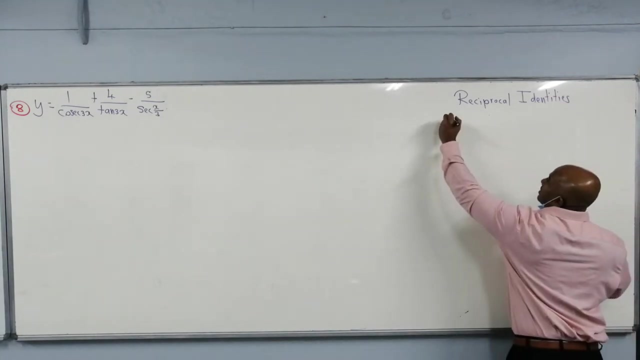 not in standard form. so this is not cosec, it's one divide by cosec. so you don't see the formula for one divide by cosec. you see a formula for cosec. so we go back to our identities. now we need to know that if you have sine x, sine x can be written as one over cosec x or cosec x can. 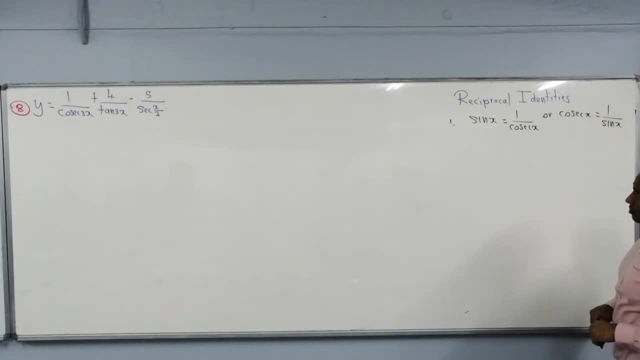 be written as one over sine. what else? if you have cos of x, it can be written as one over sec x, and then sec x can also be written as one over cos. what else? we can have tan x, which can be written as one over cot x. so therefore cot x can be written as one over tan also. 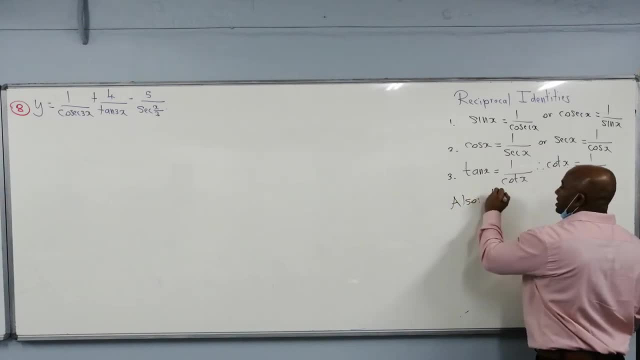 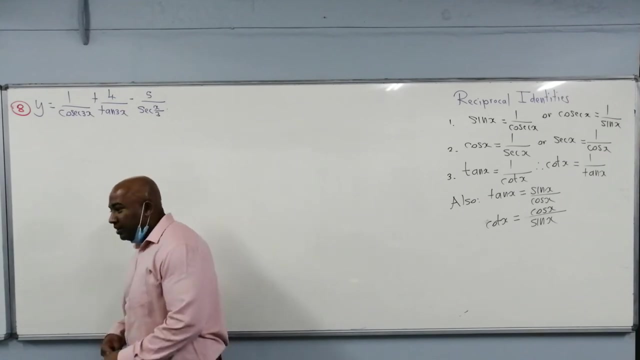 you know that tan x can be written as sine x over cosec x and cortex can be written as cosec x divided by sine x. so those are your reciprocal identities, which are not given to you on the n4 formulations. okay, so if you do not know, you might know the table of derivatives, but you don't know. 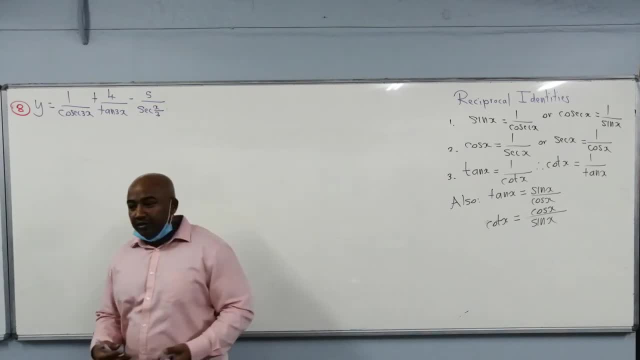 this, you're gonna have a problem. so we the new view. as a result, all this into standard form: one over cosec is going to be sine of 3x, then four over ten will be one of the tens cot. so that's going to be Bitchon, so times. 5 divided by sec, it's the same as five. cost of one over 3x. okay, because one over 3x and 5 divided by sec is the same as five. cos qo Pelham Nassim Seller has J Bal Hayır. conquests by verse: nolik. 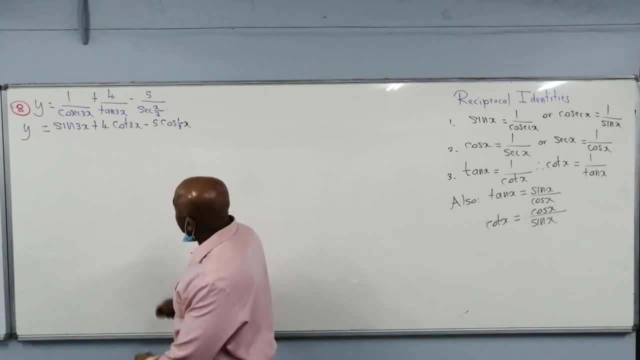 Let's say: this cos is right here in front of you. You can see that. So once it's in standard form, now we can differentiate. So therefore, dy over dx, the derivative of sin 3x. now the derivative of sin 3x is cos 3x. 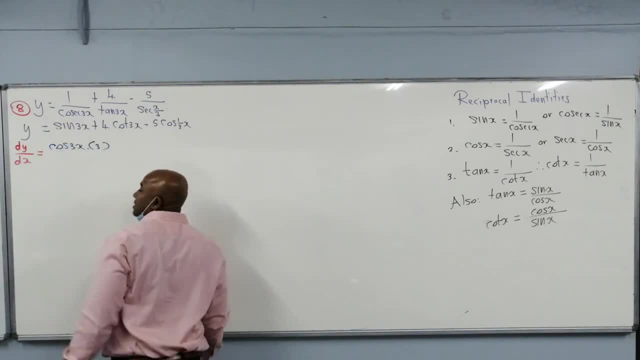 And sin f of x, cos f of x times the derivative of 3x, which is 3.. Here we've got cot. The derivative of cot is negative cosec squared of 3x times the derivative of 3x there, which is 3.. 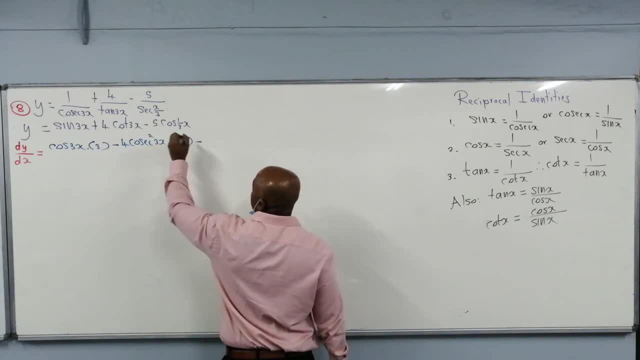 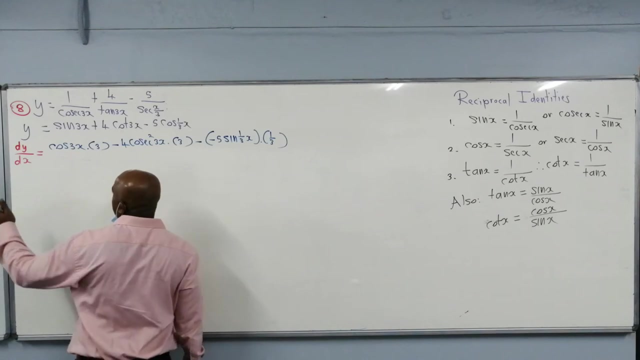 And here you've got cos. Check your table. The derivative of cos is going to be negative: sin 1 over 3x times 1 over 3.. So once you get the hang of it, and it's not difficult, but the main thing is you must know the formula. to make it simple, 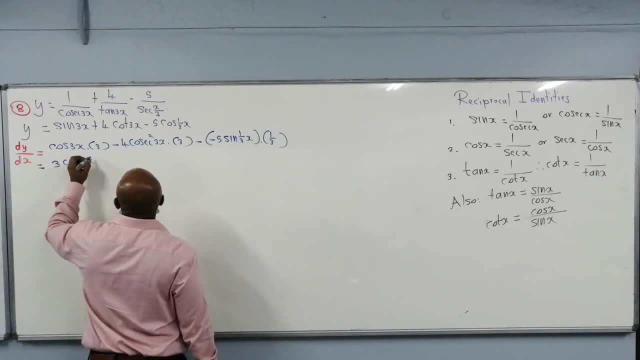 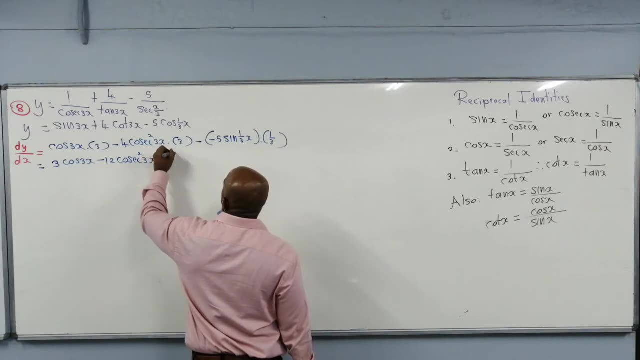 So this is going to equal to 3 cos 3x minus 12 cosec squared 3x. And here this is going to be plus 5 over 3, sin 1 over 3x. There's nothing more to do. 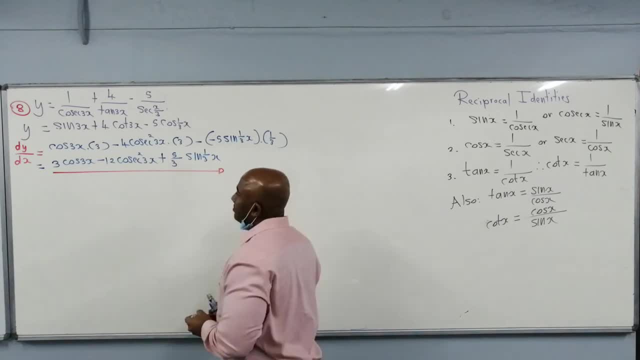 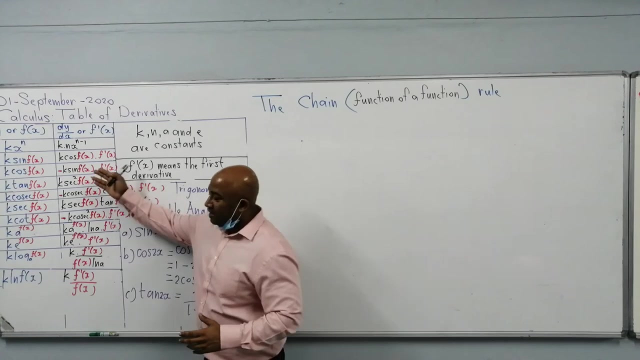 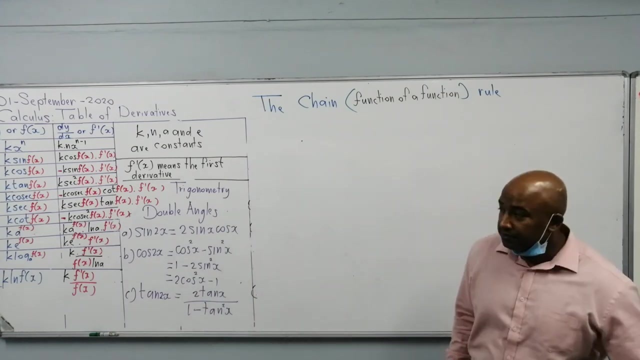 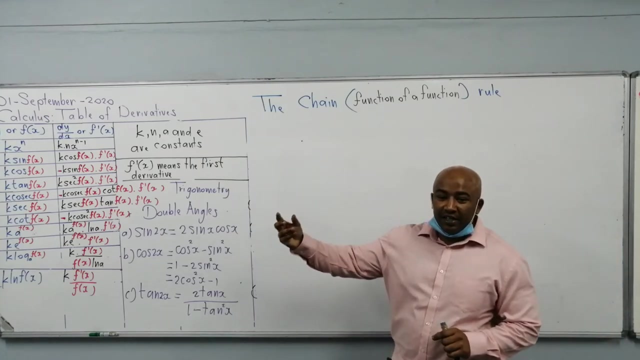 So this is our final answer. All right, so now we're going to deal with the next few rules. All right, so we have been dealing with the table, standard table of derivatives, Now the chain rule. The chain rule deals with, basically, when you have a function of a function. 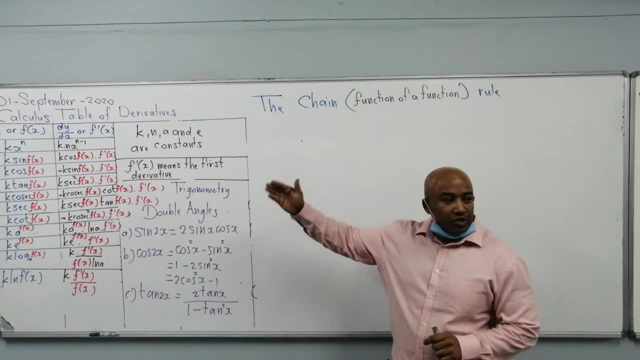 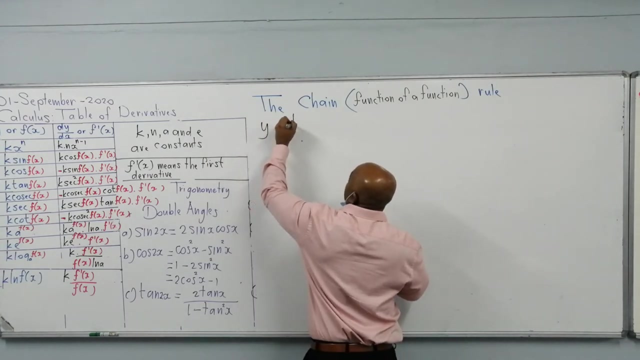 So the chain rule can be applied. It can be applied to any one of these formulas here, And then also when dealing with exponents. Now let's start with something like this first. So let's take, y is equal to k sin f of x. 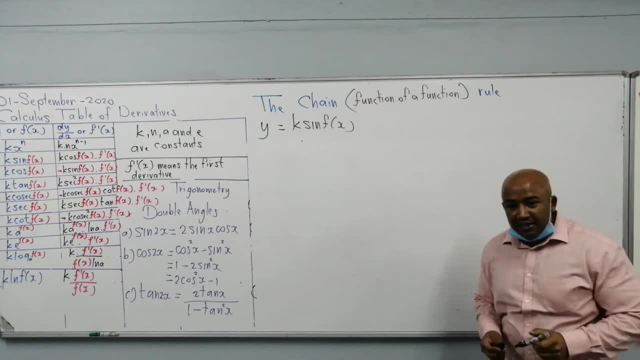 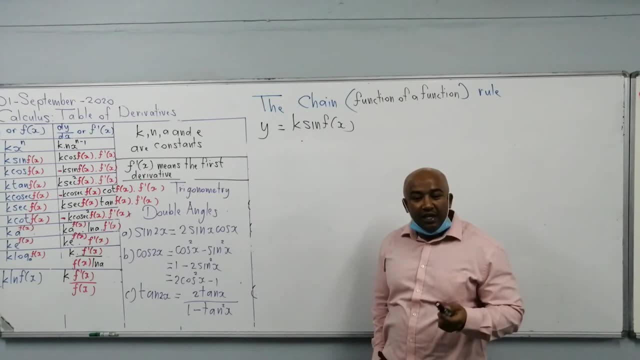 Okay, we know that from the standard derivative. there I taught you that the derivative of sin f of x is going to be cos f of x times. Now let me show you how it's actually worked out. So this is how it works. 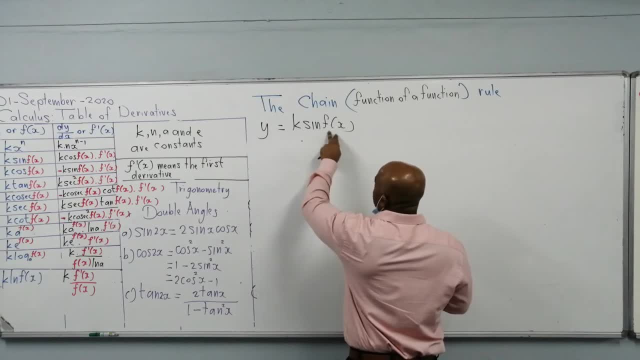 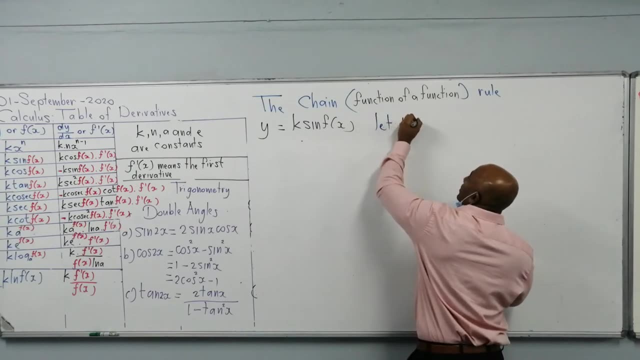 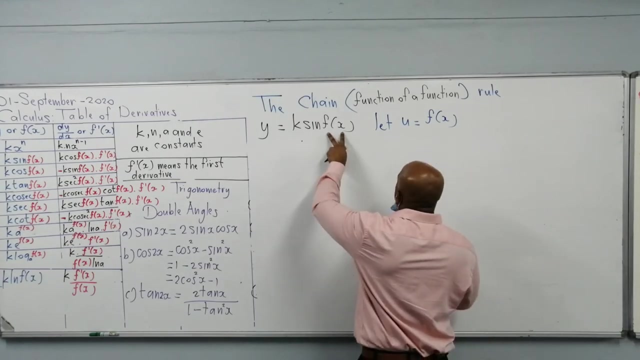 So I can use a substitution here. What I can do is I can replace. I can say: let u equal to f of x. Okay, so I'm going to replace f of x with the letter u. So I'm going to go there, for y is going to equal to k. 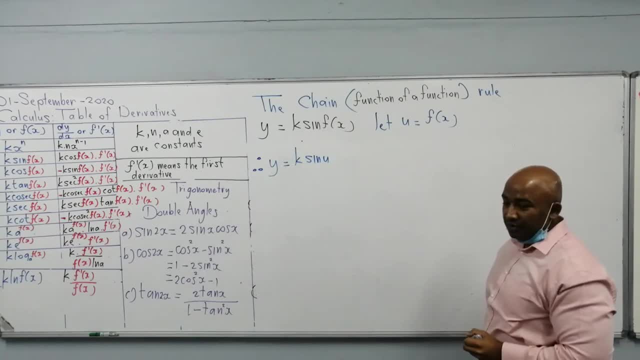 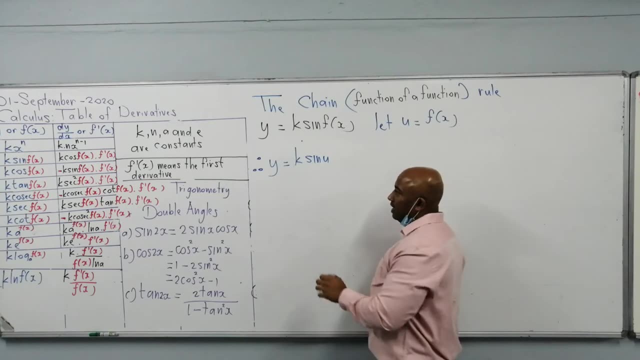 So I'm going to go there, for y is going to equal to k sin u. Right, because I'm replacing f of x with u. Now, here I have y with respect to u. So if I differentiate y with respect to u, dy over du. 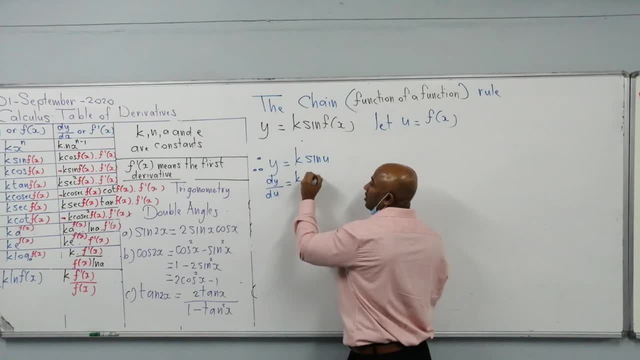 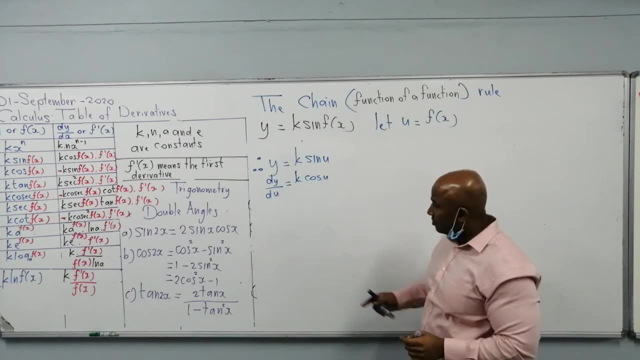 the derivative of k sin u is going to be k cos of u. It's just that it's not x, now it's u. So here I've got u with respect to x. So if I go du over dx, the derivative of f of x is written as f prime x. 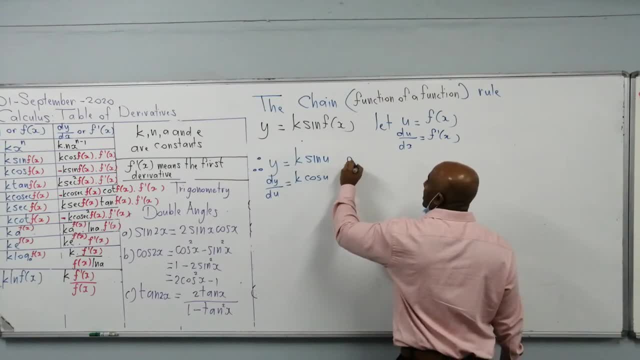 Okay, now the chain rule formula. I want to find dy over dx. That was the question. So I wanted to find dy over dx. Okay, that was what it was originally. I'm going to have y in terms of x here. 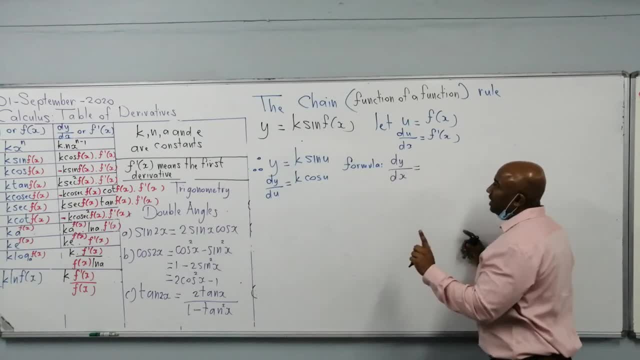 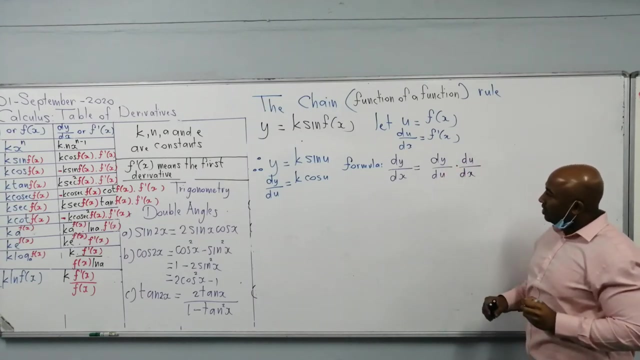 Can you see that? So dy over dx. How can I use this information that I just worked on? How can I use that and that? So all I have to do is take dy over du and multiply it by du over dx. Notice du and du. cancel on the left-hand side. 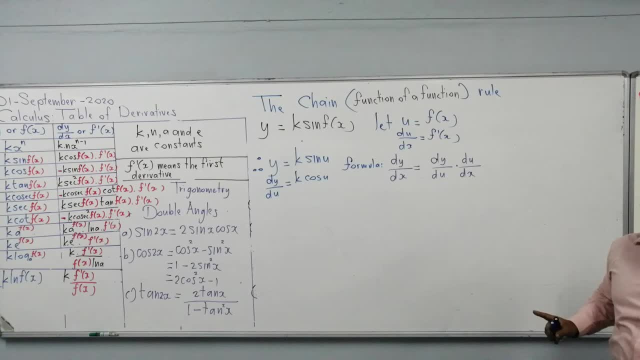 I've got dy over dx on the right-hand side, Also dy over dx. Can you all see that? So now this is the chain rule for dealing with something like this. So what is my dy over du? My dy over du was k cos u. 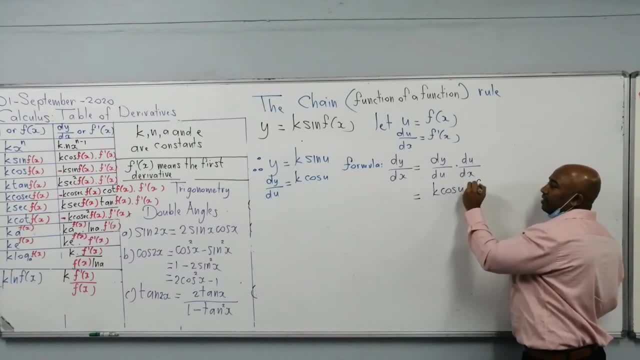 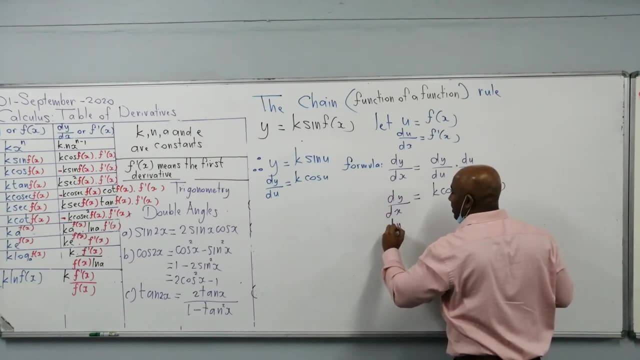 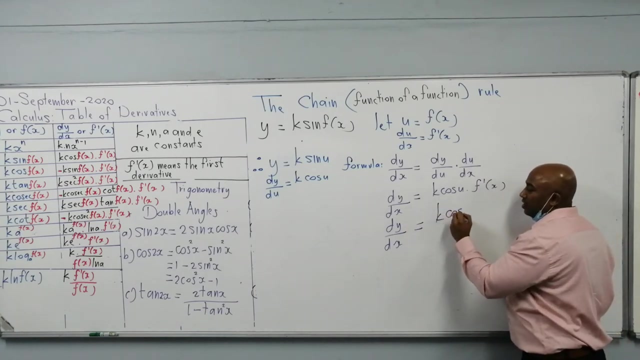 What is my times du over dx? What is my du over dx? f prime x. So therefore, my dy over dx. I can now substitute that for u. So that's going to be k cos. So that's going to be k cos of u times f prime x. 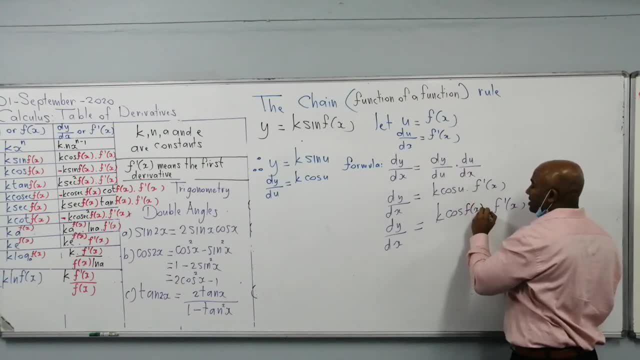 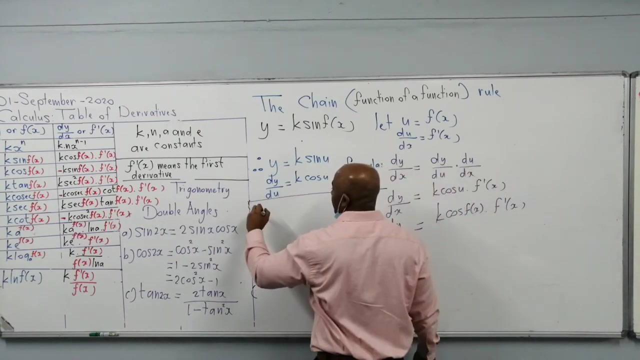 And what was u, What was u? u was f of x. So this is how you actually work it out: by using the chain rule. You could be asked to use the chain rule to differentiate, something like: let's take this one here. 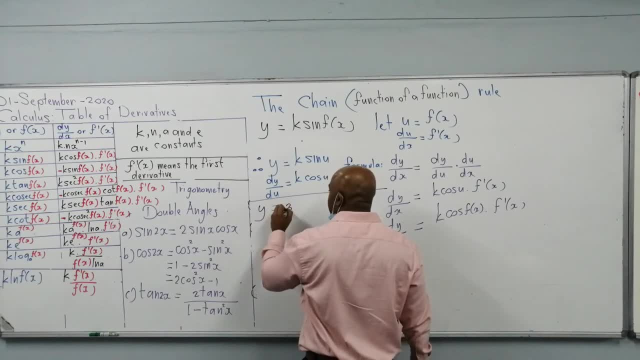 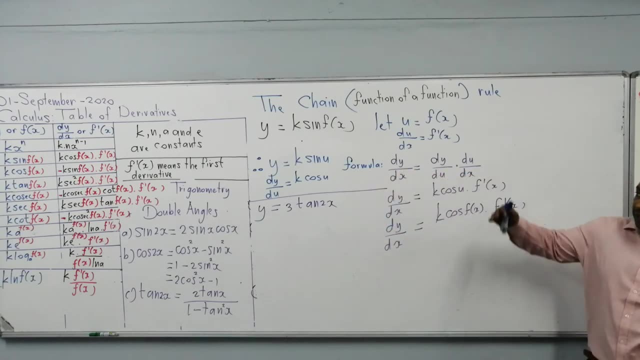 Let's go for. y is equal to 310.. 2x. So if we're going straight from the table, if it applies for sine, it will apply for cos tan, anything from the table on derivative. So if you are given 3 marks or 4 marks and the question states: use the chain rule, then 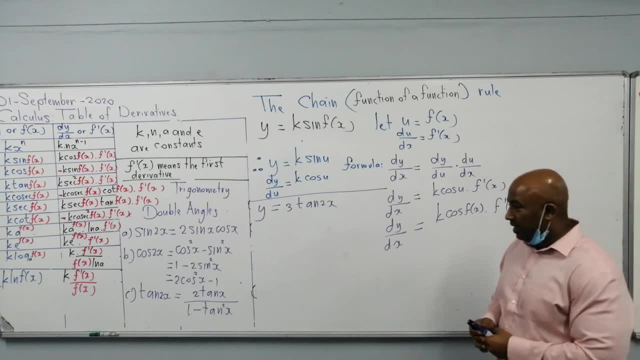 you need to show working. So now what I can do here is I can always my f of x part. I will leave it equal to u. So here I can state: f of x is equal to u. So here I can state: f of x is equal to u. 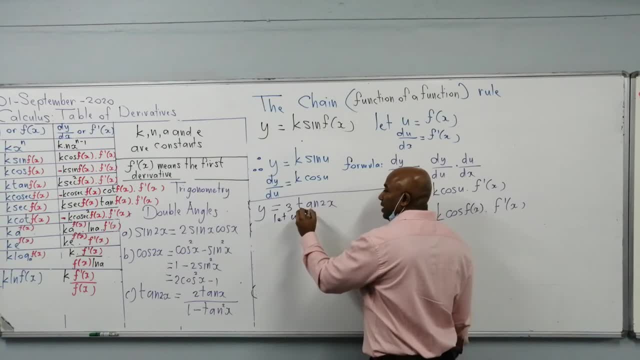 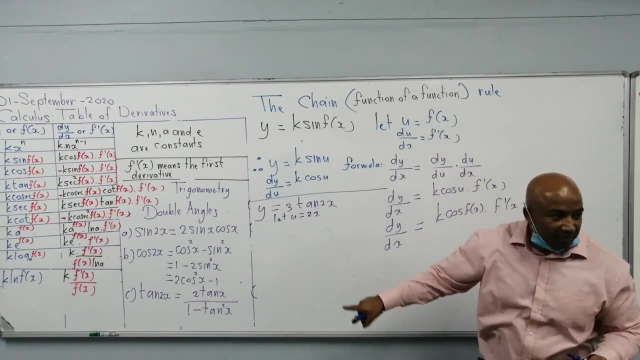 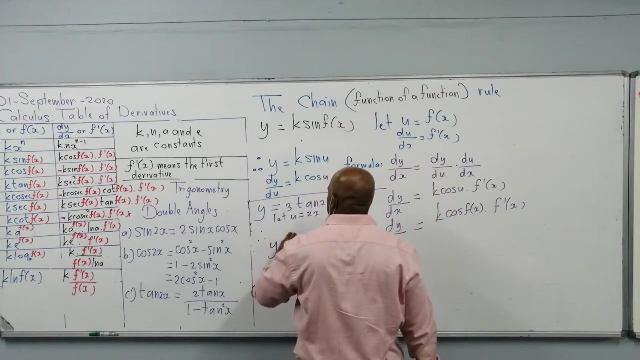 So here I can say: let u equal to 2x, which is f of x. I always let u equal to f of x from any formula here. So therefore y is equal to 3 tan u. Can you see that? 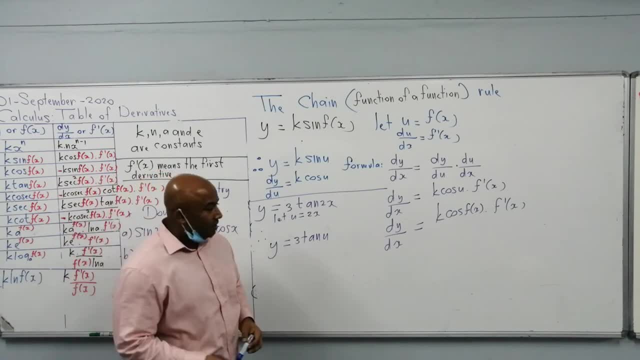 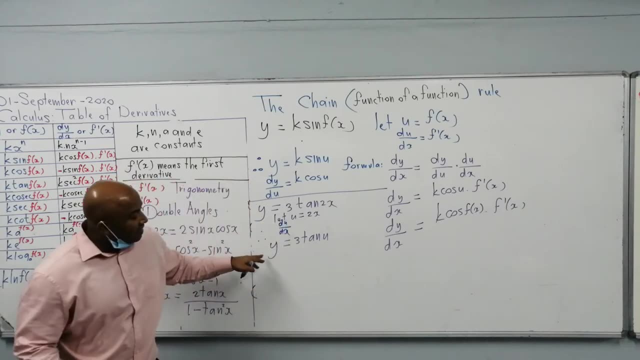 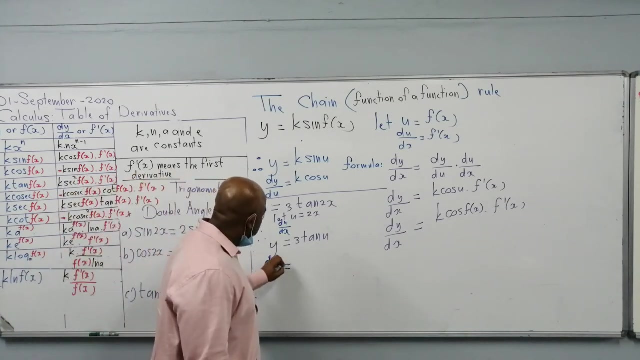 I'm replacing 2x with u. Now, here I will find du over dx. That's right. So I'm replacing du over dx. So now I can say I'm replacing u over dx, And here I'll find dy over du, because it's y with respect to u. I'm going to go dy du. So here, what is the derivative of 2x? It's just 2.. What is the derivative of 10?? The derivative of 10 is going to be sec squared. 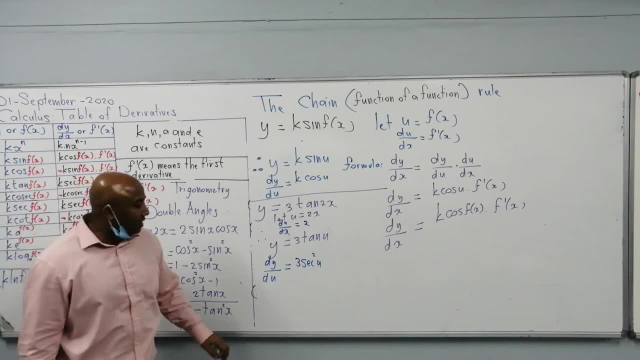 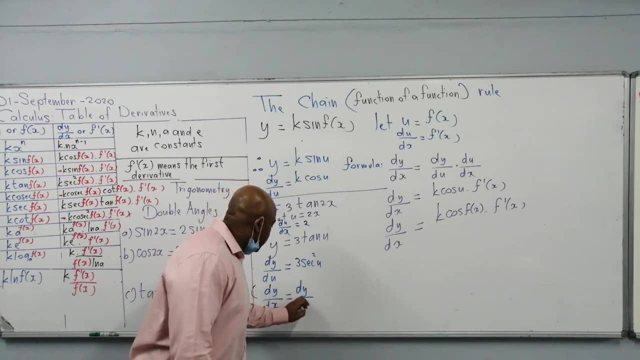 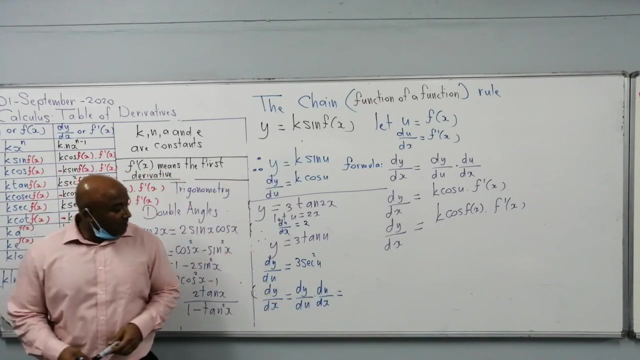 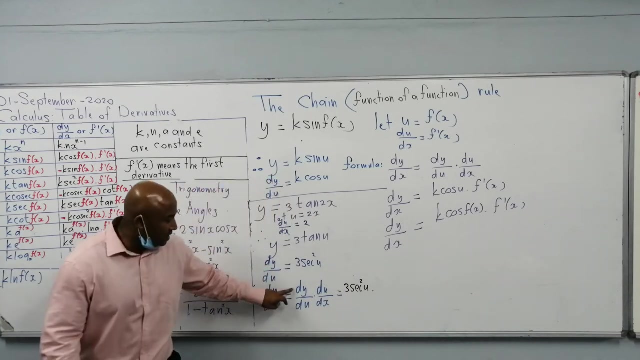 Okay, Now all you do is write down the formula: dy over dx is equal to dy over du times du over dx, And then I do my substitution. What is my dy over du? It was 3 sec squared of u. Here's my dy over du. Here's dy over du. You can see that. 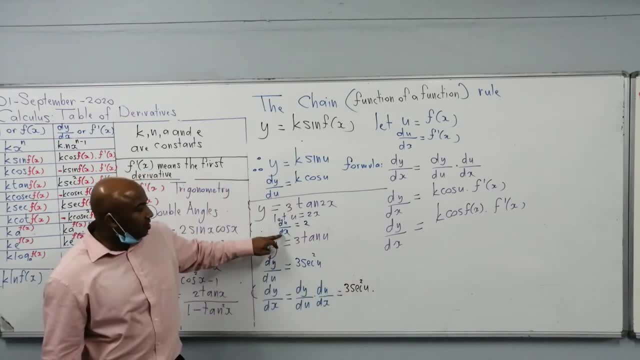 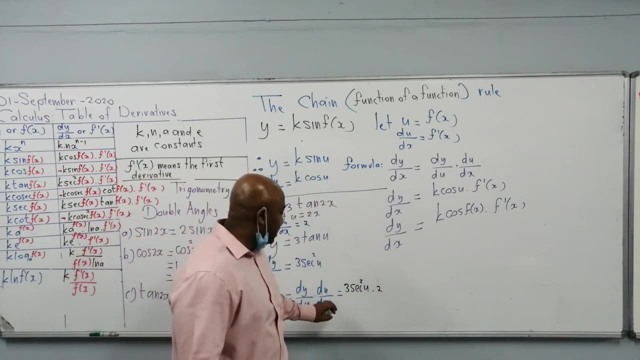 Times du. My du over dx, My du over dx is 2.. Okay, So now I'm done. now, 3 times 2, that's going to be 6.. Sec squared u And what is u? u was 2x. 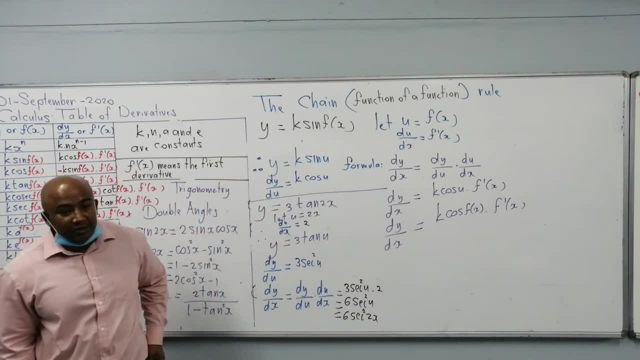 So if you are asked to use the chain rule for something that's so simple, you will have to do it this way. Now it will apply for anything on the table here. You always let u equal to f of x, Alright, So now let's deal with exponents. Let's deal with the exponents. 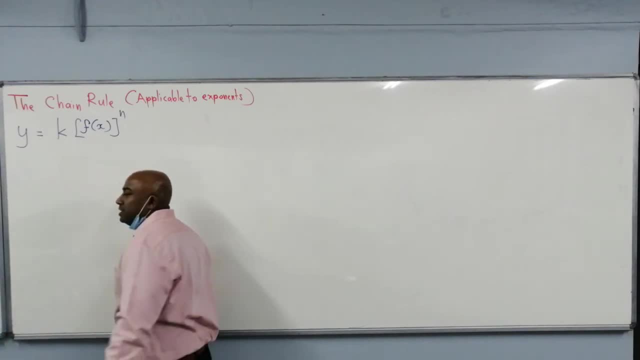 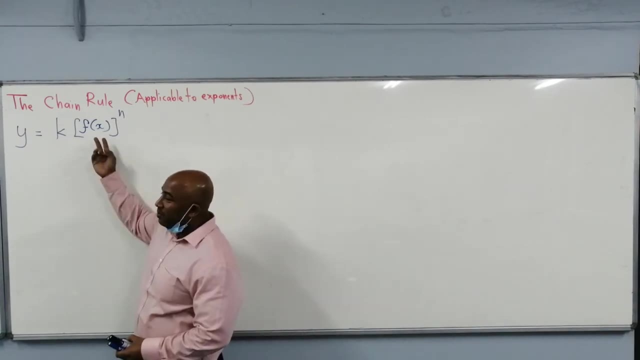 Alright, So now what happens when we have exponents? You haven't dealt with that. Okay, So now what happens when we have exponents? You haven't dealt with that. your function of x, so this can be anything from your table of derivatives, right? so? 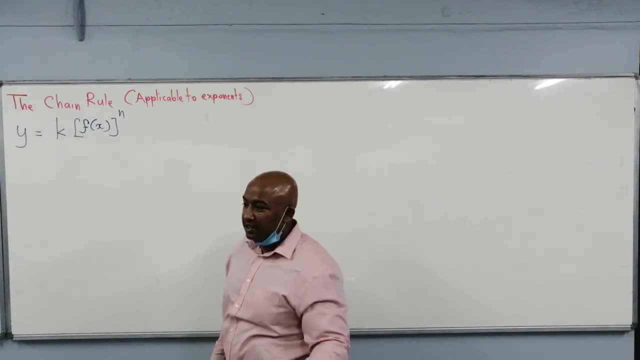 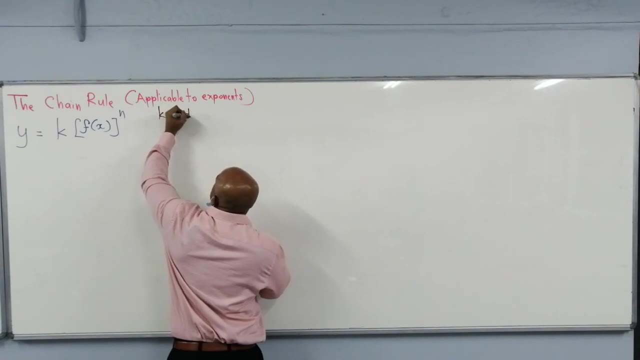 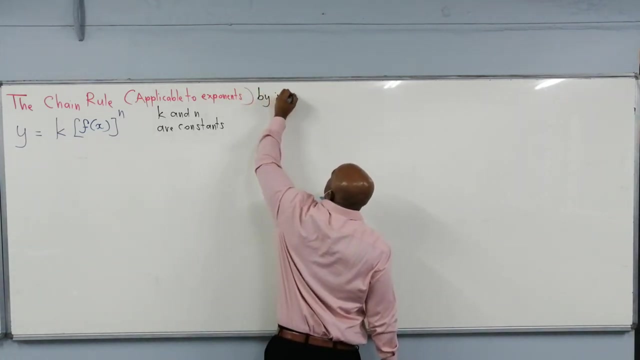 this here could be x, it could be sine x, could be cos x. how do you deal with something? for now, you know your k and n are constants. so now this is the chain rule by inspection, two methods when we're dealing with exponents, right? so if i want to differentiate this here, 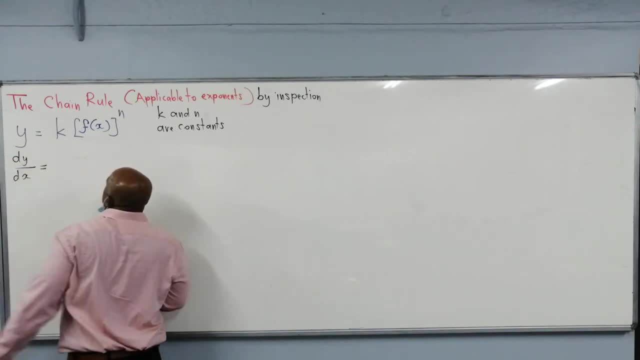 i'm going to go dy over dx. so now, this is similar to the first formula. when you have an exponent, what do you do? you take your constant for your coefficients multiplied by the power, so that's k times n. can you say that? then you've got your f of. 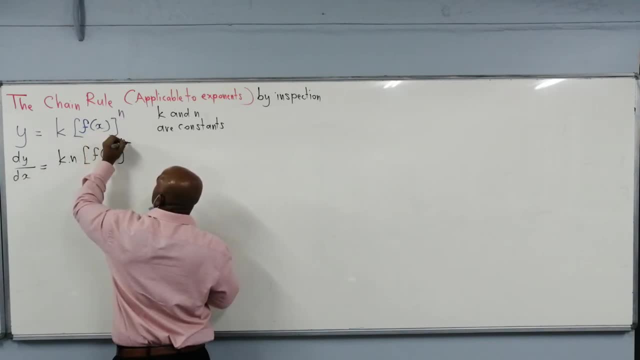 x, whatever's inside. here you take the power and you subtract one, but now remember, there's an f of x. so whenever there's an f of x, i need to times and differentiate this. and i got my answer outside. so you're dealing with a function of a function here. 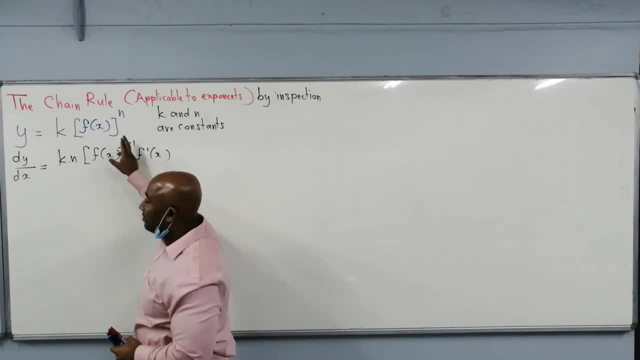 so you're dealing with the exponent. it's like you're differentiating the exponent first, then you're differentiating what's on the inside. so you start on the outside and then you move inside. so this is by inspection. let's take an example. let's say y is equal to 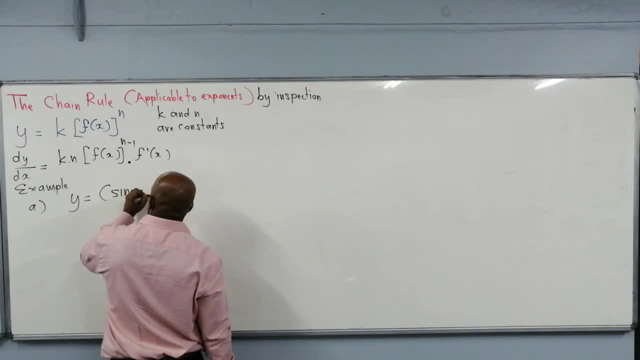 um sine 2x plus one. okay, this goes for sine 2x plus x squared, all raised to the power four, right? so if i want to differentiate this now, this obviously the great draft you won't be able to deal with, right, but because of the trig function, yeah, but the power four. that means they are formal. 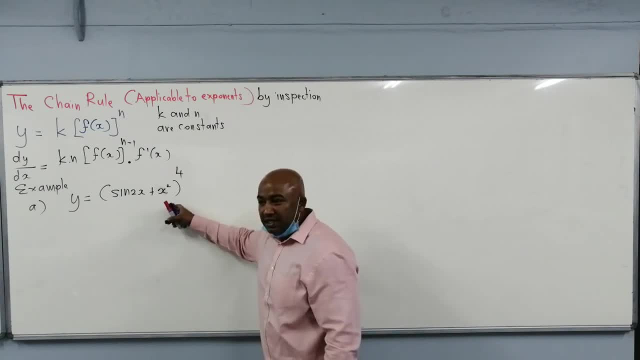 parts of this here. so you're not going to go and write this sine 2x plus x squared, sine 2x plus x squared four times. you're not going to multiply, it's going to take too long. so therefore we use the chain rule to differentiate. so i check now my number. let's add a number in front. let's put it as: 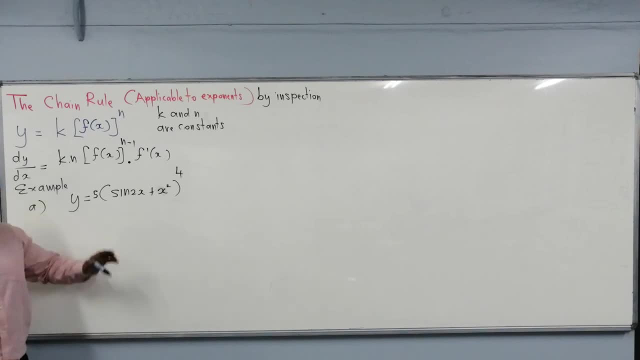 five, any number in front. so now my k is five, my n here is four. my function of x is something from the table of derivatives. it's sine 2x plus x squared. Can you see that? Now I need to differentiate, So I'm going. 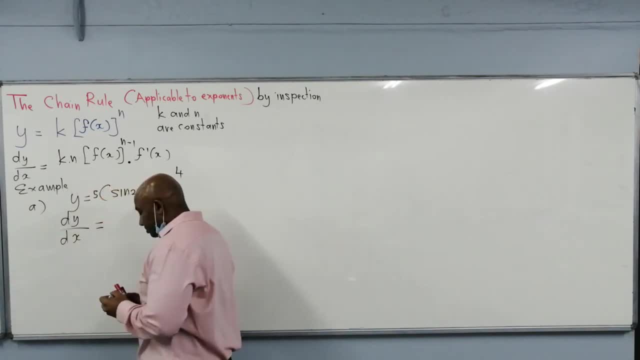 to go dy over dx. So now, how do we do this? We're going to go. there's your k, there's your. we do the exponent first. So it's going to be 5 times 4.. And you've got sine 2x plus. 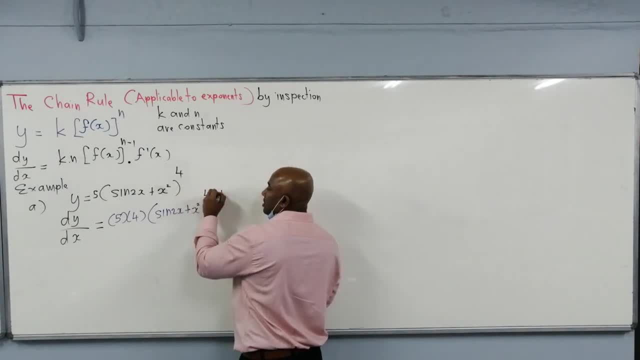 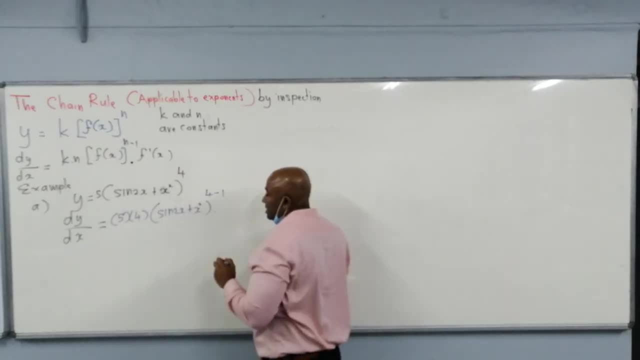 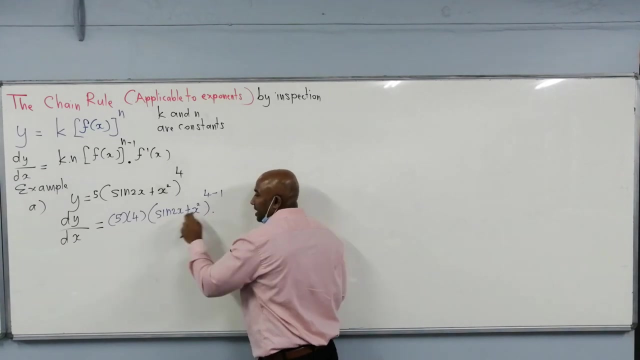 x squared there And now here, 4 minus 1.. Can you see that You deal with the exponent first. So I'm at this stage, here, now Times. now remember your f of x, this is your f of x. So what you need to do is now differentiate this and write down the answer outside. So, 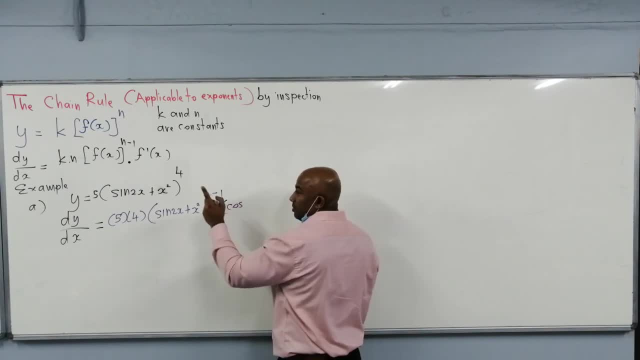 the derivative of sine 2x is going to be. you go to your table of derivatives now. Derivative of sine of f of x is cos of f of x. cos of 2x Times f prime x, the derivative of 2x is 2.. Plus plus, don't forget, we've got term. 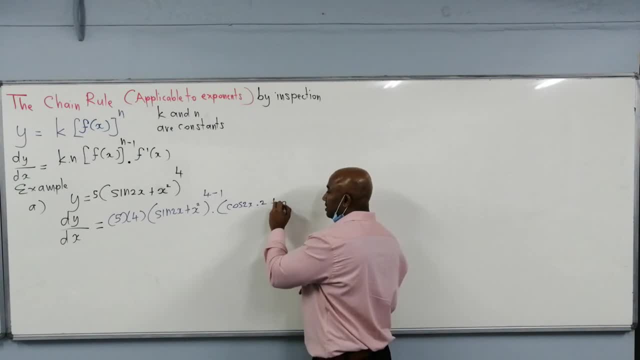 2. The derivative of x squared is going to be 2x, And that is a chain rule. It's not difficult. Remember exponent first and then everything on the inside. This is by inspection. Let's simplify here: 5 times 4, that is 20.. And then I've got sine. 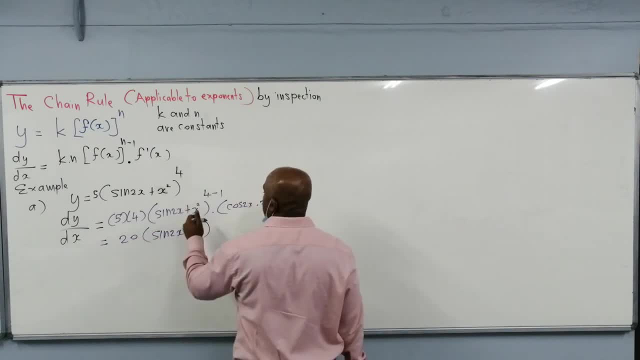 2x plus x, squared 4 minus 1, here is 3.. And this is 2.. Cos 2x plus 2x, Let's take another one. We've only got a few minutes left here. Let's take another one. So if I. 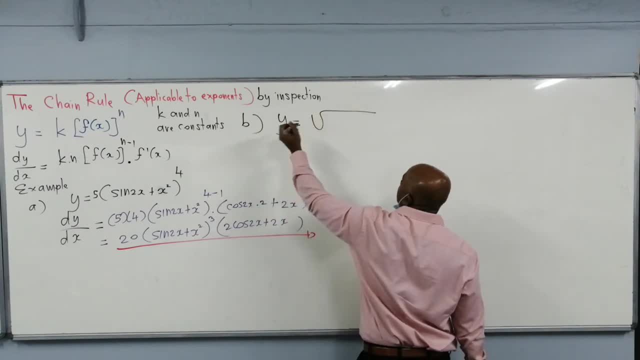 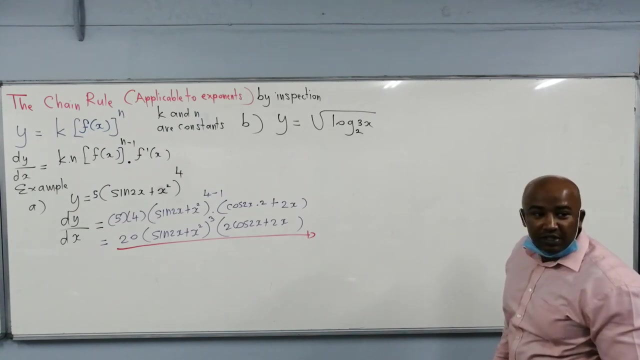 got y is equal to the square root of. Let me go for Log of 3x to the base 2 here. If I got y is equal to the square root of log 3x to the base 2, first thing I want to do is change this, that square root, rewrite it as an exponent. 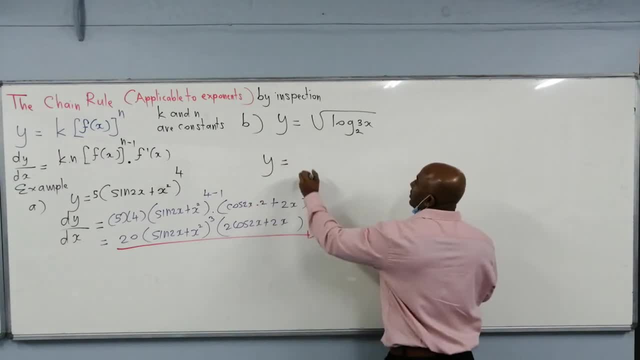 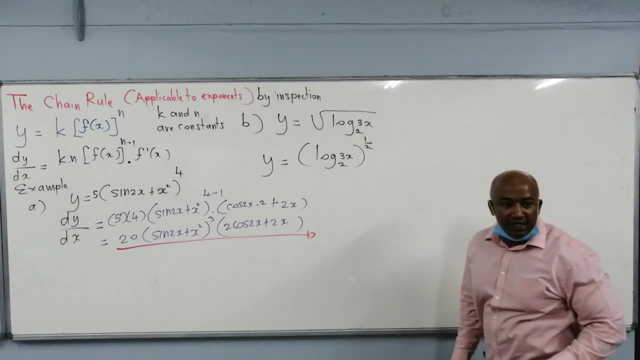 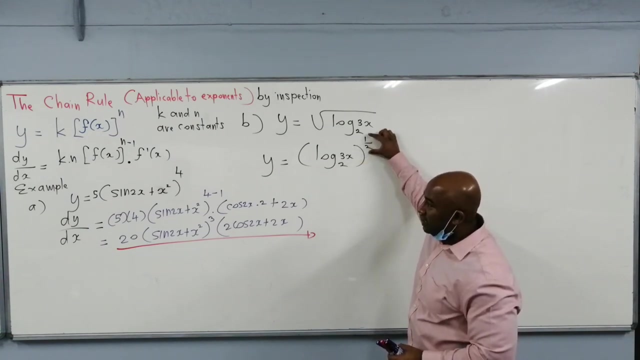 So now I've got y is equal to. I can write this as Log 3x to the base 2, all raised to the exponent r. Can you all see that? So now my f of x, my function of x from the table of derivatives, is Log 3x to the base 2.. My exponent here: 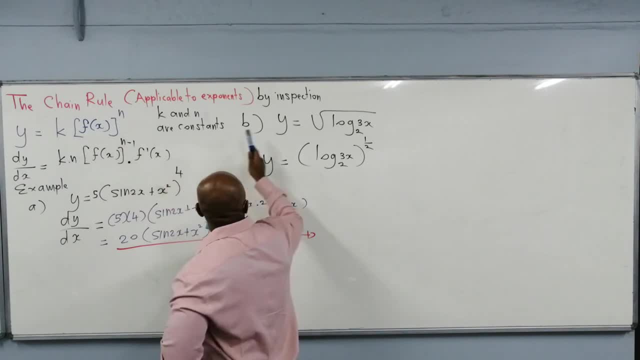 is Half. So there's the share: 10 is equal to half. And then f of x. here is everything inside the bracket. So now I'm going to go dy over dx. So I have an exponent. I must deal with the exponent. 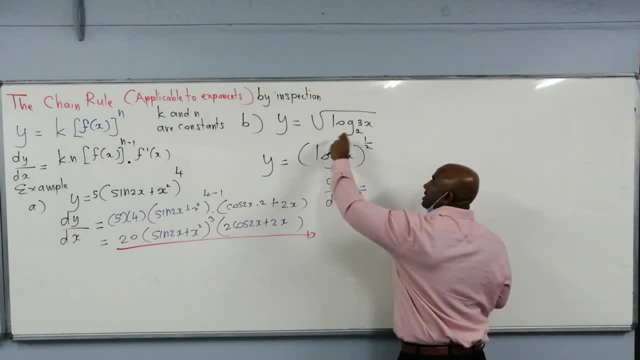 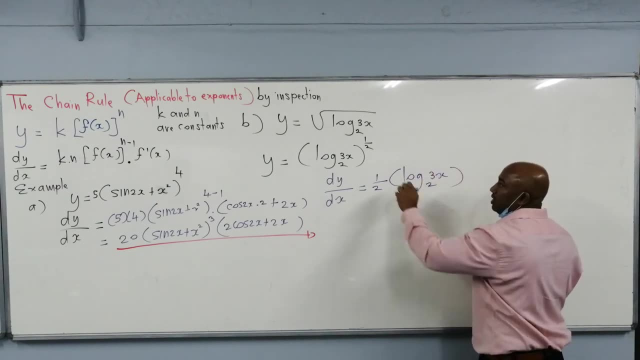 first, all the time Change. So that's 1 times half, which is Half, And then I got log of 3x to the base 2. And then here I'm going to go, half minus 1.. Can you all see that? 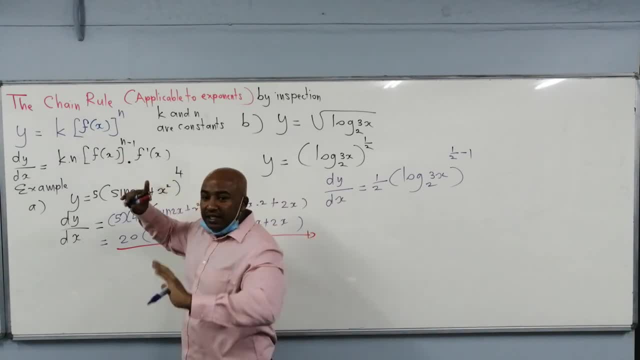 So where am I at the moment? I'm at this stage. here I deal with the exponent first. I do not insert, I just copy down f of x as it is. Now I'm going to differentiate f of x and now I'm going to load times and I need to. 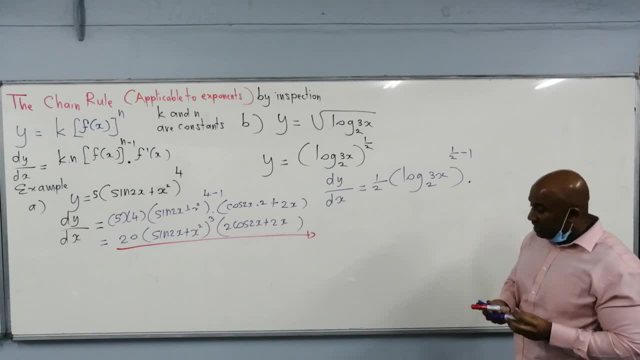 differentiate log 3x to the base 2.. How do I differentiate log 3x to the base 2?? Remember, if y is equal to k log f of x to the base a, then y prime, the derivative is going to be k, f prime x, all divided by f of x times log a. 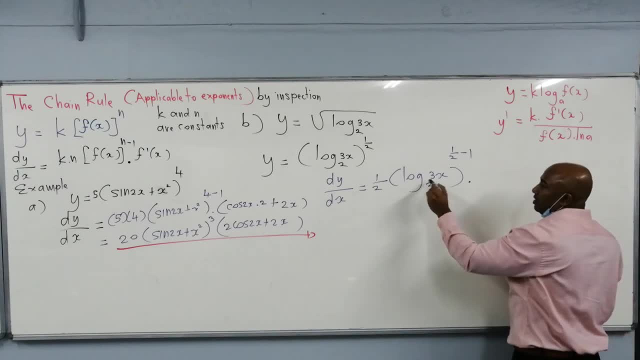 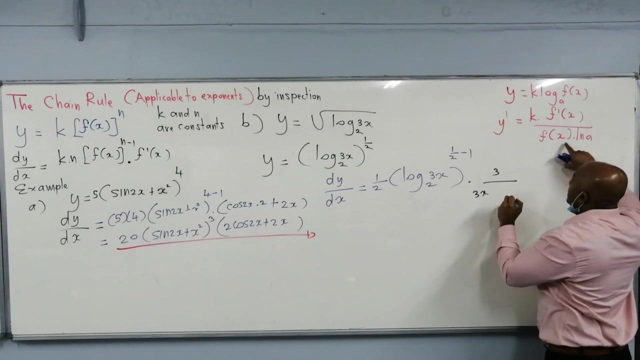 That is the formula for differentiating log. so I've got log 3x to the base 2, the derivative there is going to be: I've got my here's, my division line here. so that's going to be 3 f prime x, all over f of x, which is 3x times length of the base, which is 2.. 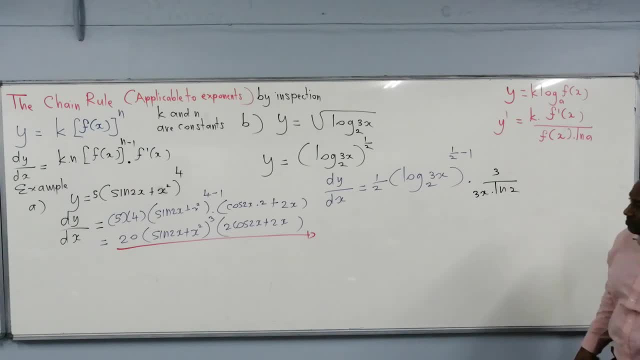 Right, so that is the derivative of log. Let's simplify this here. so that's going to be half. then we've got log 3x to the base 2, half minus 1 is minus half. 3 and 3 cancel here. so I end up with just 1 over x length.